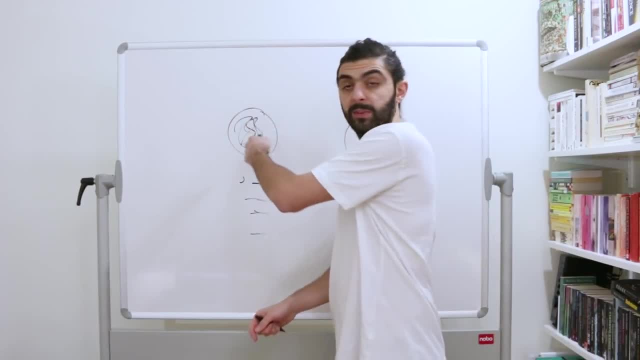 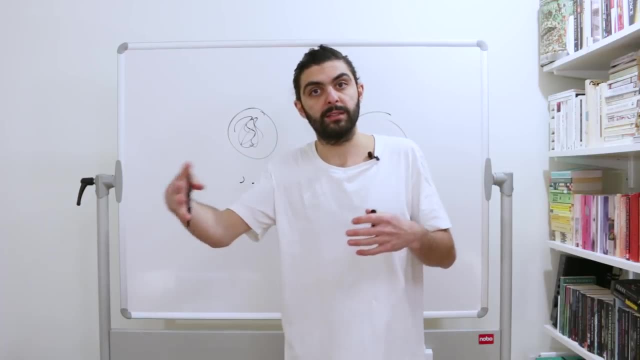 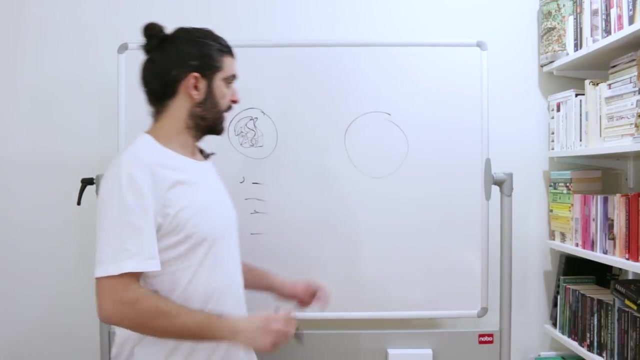 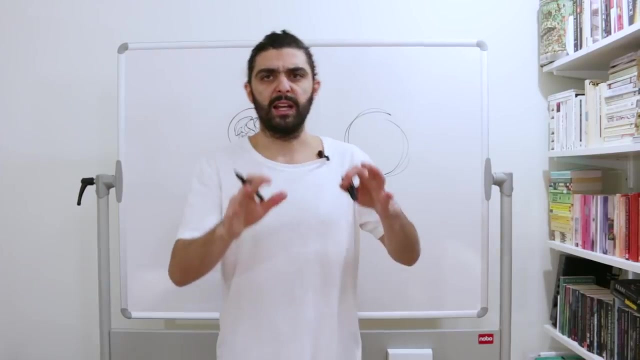 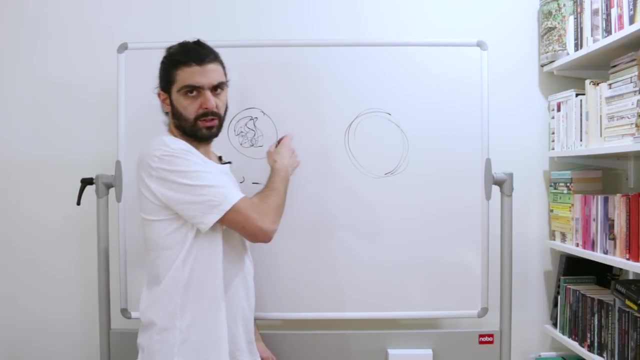 So in headfirst and in the example that we'll go through, we'll talk about something like a weather station, right So, a weather station that measures weather data, and as soon as it does another measurement, the measurements may or may not have changed. So this thing changes state, Doesn't matter what it does, but generally it changes state. And then we have this other thing, and this thing wants to know for some reason about the state that this has. And your alarm clocks may be going off and you say that that sounds like introspection, like feature envy, like maybe this object is super concerned about the internals of this thing. 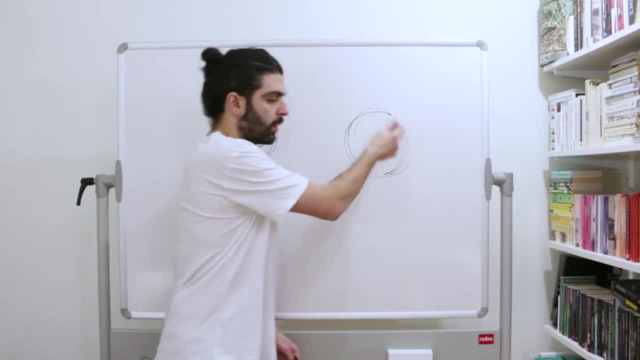 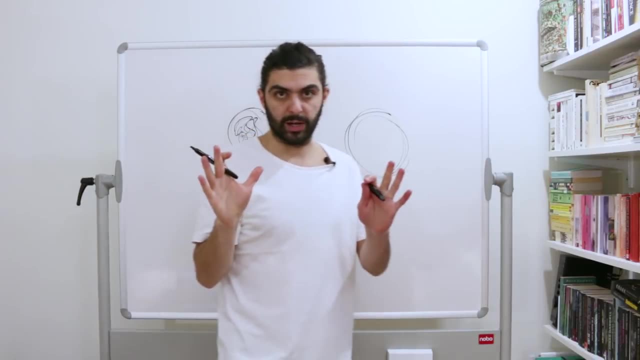 That's not what we're after here. What we're saying is that this object for some reason needs to know whenever this object changes its state. That's not an absurd situation, right? Could totally happen. Think about the weather data example, right. 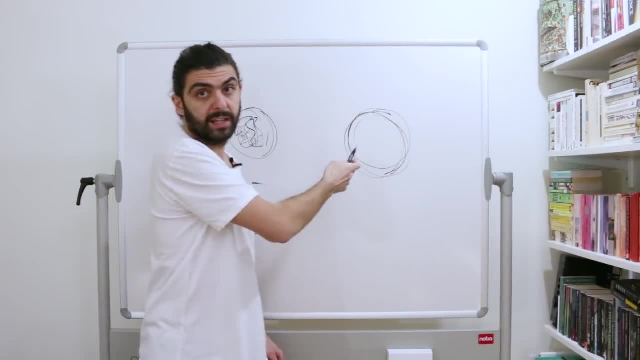 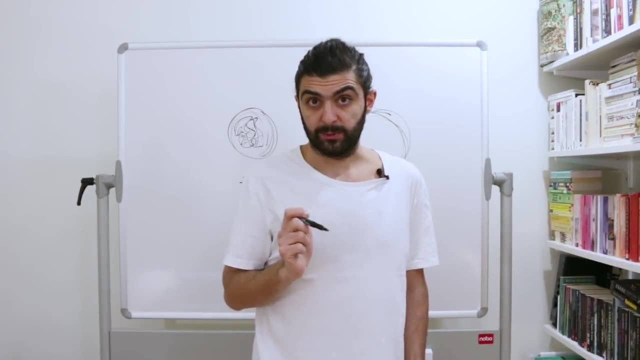 So this is a subscriber, This is some kind of- for example, in this example- display that wants to know when the data here has changed. Think about an RSS feed. This thing is a client, an RSS client, a reader, and it wants to know when the data here has changed. 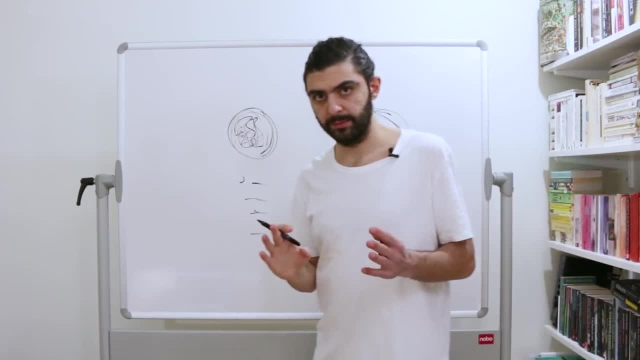 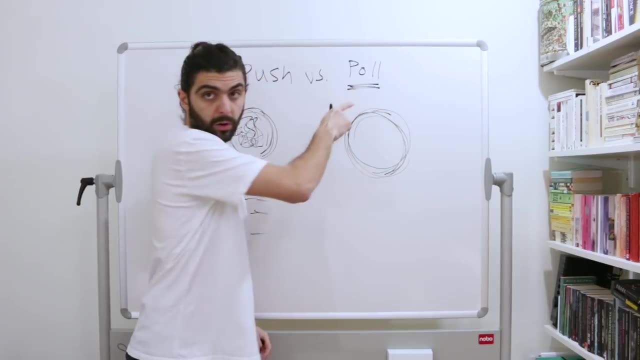 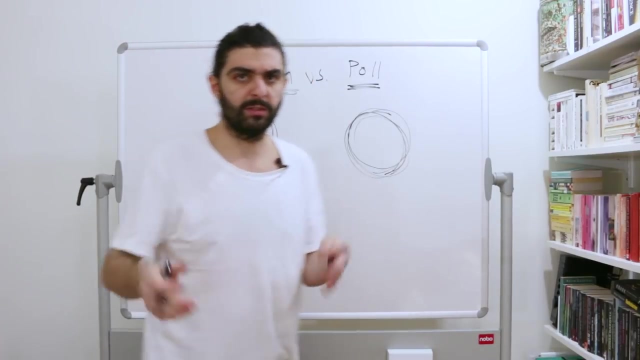 when a new article has been published. So observer pattern is essentially about push versus pull, So it's about moving from a pull architecture to a push architecture. Now, these words are usually more used in terms of networking architectures and web service and et cetera. 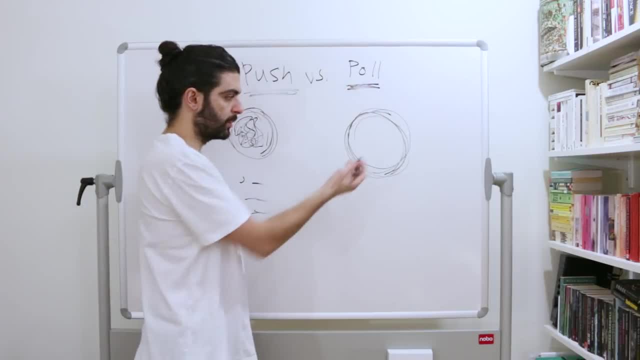 So this is by analogy, but essentially what would pull be. So this is the subscriber right, This is the thing that wants to know about the state of this thing. So what we could do is that we could just say: okay, let me just ask this thing, have you changed? 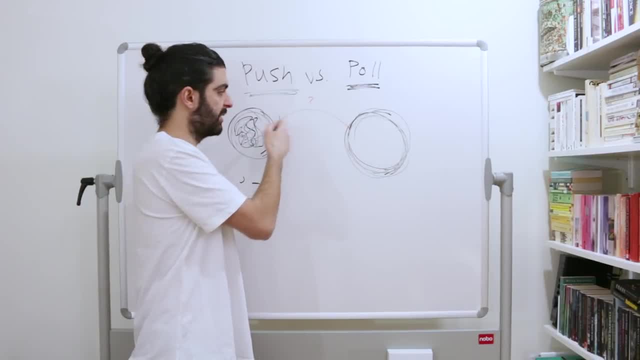 Right, we say okay, hey, object, have you changed your state? Right, give me the data back. And then again: have you changed? And have you changed, And have you changed, And et cetera, et cetera, et cetera. 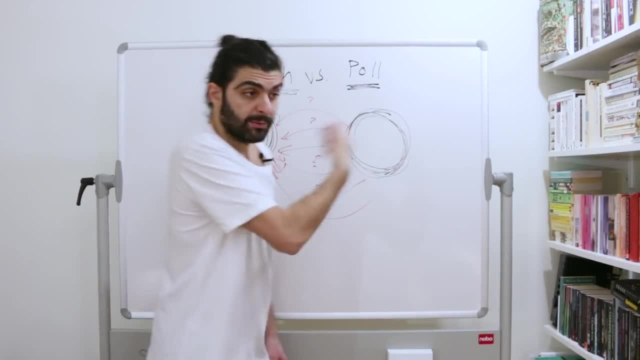 It just keeps on asking, and asking, and asking, And you have to do that indefinitely because you don't know when the state of this thing will change. So you have to keep on asking And then it's a question: okay, will you do this? 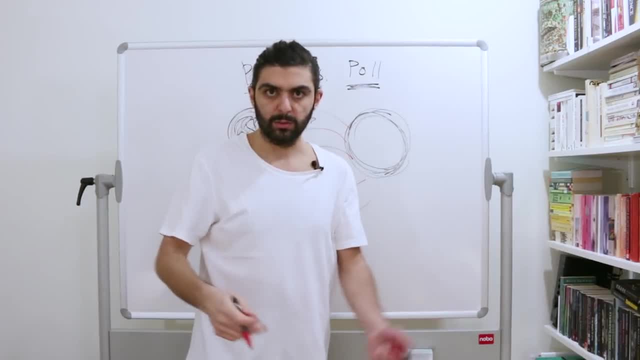 what? every millisecond? Or will you ask every second? Or I mean, if you ask every millisecond, ask every second, what if it changes after half a second? Then your update frequency is not small enough or not quick enough, And then if you scale this up, of course this is absurd. 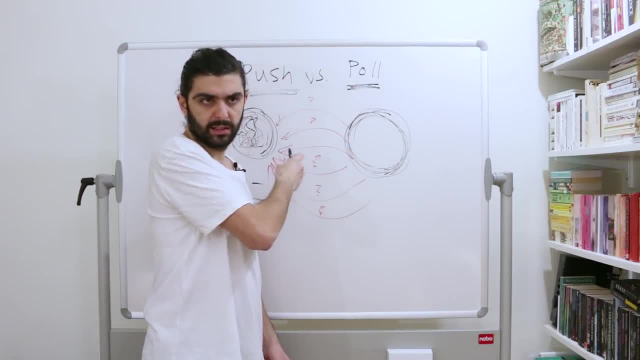 because now we're just talking about one object that's interested in the state of this other thing, But you could of course have tons and tons of tons of objects that all want to be updated whenever the state of this thing changes, And then polling suddenly becomes absurd. 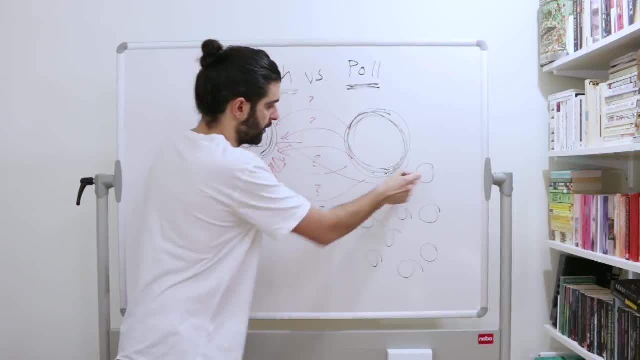 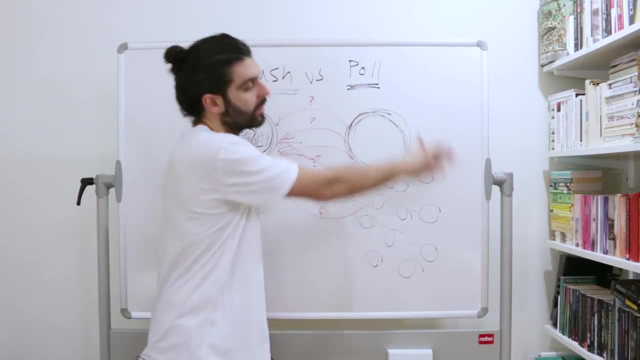 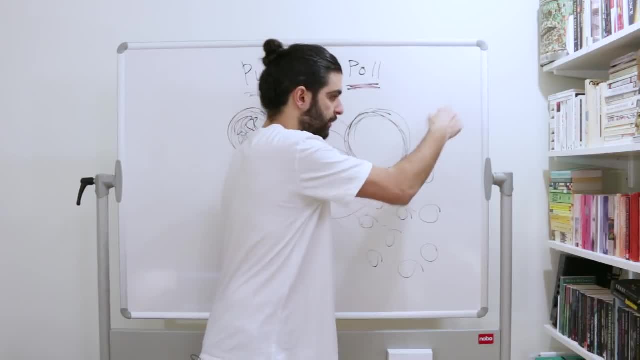 This is polling. We're polling for changes. We're asking: have you changed your state? Or it doesn't even have a question. I mean, when we're saying that, have you changed your state, it sounds like we're asking for a Boolean. 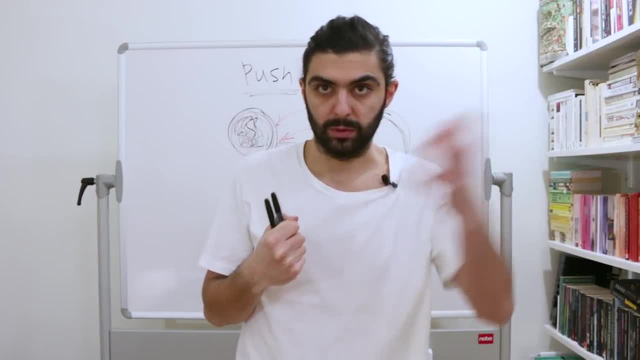 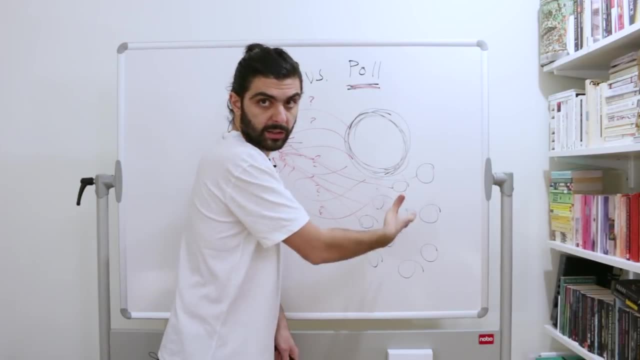 It sounds like we're saying: have you changed? If you get true back then we'll get the values. But it could have just been: we ask for the values, get the values and then update whatever we want to update here. 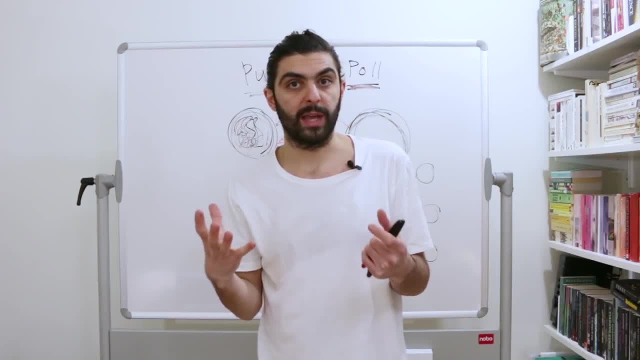 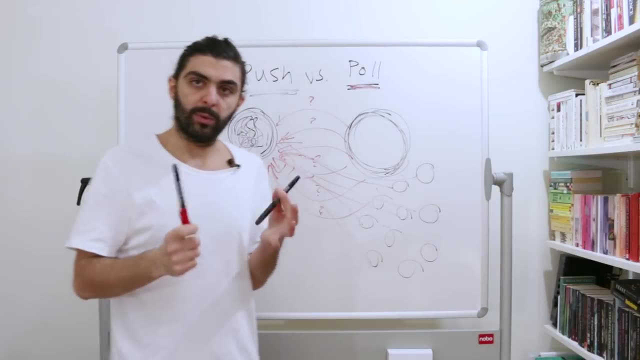 But the point is we're asking for the data before we know that we actually have new data, before we know that this guy actually has new data. So instead of that observer pattern helps us move into pushing, We're saying, okay, all of this red stuff. 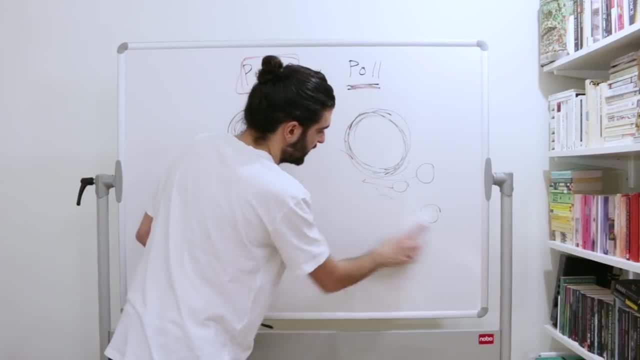 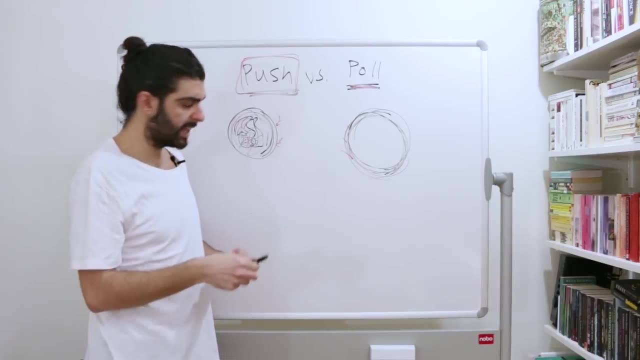 all of these asking arrows. that's a bad idea. Let's go back. let's remove these and just remember that there could be multiple subscribers, but let's just go back to one. So asking is a bad idea. So instead, what we want to do is that this guy 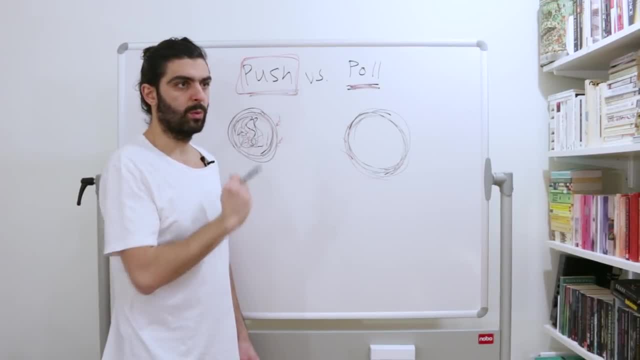 should be responsible for telling all of the subscribers when it has changed. So this undergoes changes for some reason. right? We said you have state one and then after some time you end up in state two, and then you end up in state three. 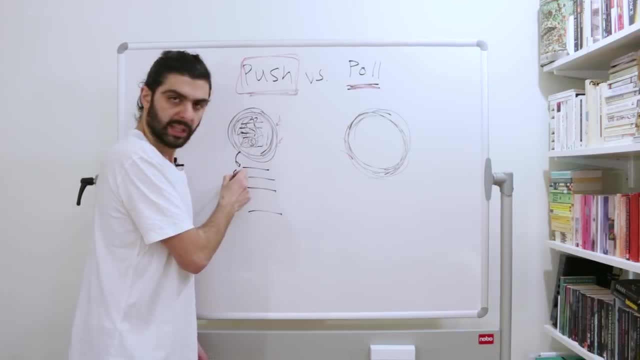 and then you end up in state four, et cetera. Whenever you move to one of these new states, it's this guy's responsibility to push to say, hey, I have changed. You do whatever you want to do, but I have changed. 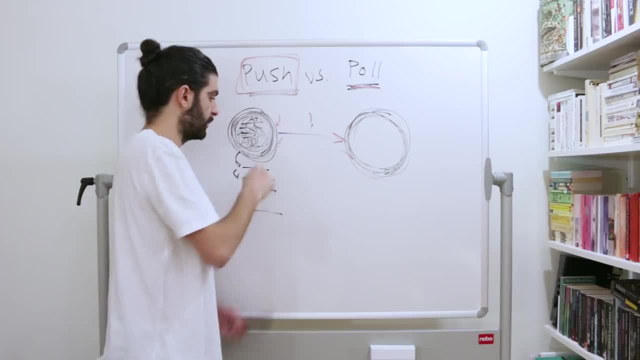 That's one and it's not pulling. We're not doing this over and over and over again, We just do it when you have a change. So you have a change, you push. You have a change, you push right. 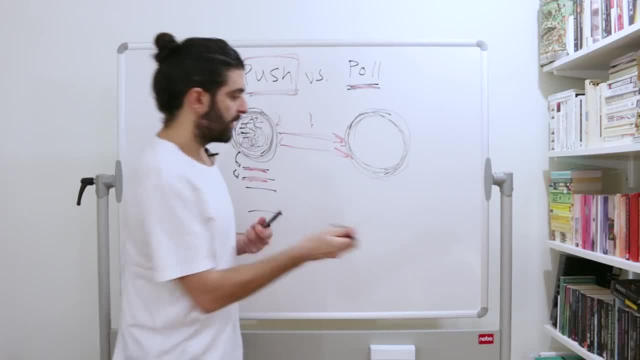 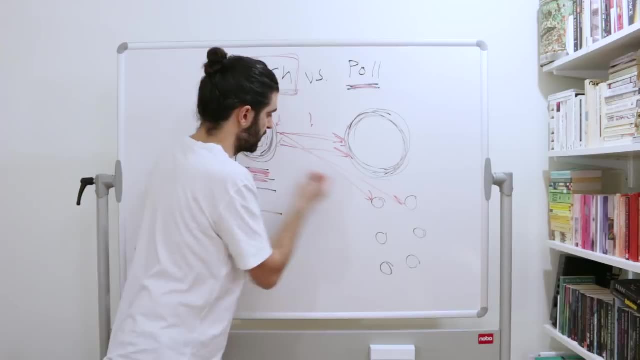 You push the notification of having changed, And the same thing goes for tons of these other ones, So you have lots of them. Whenever you have this change, you say okay, push to all of them. I have changed, I have changed, I have changed. 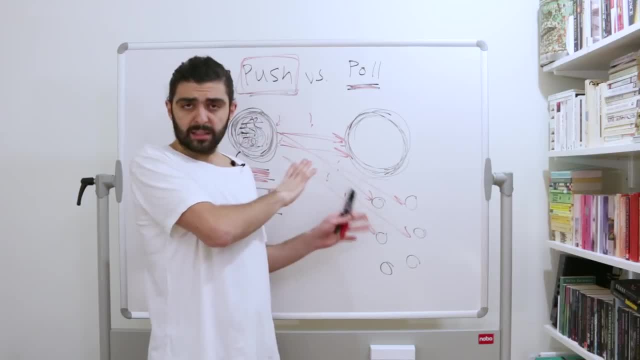 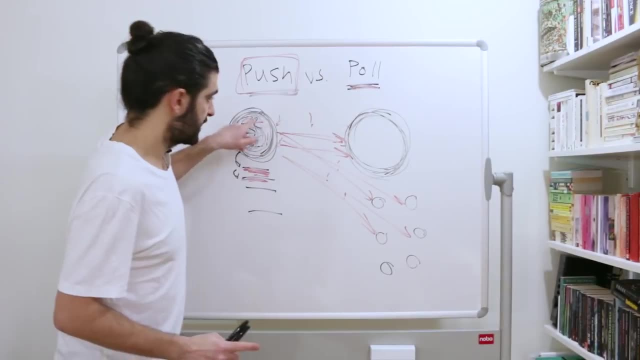 Doop doop, doop, doop. Exclamation point to all of them And in essence this is the observer pattern. Then it's just the syntactics of how to actually build that. But now we're assuming that this guy has some knowledge. 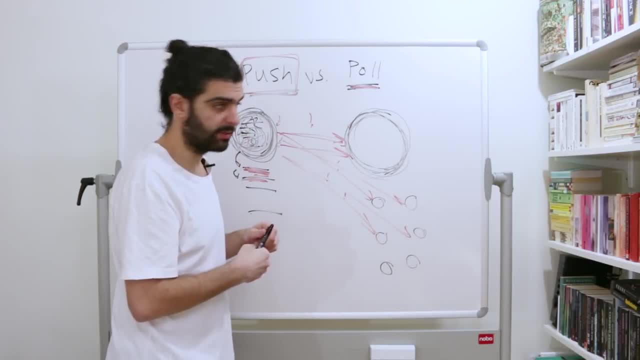 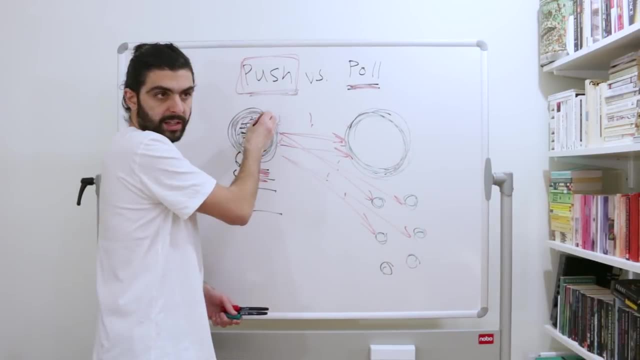 about who these subscribers are right, And that's kind of the essence of observer pattern. Somehow, before we can do this, pushing all of these guys, they need to register to this subject, They need to register to this observable. So these guys are observers. 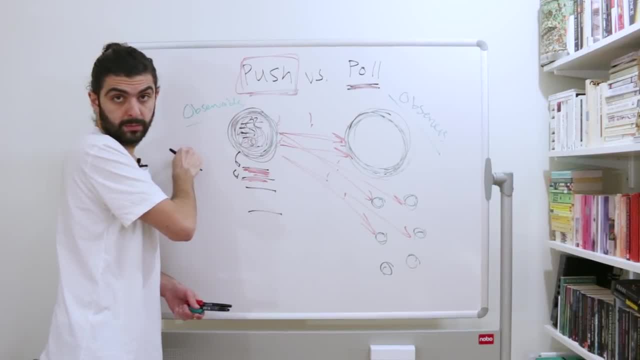 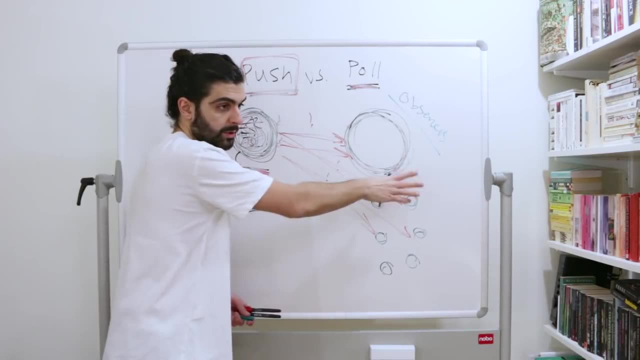 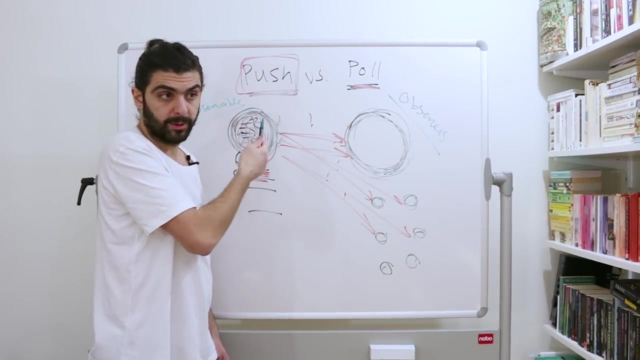 and this guy is an observable. Observable is being observed by observers. When the observable changes, the observers are notified. And in this book and in lots of programming languages the observable is sometimes referred to as the subject. So if you read head first, they'll talk about this thing. 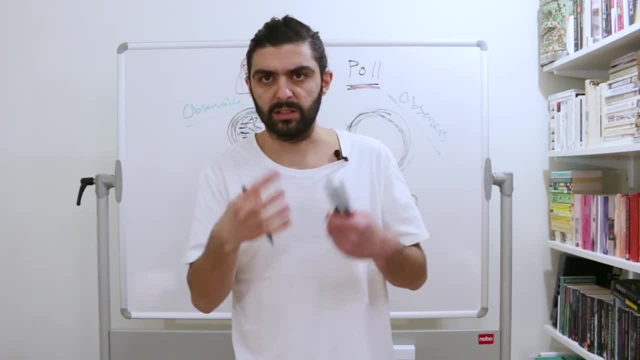 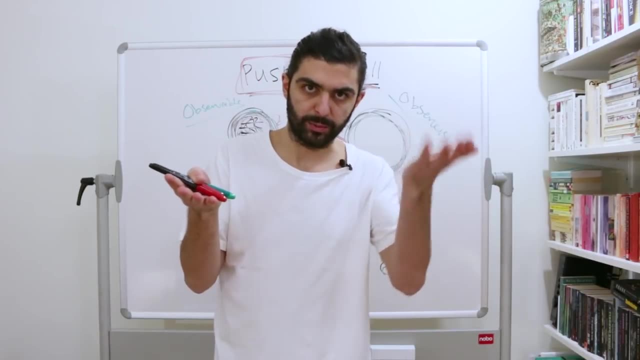 as the subject, But I think it's easy to get confused about what a subject is, So I think it makes a lot more sense to just think about it in terms of something that's observable, and then you have observers that observe the observable. 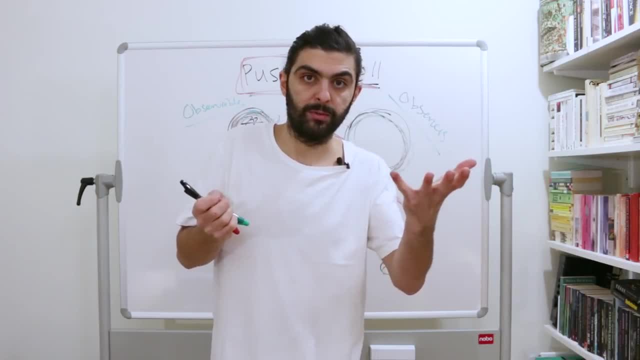 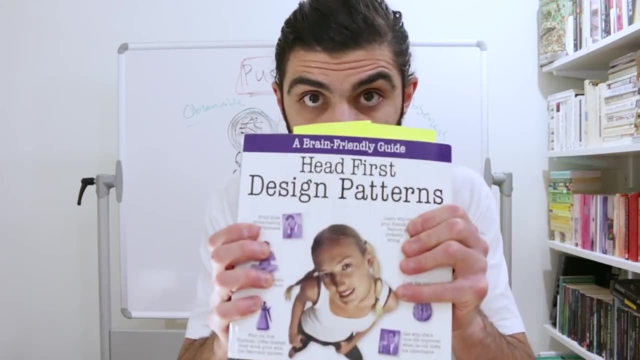 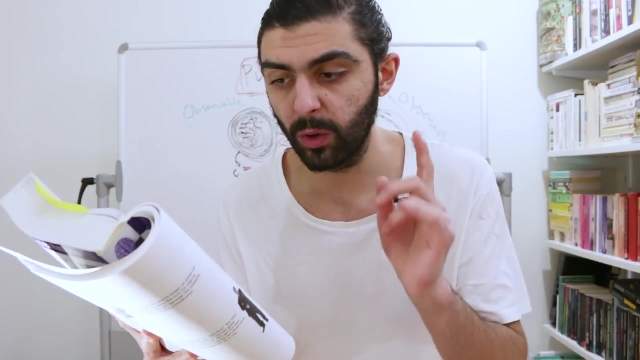 Something can be observed and others can observe. So that's the observer pattern in a nutshell. Let's now dig into the actual definition from the head first book. So they say: the observer pattern defines a one-to-many dependency between objects, so that when one object changes state. 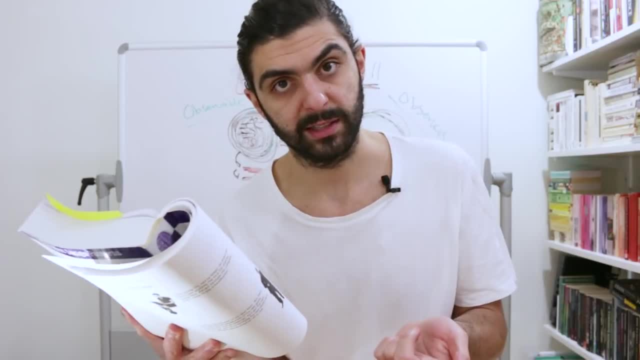 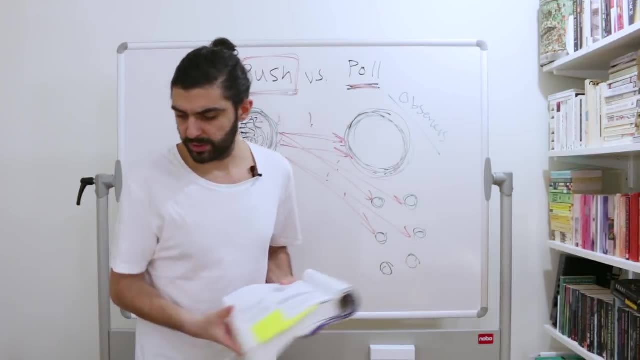 all of its dependencies are notified and updated automatically. Let's look at what we've drawn and let's think about this. The observer pattern defines a one-to-many relationship. So what's a one-to-many relationship? A one-to-many relationship is when you have one thing. 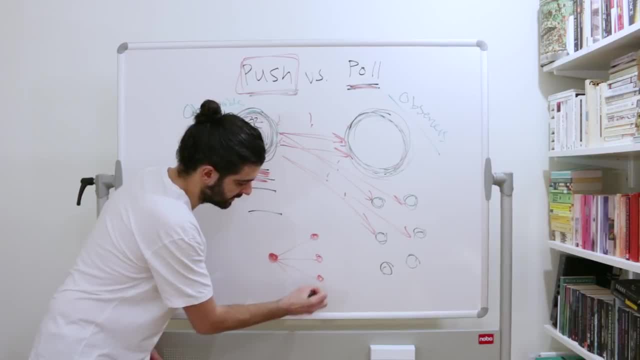 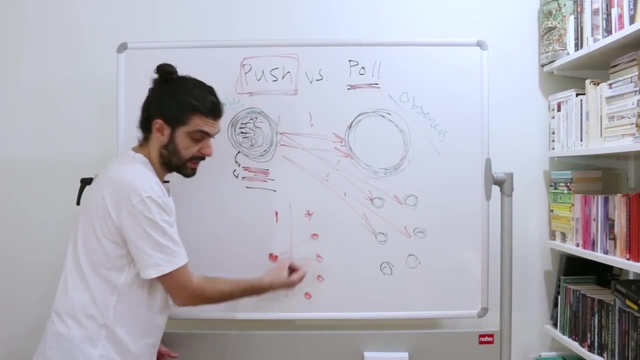 that has a relationship with many other things. So you have one here and you have many here. On this side you have one and on this side you have many. So that's why we're saying it's a one, two, three, four, five. 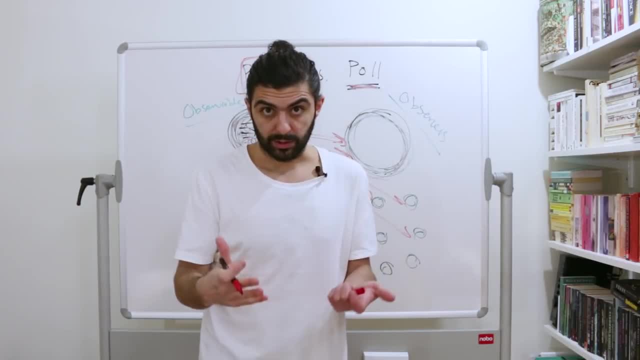 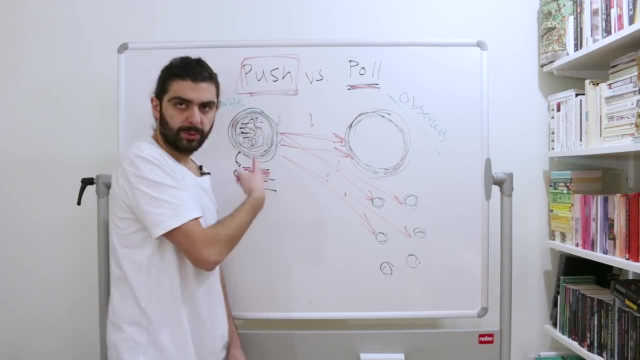 two, many. Exactly as in entity relationship diagrams and relational databases, You have a one-to-one, one-to-many or many-to-many. So this is a one-to-many relationship And if you look at what we've drawn- except from the fact that it's very fuzzy- 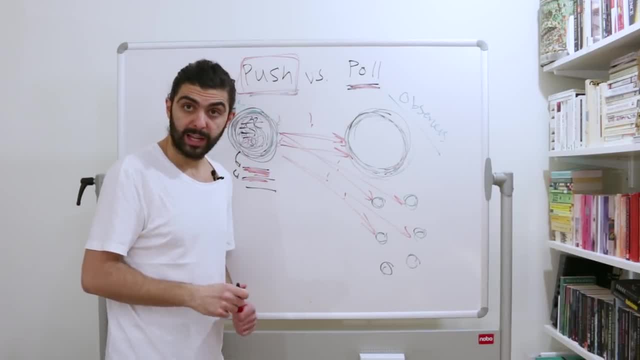 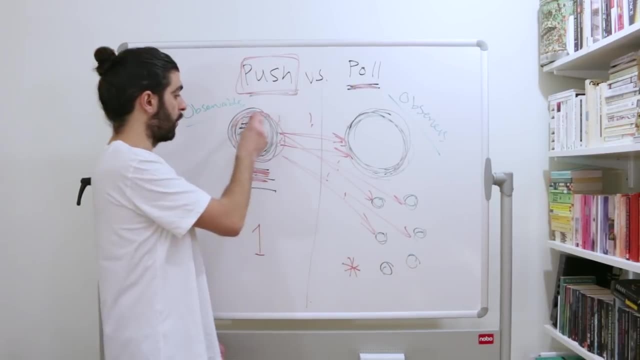 and kind of sloppy. apologies, but what we've drawn is we've drawn a one-to-many relationship. You have one thing here on this side. On this side you have one and on this side you have many. The one thing has a relationship with many other things. 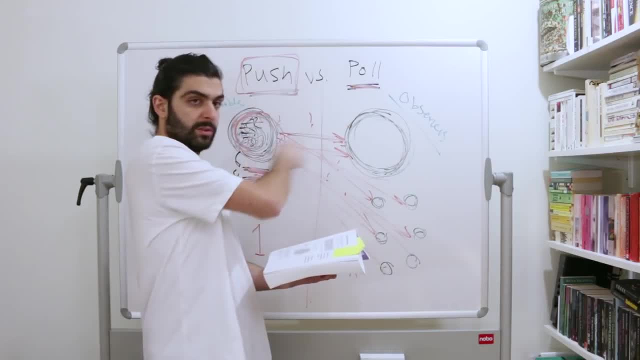 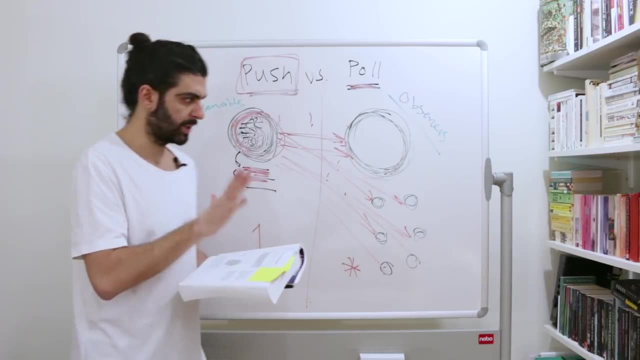 One-to-many. So that's what we're saying. The observer pattern defines a one-to-many dependency between objects. these are objects, so that when one object changes state- not just any object in this context- it's this object. When this object changes state. 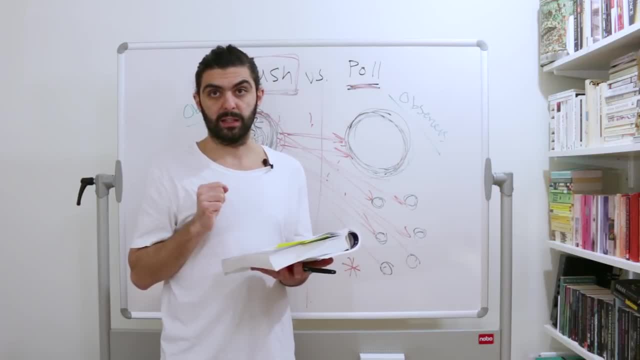 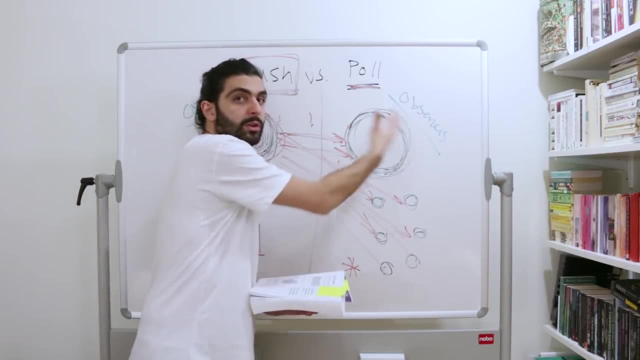 all of its dependents are notified and updated automatically. All of its dependents are updated and notified automatically. So again, this thing changes state and all of these guys are notified of the fact that this has changed state, And that's it. 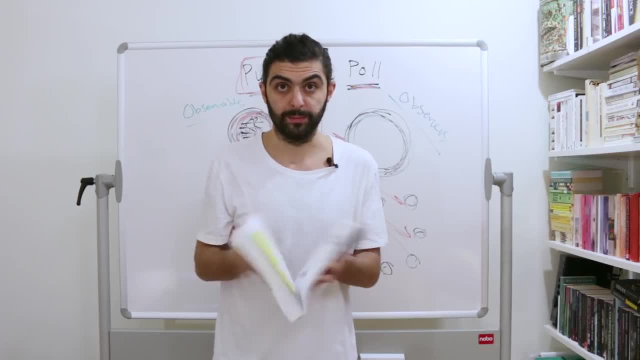 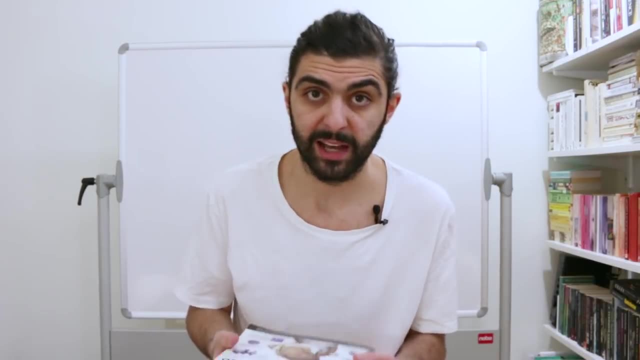 It's really not any more strange than that. Let's now dig into the UML diagram. So before we draw the UML diagram, I want you to be cautious of the fact that different programming languages have different default implementations of the observer pattern. 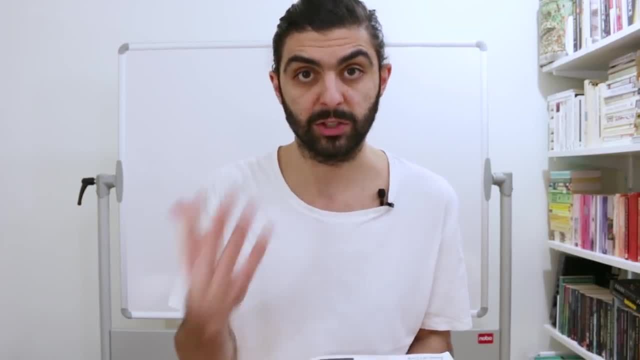 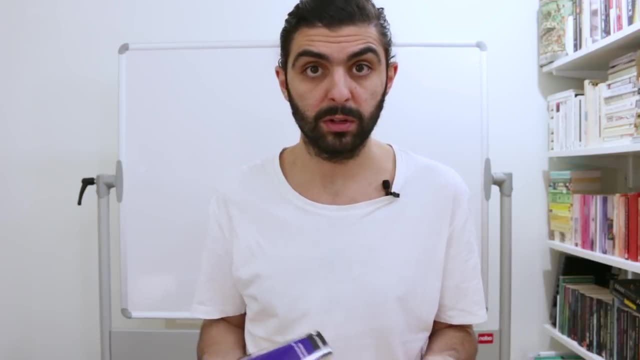 and different people draw different diagrams because there are variations of observer patterns. If you Google observer pattern, for example, if you image Google, you'll see slight variations in the pattern. I guess we could deem all of these observer pattern and these are flavors with advantages and disadvantages. 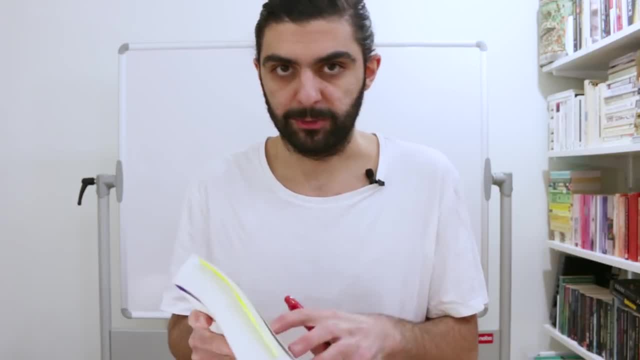 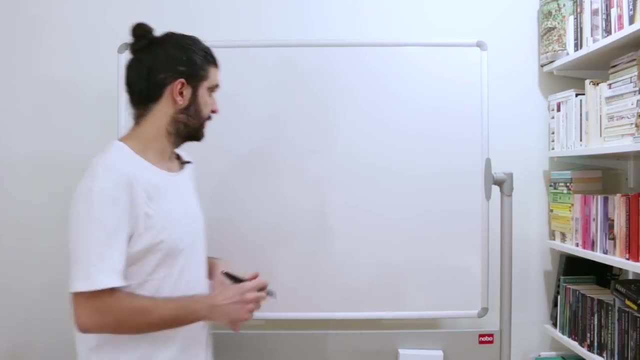 So I'll draw the one that's in this book and I'll try and talk about what the benefits of the approach that they are suggesting is, And then we'll look at a slight variation. Let's get into it, All right. so what we've got is that we've got. 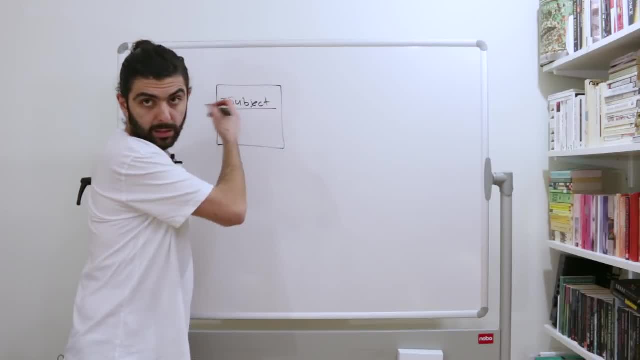 We've got an I subject and remember that when I say I in the beginning of the name, it's just to denote that it's an interface. This is by convention. it has no other meaning. The syntax they're using in the book. 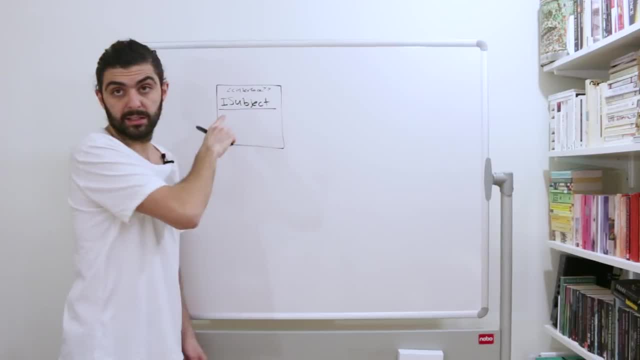 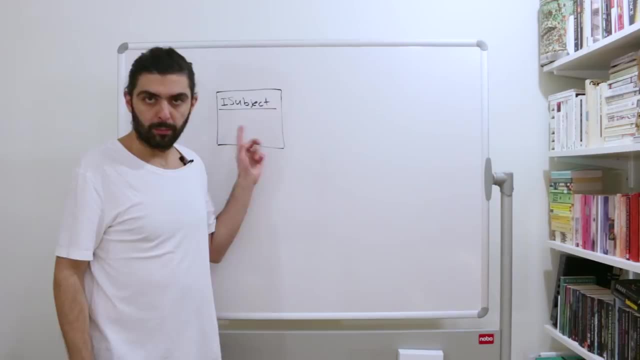 is that they put this node here- interface, to say that it's an interface. But it's quicker for me to just say I subject to denote that what we're talking about here is an interface and not a class. But note here that, as I was saying before, 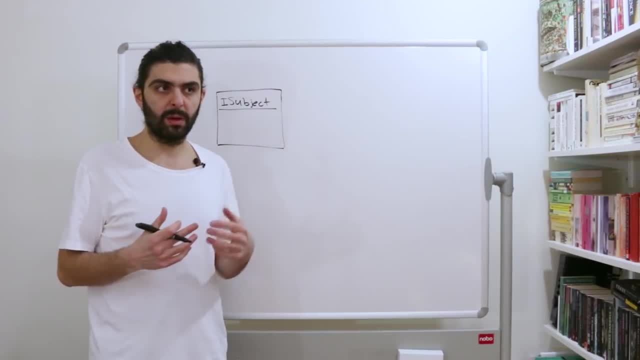 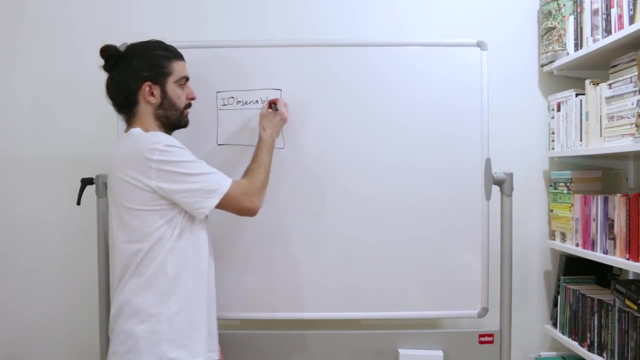 the term they use is I subject. But again, for me it's confusing to remember whether the subject is the observer or the observable. So let's actually rename this from subject at once to I observable. right, This is the thing that can be observed. 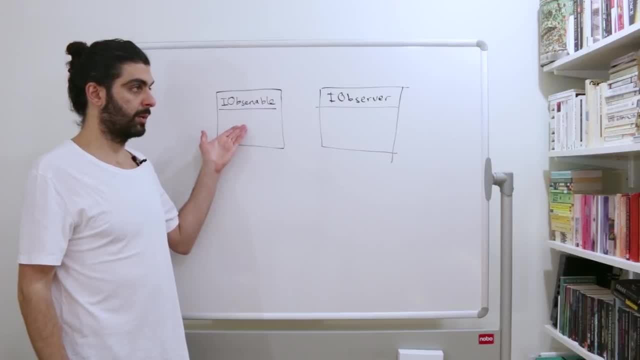 Step one, Step two: I observer, You have the thing that can be observed and then you have the thing that can observe. Notice how we're drawing them in the same places. We had the observable here before and we had all of the observers here before. 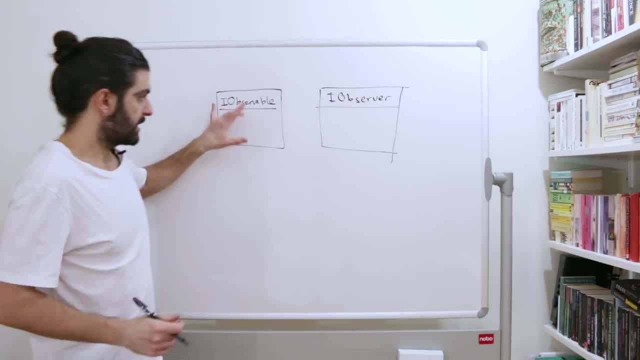 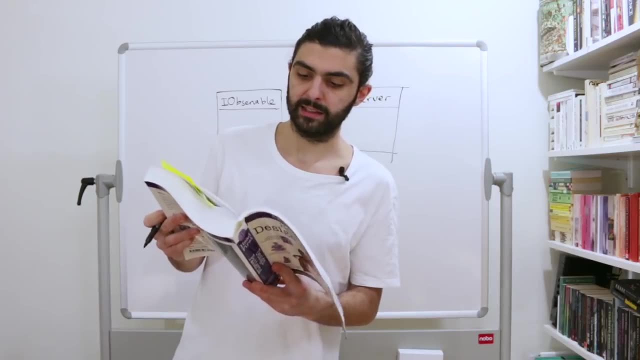 The thing that can observe and the thing that can be observed. So this is the thing that undergoes changes and this is the thing that's interested in the changes that happen. So notice, in the definition it said that the observer pattern defines a one-to-many dependency between objects. 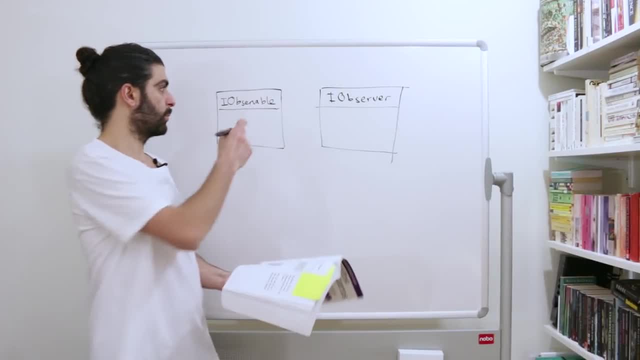 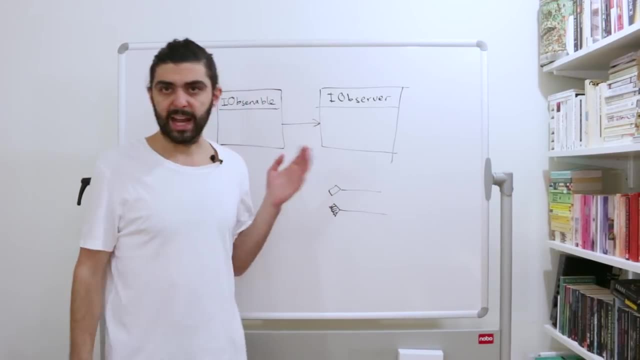 a one-to-many dependency, And this is the dependency we have to draw. We have to say that it's a one-to-many dependency between the observable and the observers. Now, just to be entirely clear, there's the aggregation and composition syntax in UML. 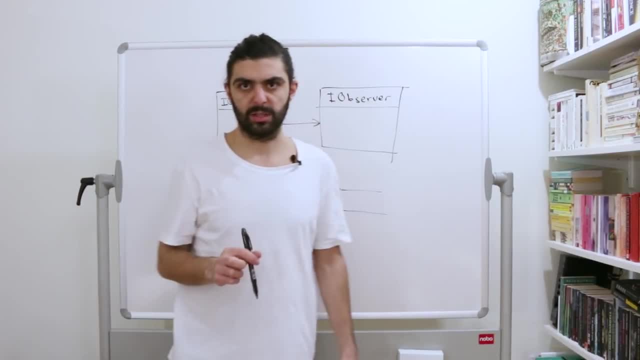 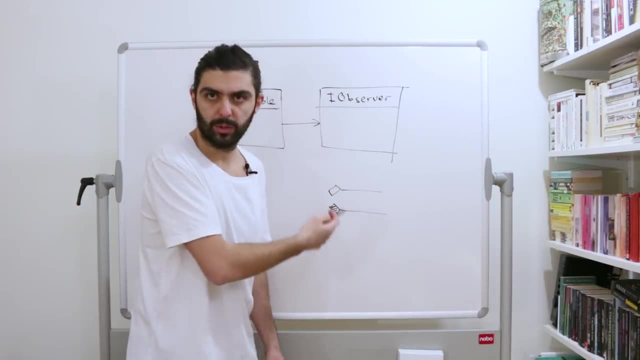 that supposedly can be used to denote a one-to-many relationship, And possibly it's that I haven't fully understood these, but the way I read it, it seems that there are conflicting opinions of how to interpret these. I'll make sure to dig to the bottom of that someday. 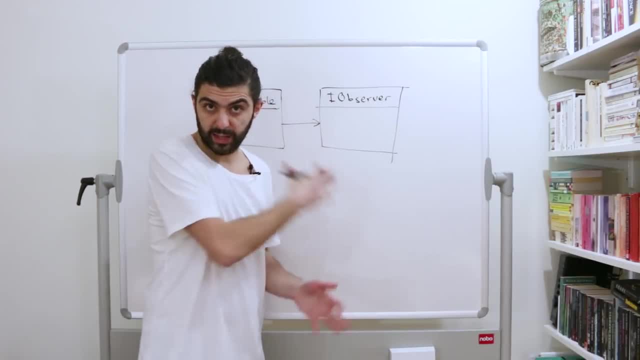 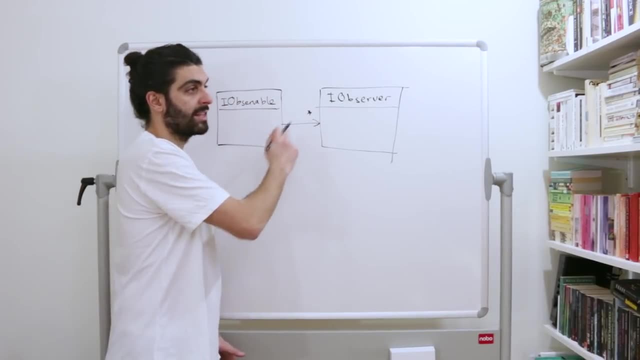 and we'll talk about that in a specific video. But instead of digging into that thing, let's instead just say: I'll just use this star to denote that this is a one-to-many. It's not that an I observable has an I observer. 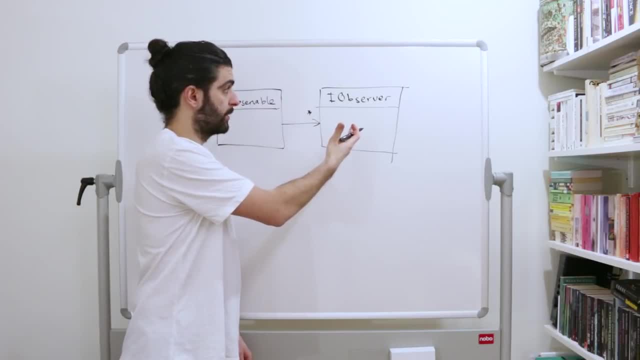 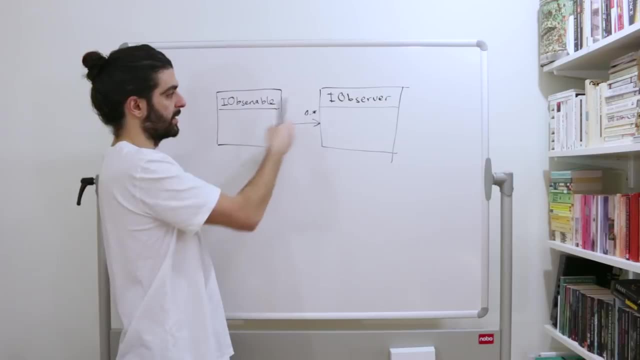 it's that an I observable has zero-to-many I observers. So we could even be super clear by saying zero-dot-dot-to-many. So note that that's in this end. It's not here. It's not that the I observer has zero-to-many I observables. 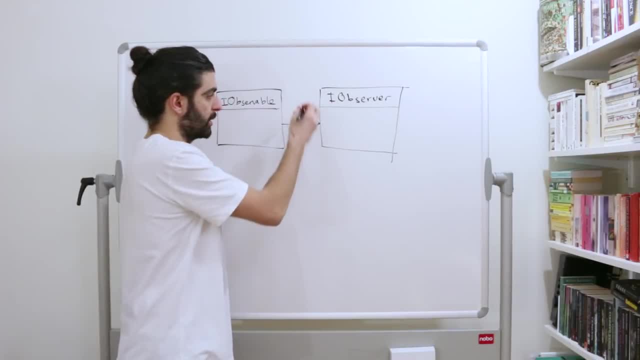 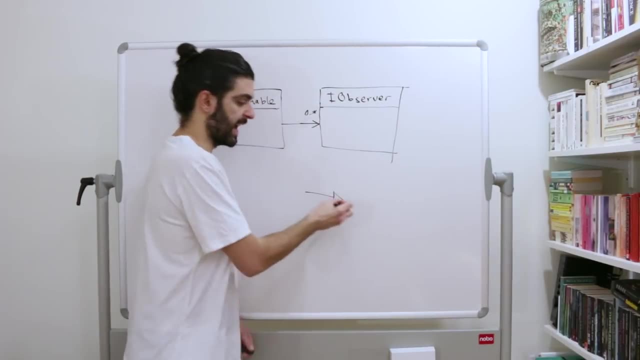 it's that the I observable has zero-to-many I observers, because we've put it in this end of the arrow. And again, remember that this arrow denotes has a and this arrow denotes is a. So we're saying an I observable has many I observers. 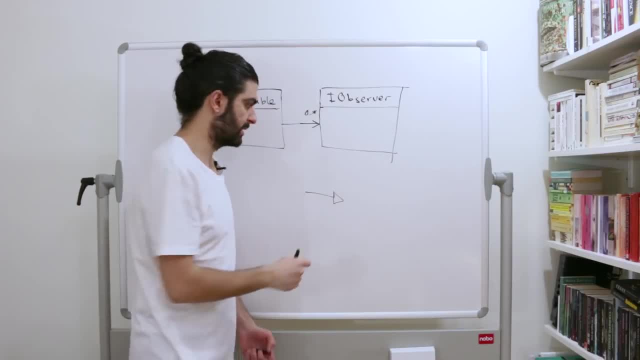 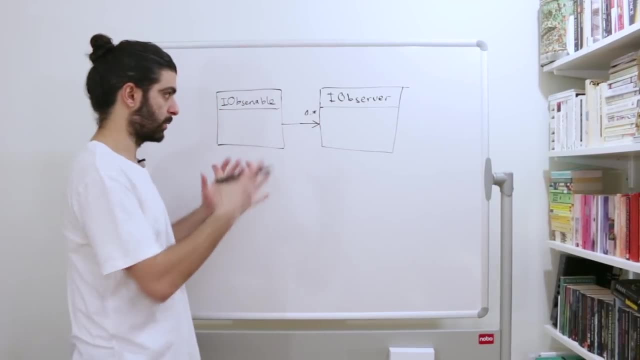 not is many observers, which actually would make sense. but moving on, So these are the interfaces, but then we actually need to have concrete implementations of these interfaces or concrete things that implement these interfaces. But before we look at those, we have to look at what the actual methods are. 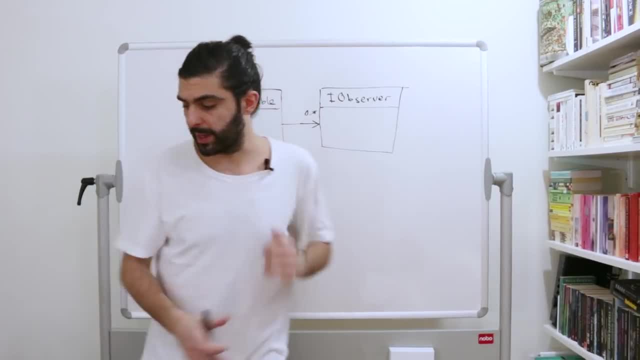 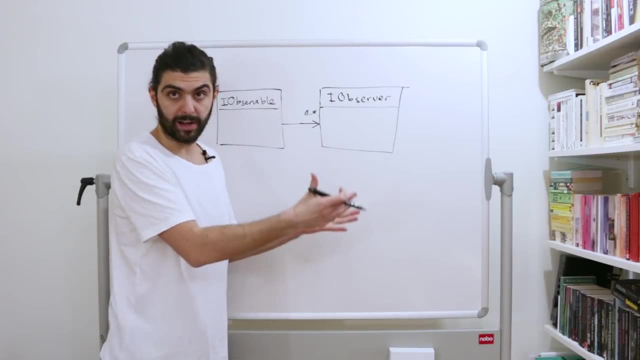 that we expect I observables and I observers to implement. So I observable remember to I observable. we need to be able to register observers so that we can notify them. So that's easy, We just have register. So I'm realizing there's gonna be no room for me. 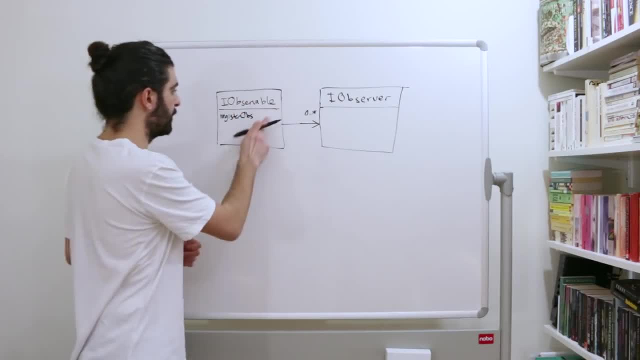 to spell out all of the names, So I'll diverge from the names that they use in the book And I'll just say I'll explain this in a moment. I'll say that the methods that we have are: add, remove. 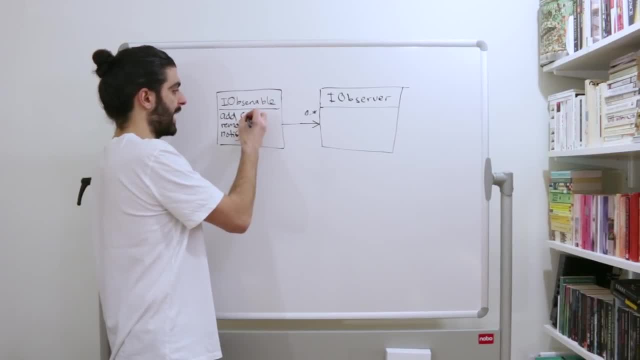 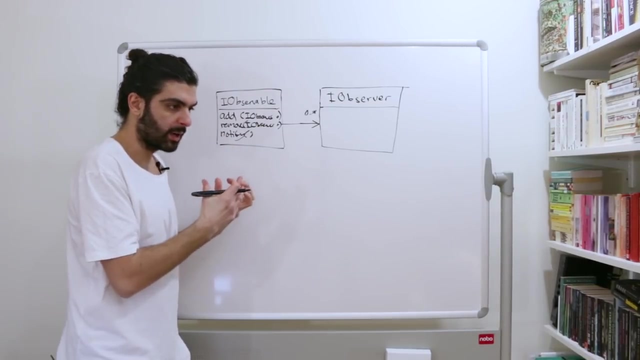 and the notify. So add, takes an I observer, Remove, takes an I observer And notify. takes no arguments. Now, what are these methods? So the thing is that I observable needs to be able to keep track of who wants to know when something changes. 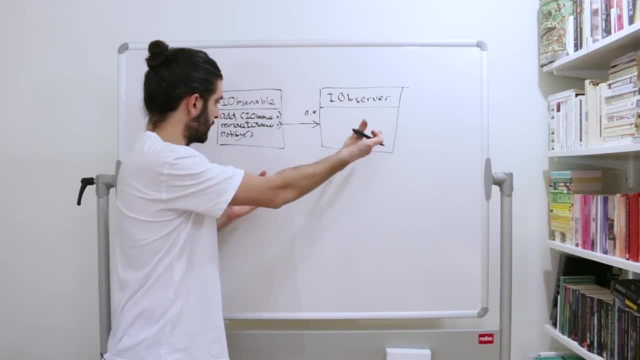 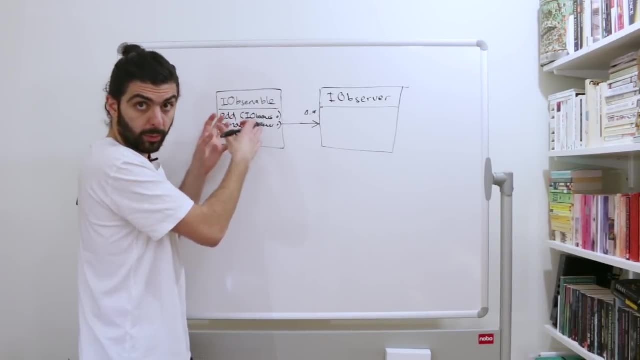 And the things that want to know are observers. So somehow we need to be able to add instances of observers to an instance of an observable. So this is why we have add and remove. So in the book they call these register observer and remove observer. 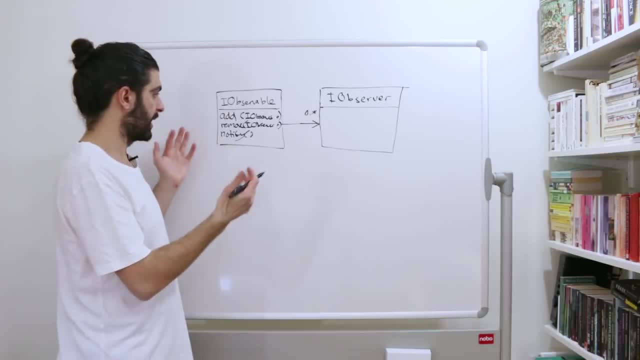 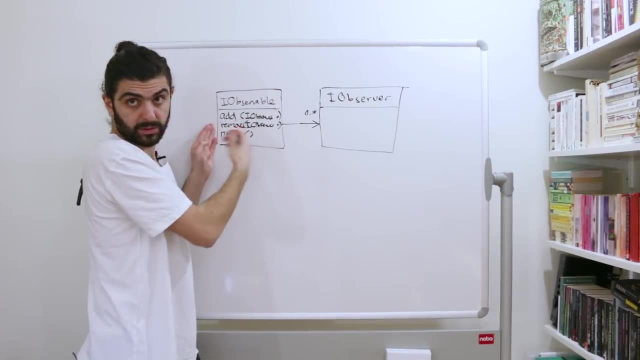 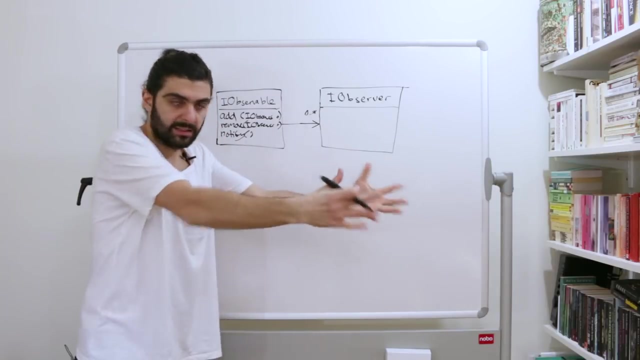 Other common names are register and unregister, But essentially we're then talking about add and remove. We're adding observers to the observable or we're removing observers from the observable, And then the method notify is essentially the method we can call to broadcast the fact that this has changed. 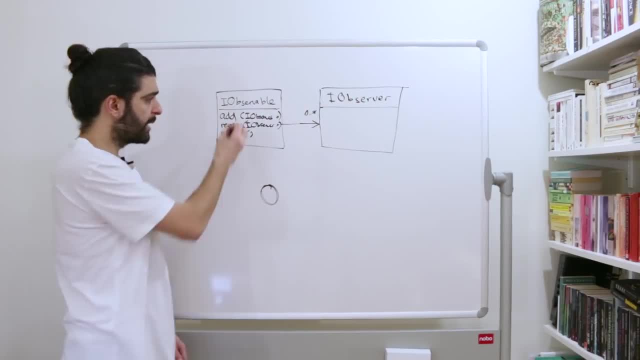 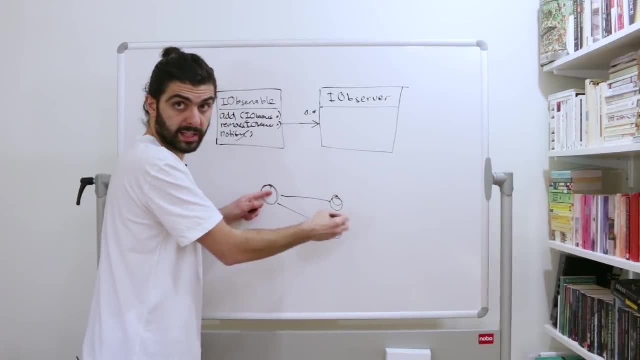 to all of the observers. So you have an observable and when you call add, you add an observer, And then, when you call add again, you add another observer. Of course you pass these observers in. You call add again, add another observer. 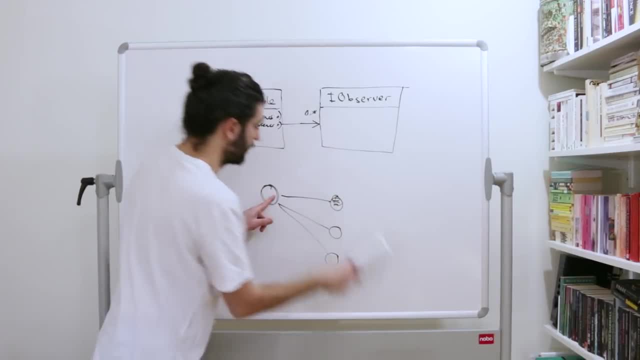 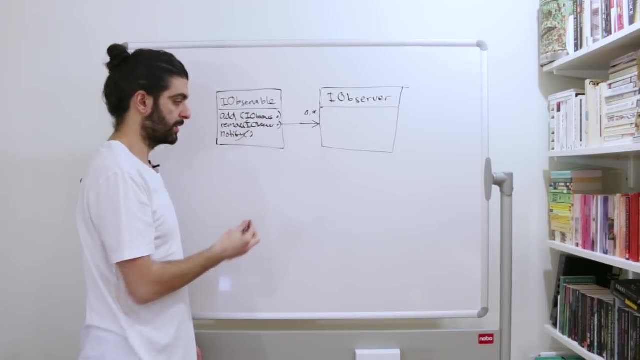 But then you maybe call remove and pass this one and that means that we remove this observer. So, concretely, the observable has some kind of a function. It's a kind of collection that contains a bunch of observers, Whether that is an array. so we have 01 and 02 and 03,. 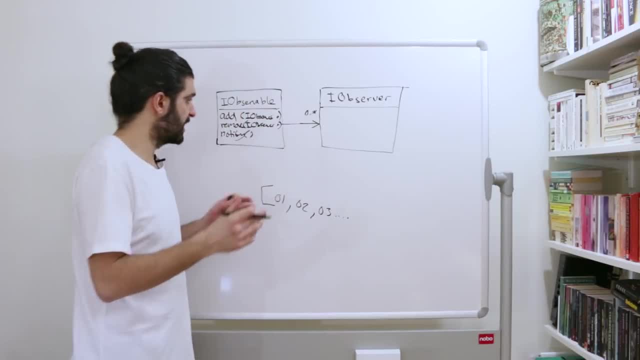 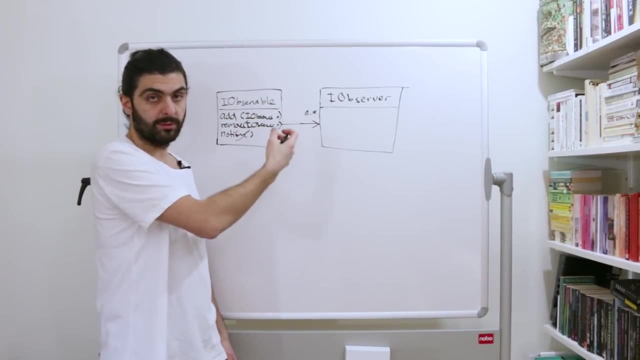 et cetera, et cetera. Or whether it's a hash or a dictionary, doesn't matter. That's an internal of an implementation of an observable. So this is why we have add and remove. We can add in observers and we can remove observers. 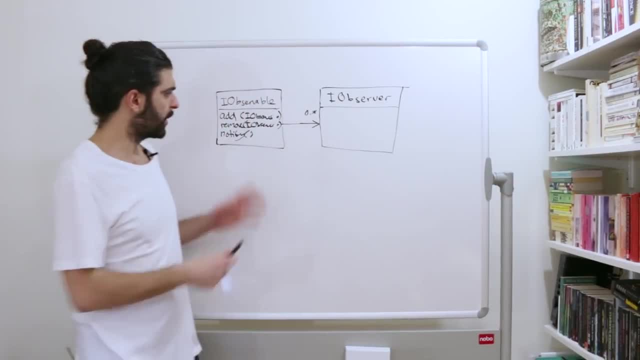 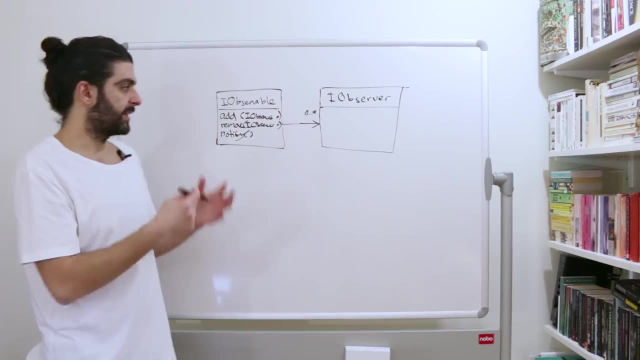 And notify again is when we do the actual broadcasting. Okay, so these are the interfaces. Let's now talk about the actual implementations of these interfaces, or concretions that implement these interfaces. So we have a concrete observable and we have a concrete observer. 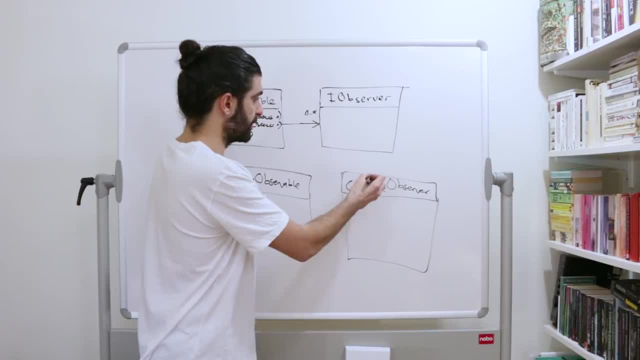 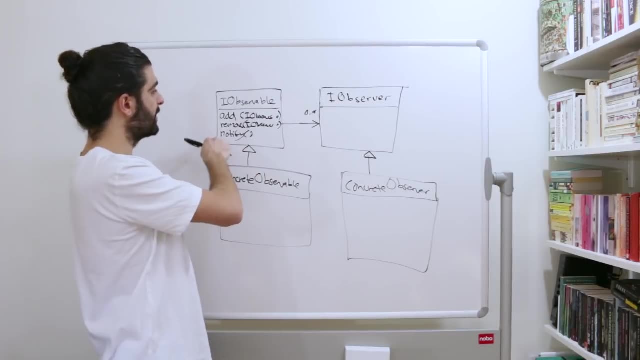 What's the relationship here? Perhaps quite obviously. the concrete observer implements the IObserver interface. The concrete observable implements the interface IObservable. Concrete observer implements IObserver. Concrete observable implements IObservable. This is a concretion of this interface. This is a concretion of this interface. 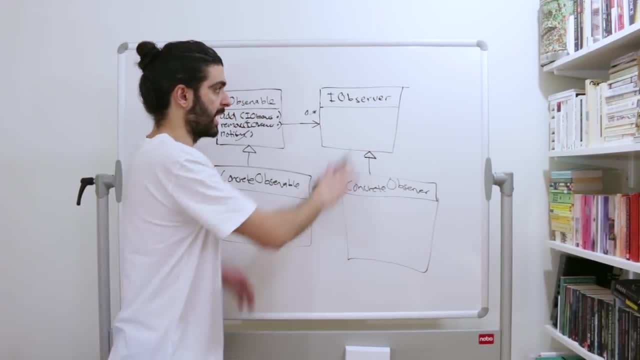 Ah, I'm now realizing I actually forgot to add the methods here. Before we get into this land, we should of course figure out what the methods are here, So let's do that first, And that's actually pretty simple. The contract is essentially a single thing. 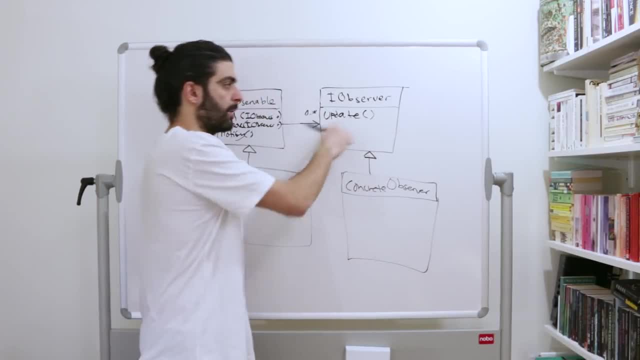 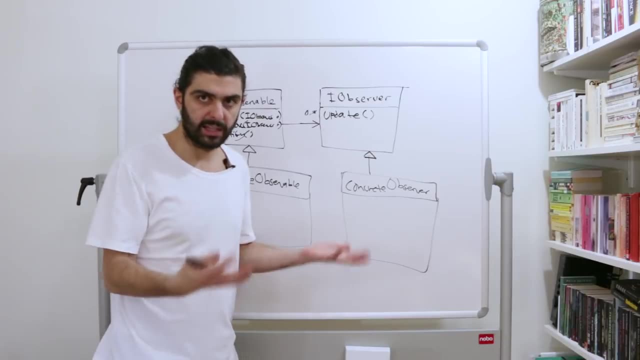 It's that an IObserver should be able to respond to a call to the method update. In other words, the observable wants to notify all of the observers. And how does it do that? It does that by calling the method update. So you instantiate observers. 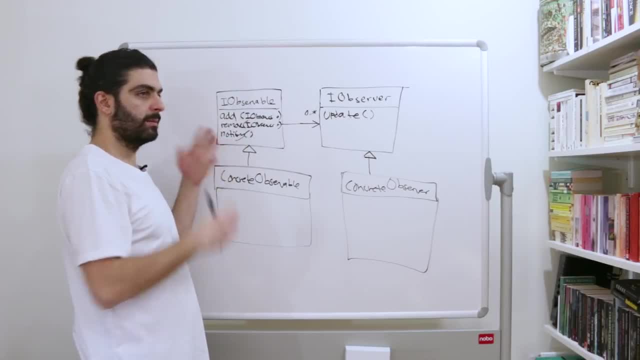 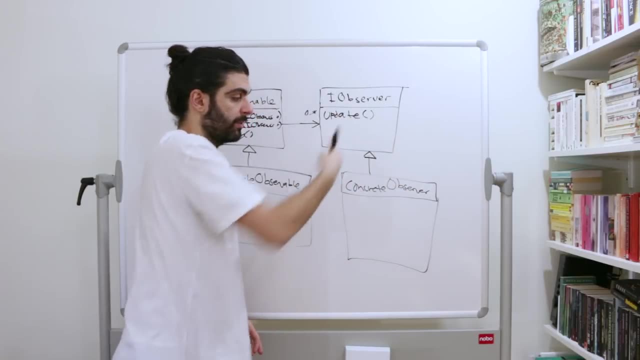 you add them using the add method and then, whenever you call notify, whoever calls notify the observable instance will then call update on all of the instances of the IObservers. Again, observable has a relationship with many observers. These register using the add method. 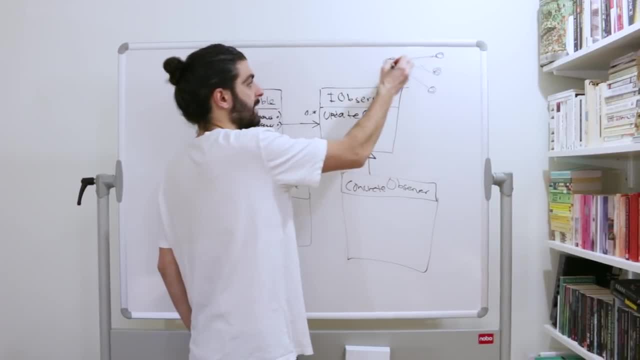 We take this one and we say add, it's added. We take this one and we say add, it's added. Take this one and we say add and it's added. Then when we call notify, we'll notify all of these. 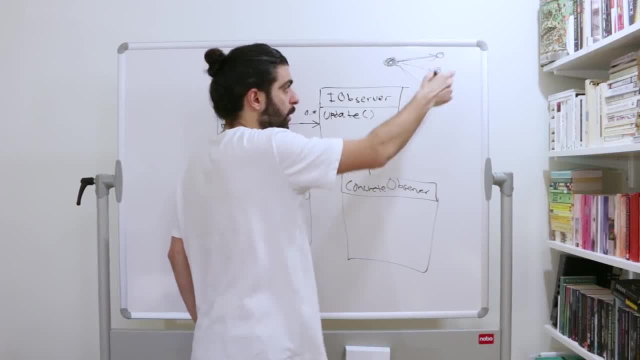 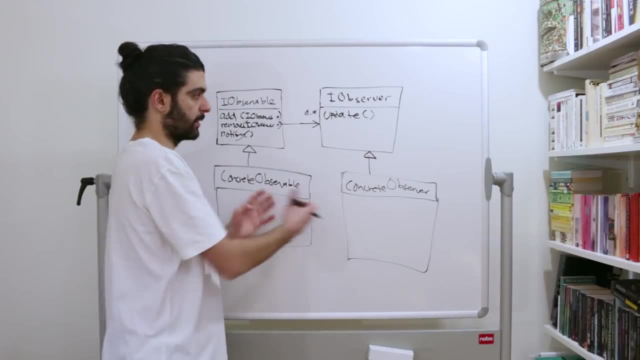 by calling update, update, update, And they, the concrete observers, will be responsible for whatever they want to do when update is called upon them. Let's move on. So, because these are concretions and they implement the interface, we can just copy the signatures of the methods. 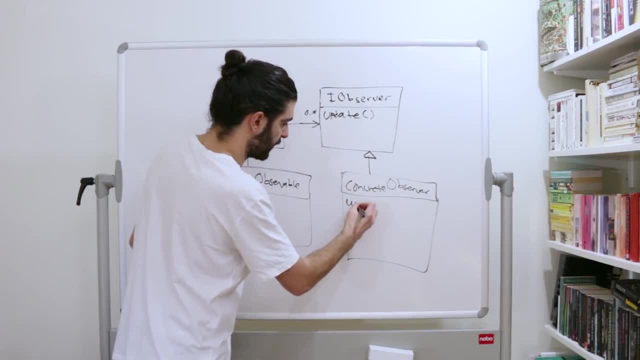 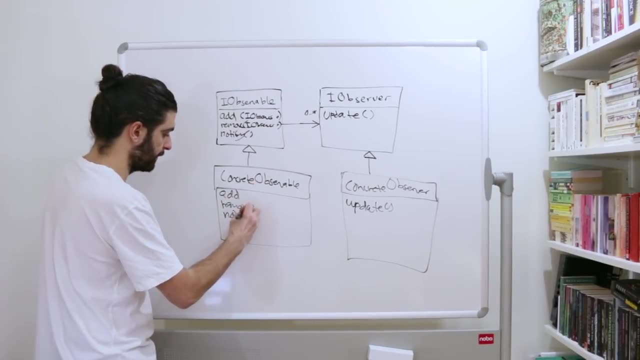 because of course they need to implement these methods. So the concrete observer needs to implement the update method, The concrete observable needs to implement add, remove and notify. Pardon my crappy handwriting, Same thing as here. I've just sort of taken the signatures. 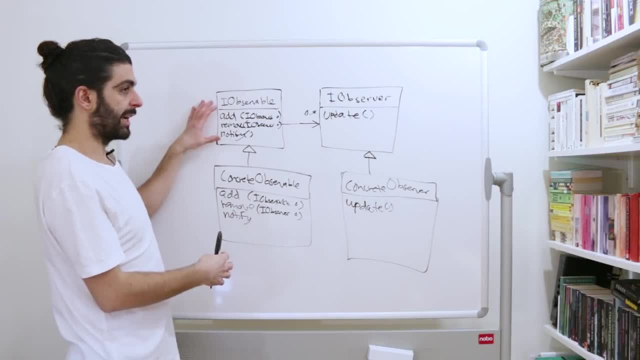 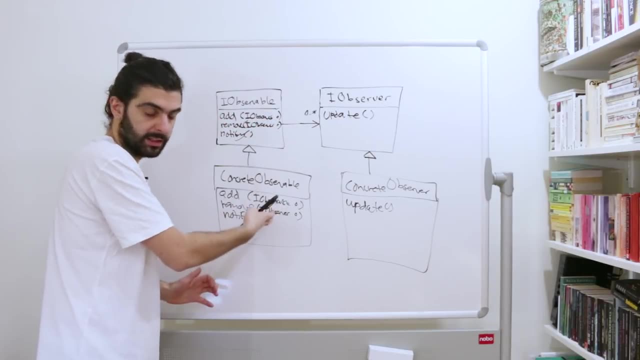 and copied them down here. But here we have concretions. Here we just state that this method needs to be implemented and needs to have this signature, This is the contract, And then here we actually need to implement these. But what does concrete observable also have? 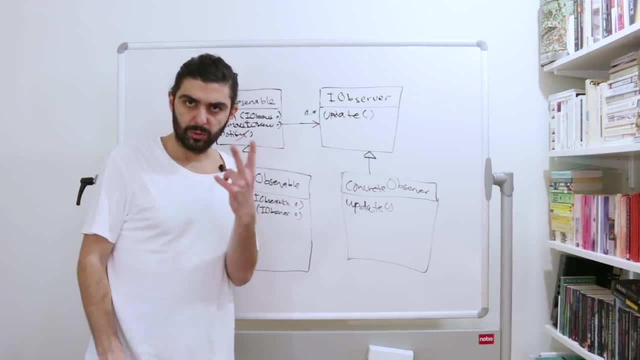 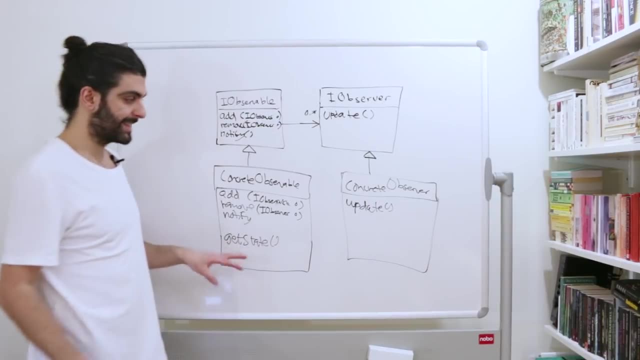 We'll dig into why this is, But the book suggests two methods. It suggests that you should have get state and set state. I'm going to ignore set state, because set state they're essentially only using for this application to do anything sensible. 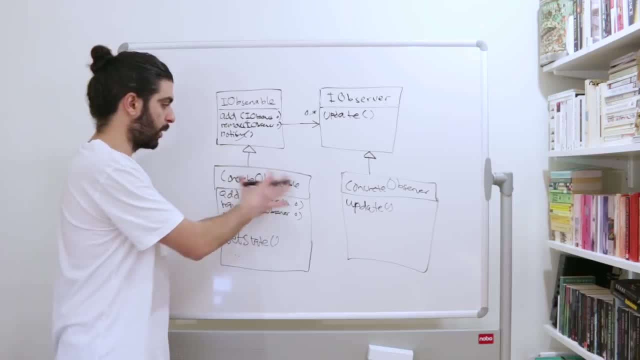 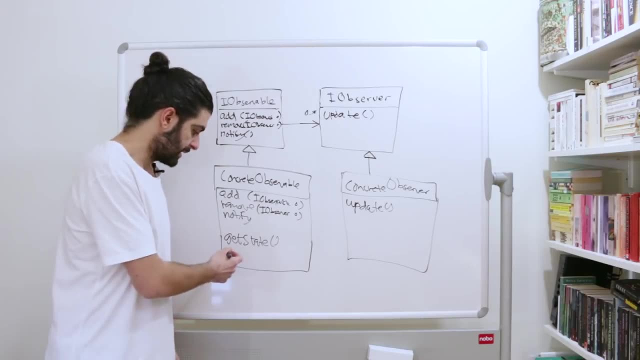 I'm sort of just leaving that unsaid because I want to emphasize that the concrete observable would be concrete in your scenario and could do anything dependent on your scenario, right? So set state is just a placeholder for whatever your observable would do If it's the collection of articles. 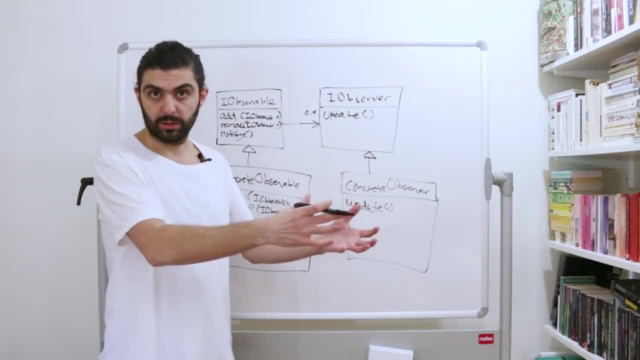 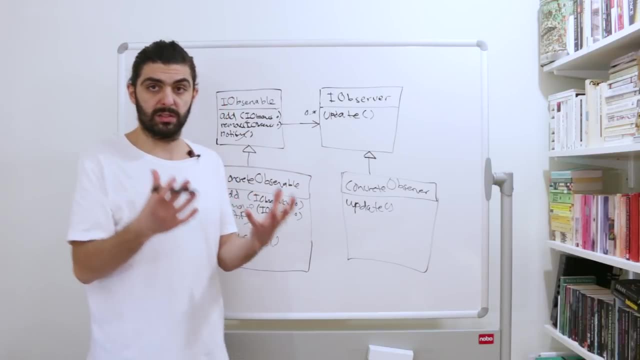 that we talked about before. maybe it's a method that's called save new article or add new article, Or if it's a chat room, for example, that's actually a good analogy. Observer pattern is very susceptible to chat rooms, or chat rooms are very susceptible to observer pattern. 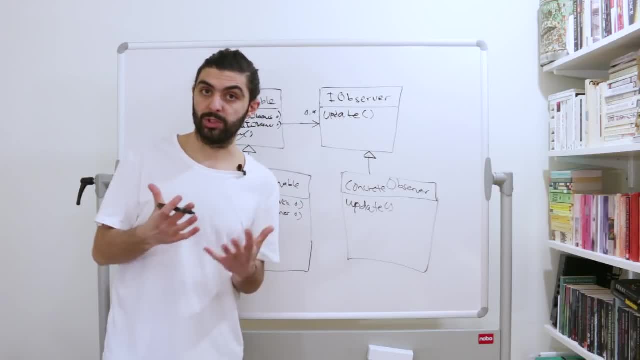 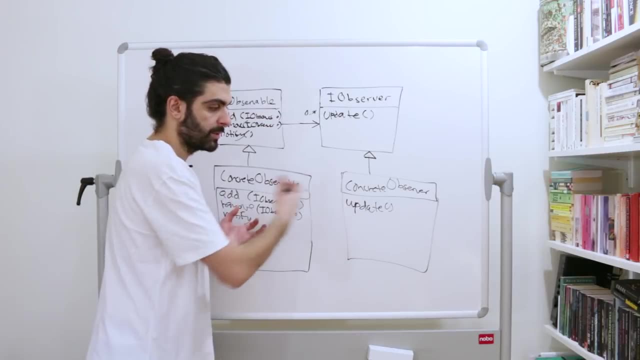 I should rather say Observer pattern is a very suitable architecture for chat systems. So, if you think about it, you have a chat room right, Which is an observable, And then you add in observers to the chat room And then, whenever somebody broadcasts a message, right. 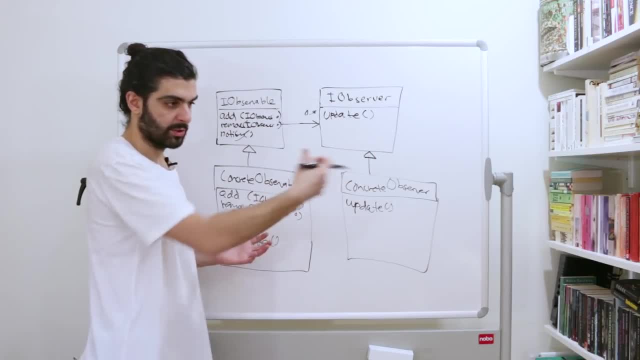 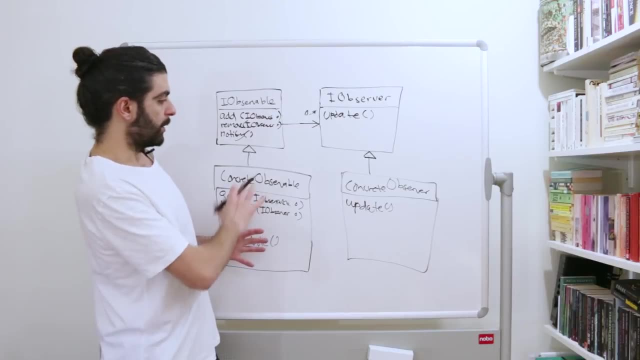 Whenever somebody sends a message- observer sends a message, a user sends a message and they want to broadcast that to everyone- Then maybe we save that here as in: we save a message and then we call, notify, so that all of the clients that are connected to the chat system. 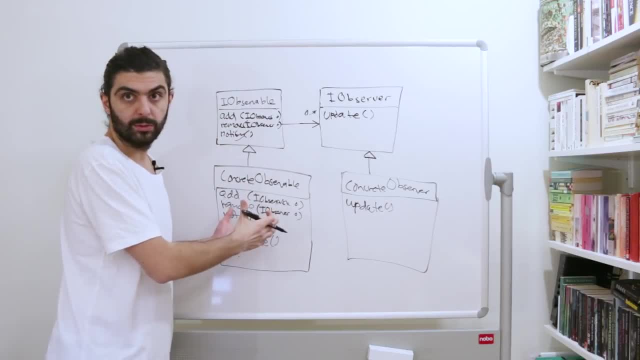 can get the latest message that has been broadcasted by one of the users. I'm saying, set state is again kind of a placeholder. It totally depends on your scenario And get state is actually the same thing, but I think we need it here. 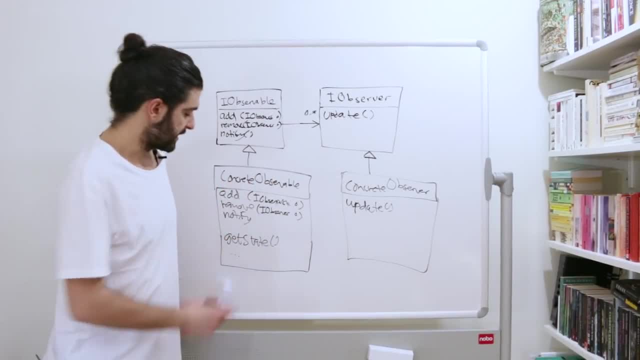 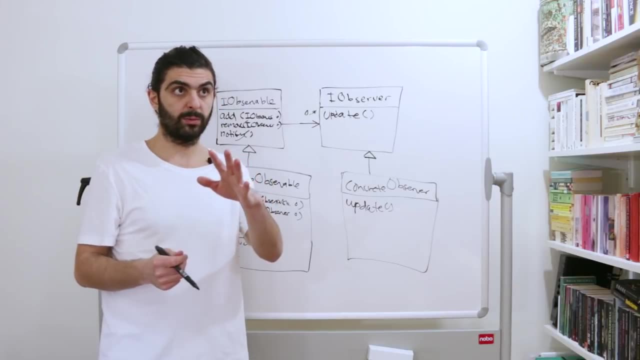 in order to go sort of go full circle with this example, But essentially the dot dot dot here you can think of as that the concrete observable does two things. It's so single responsibility principle people, I'm aware that we're kind of potentially breaking. 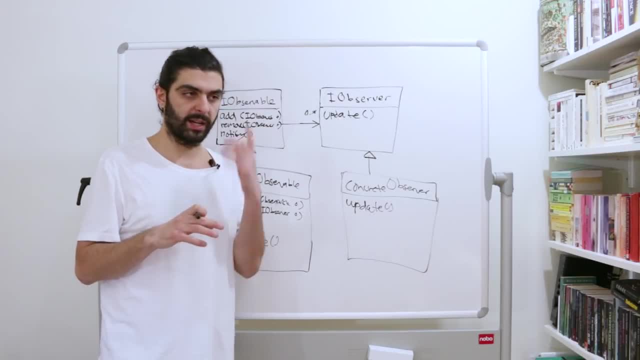 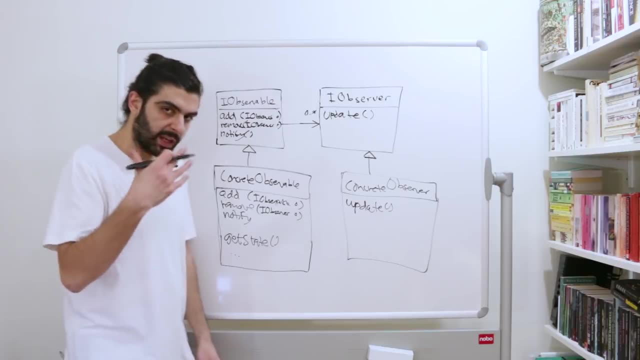 single responsibility principle here, So we'll talk about that some other time. I need to do some thinking and come up with an alternative solution. But if you have an alternative solution, please do shoot that in the comments and we can discuss that. But you can think of it in terms of that. 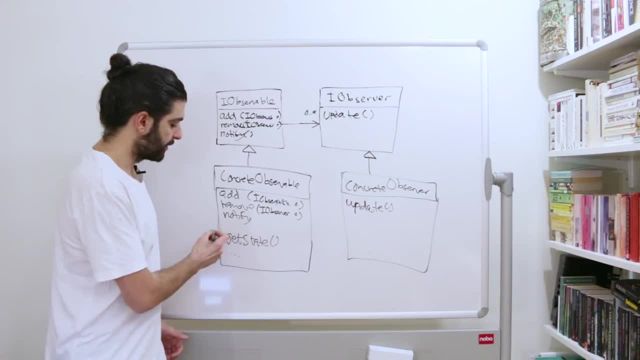 the concrete observable actually does two things. It does whatever it usually does, right, Which is all of the stuff that we put down here- the dot, dot, dot, dot dot, the get state and all of that stuff. But then it also does this stuff. 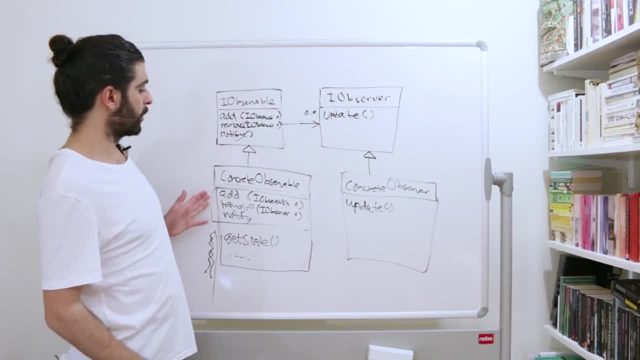 which is strictly observer stuff. And of course now I'm sort of going ahead of myself. but what we could do is that we could move the implementation of these methods into here and make this an abstract class rather than an interface, Because now that we're making it an interface, 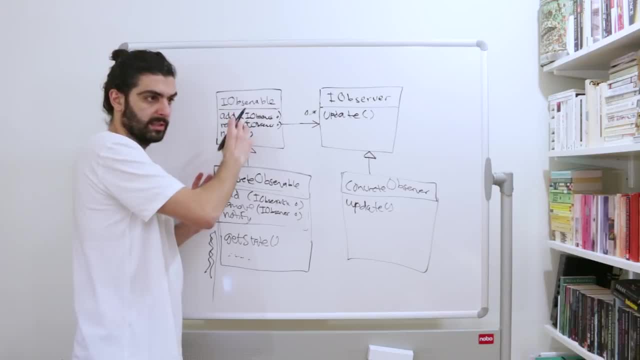 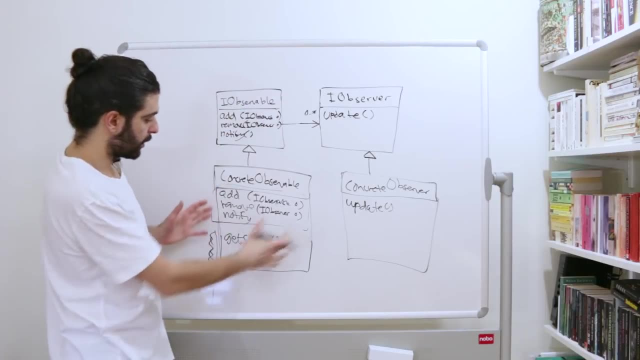 we're forcing the concrete observable to actually implement these methods. But if it was an abstract class, we could have had baseline implementations here and then let the concrete observable do all of this stuff. But let's stick to the book's example for now. 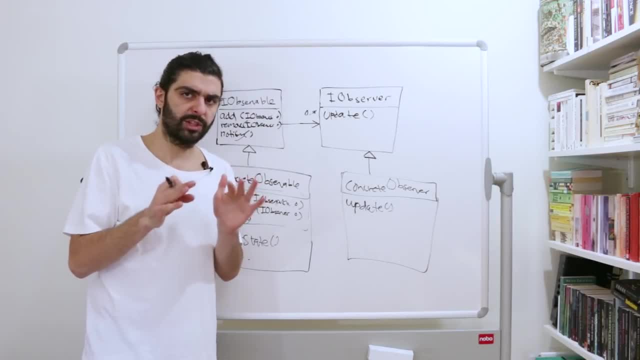 Let's not make it overly complicated, but just be aware that it's potentially a bit shady that we're kind of doing two things. So that's that, And the concrete observer may have other methods, but again, that totally depends on your domain. 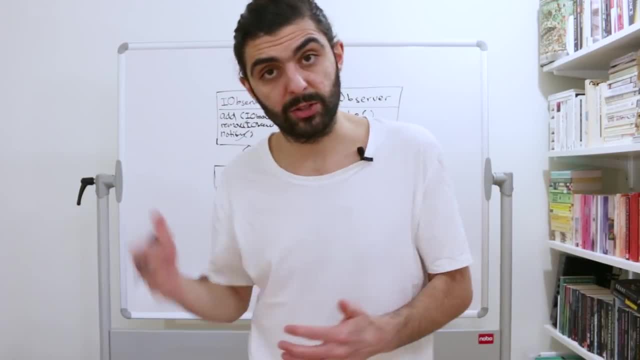 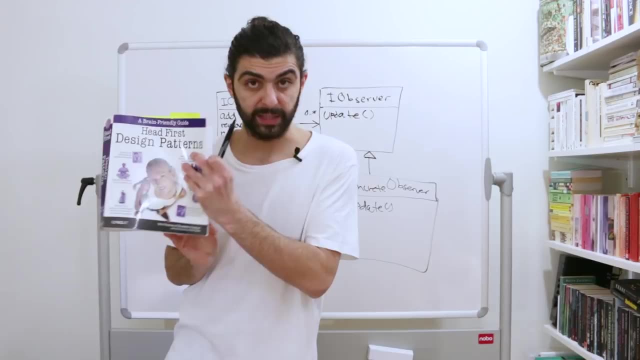 So let's not dig into that now. So I was saying before that people draw different variations of the observer pattern, And some of the variations that you find on the internet stop here. So the pattern essentially looks like this, But the headfirst book actually. 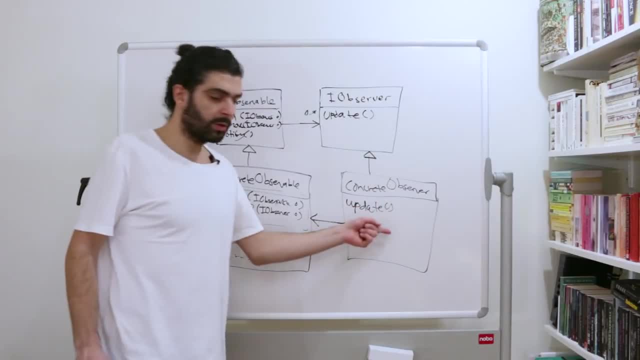 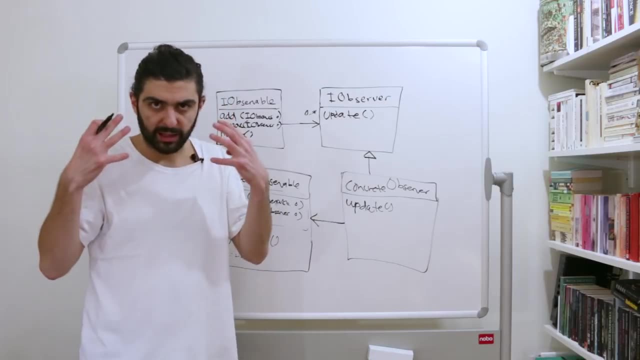 they also introduce this arrow, So a concrete observer has a reference to, has a concrete observable. This, for sure, is what struck me as the most strange thing whenever I'm looking at observer pattern. And it's actually not that strange And it's actually kind of ingenious. 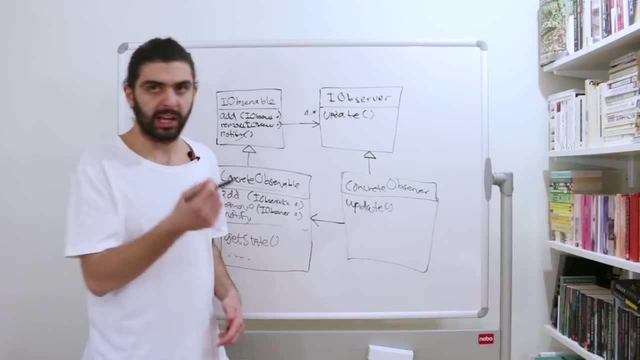 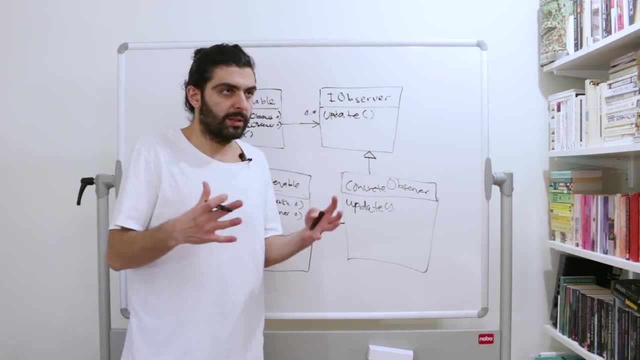 It's kind of smart, But again, more people are confused about this. There's actually a Stack Overflow post that asks: what's the point of this arrow? It's obvious that it causes confusion. It kind of also feels strange because when we talk about design patterns- 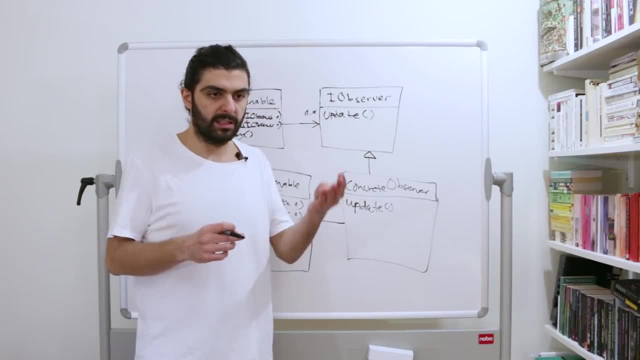 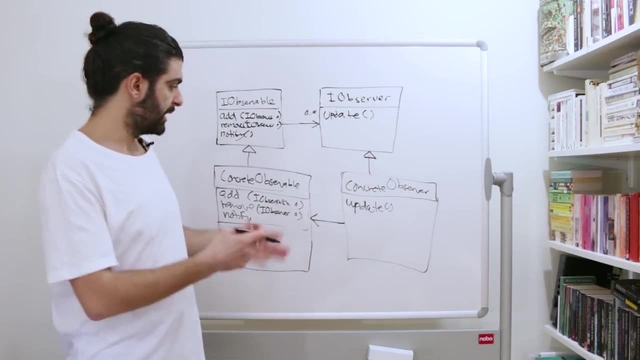 we want to increase abstraction And usually we want to have dependencies between abstract things, not between implementations. We want to have dependencies between interfaces and not between concretions. But here we actually have a concretion that have a relationship with another concretion. 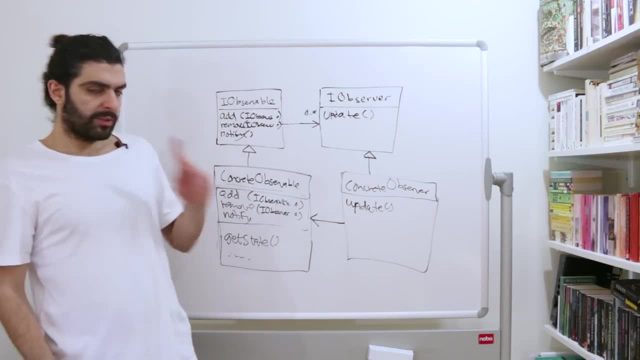 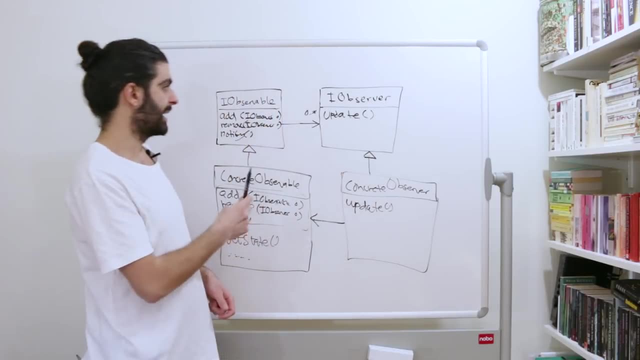 This concretion has a of this concretion, And then the question is: why? So the thing is this: The idea is that when you instantiate a concrete observer through the constructor, you pass a concrete observable Through the constructor when you create an observer. 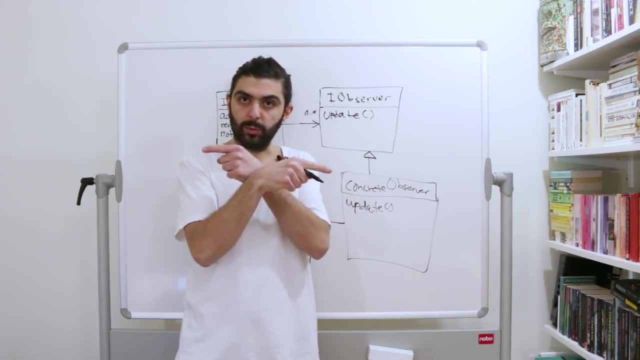 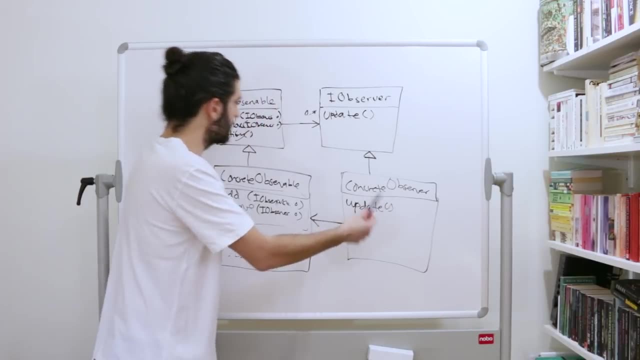 you pass the thing that you want to observe. So it kind of goes two ways. So the observer is passed into an observable via the add method. A concrete observer instance is added as somebody who's subscribing to changes right To somebody who's subscribing to changes. 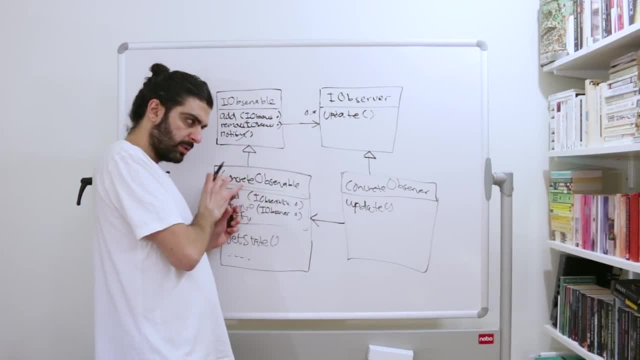 on the concrete observable. But what we also do is that we take, you know, we take the observable and pass it into the concrete observer upon construction of the concrete observer. We'll look at this in code. But the point of this is that when we do that, 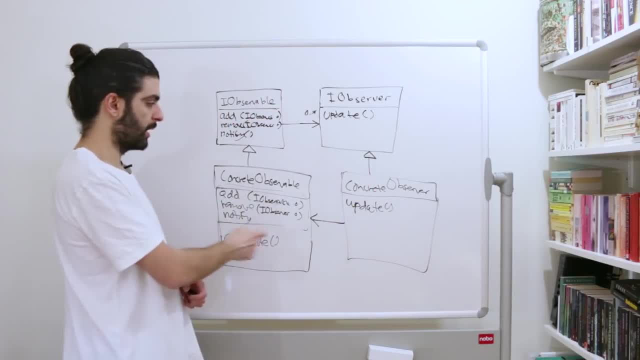 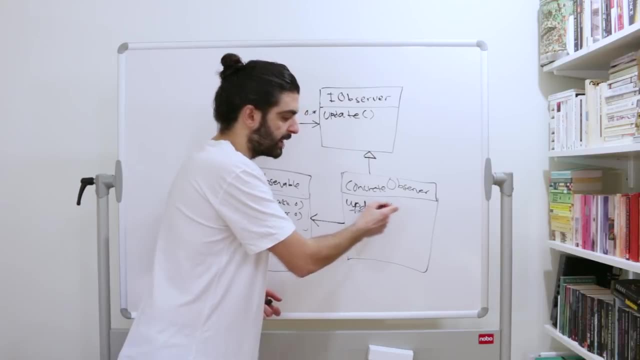 that means that the concrete observer has a reference to the concrete observable that it's observing. And if it has, that when we then call update we don't have to pass anything here in the update method, Because if you think about that, the update method. 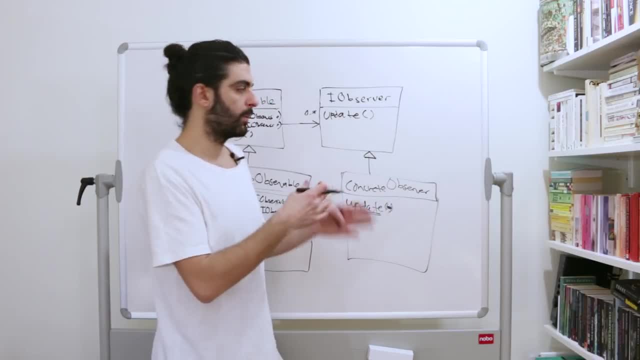 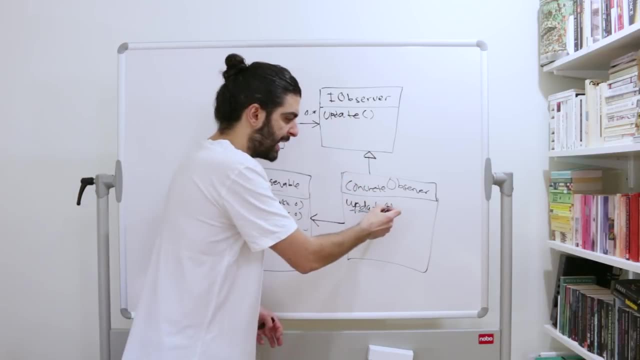 if it has no arguments, then we're just saying that you were interested in knowing when this thing changed, right? You said: register me as an observer. I want to be able to know when that thing changes. But if we're not passing anything here, 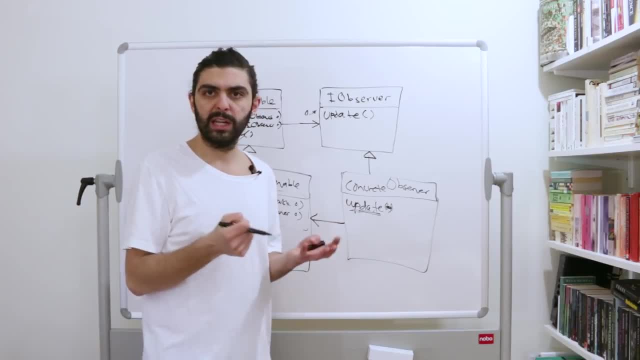 how would you know what has changed? Or how would you know what to read? How would you get the information? You would just know: ah, it's changed, but what has changed? Or how can I read information from it? So that's the point of this arrow. 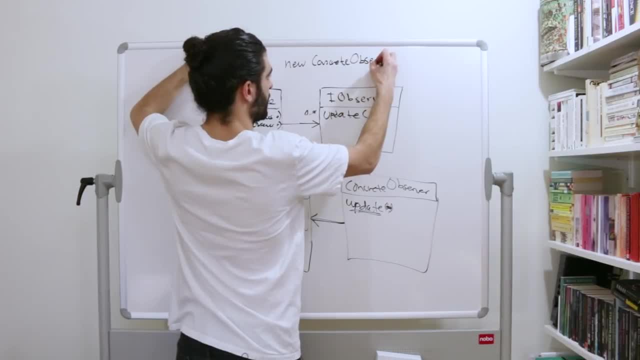 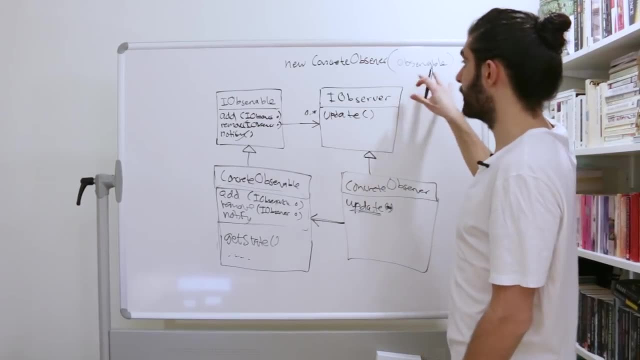 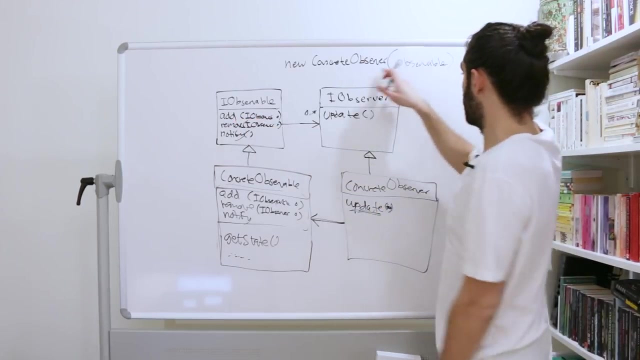 So when we're saying new concrete observer, we pass in an instance of the observable that we want to observe right. That's not registering us as an observer. That's not registering us right, Because registering happens through this method. But what this does is that it allows us to access. 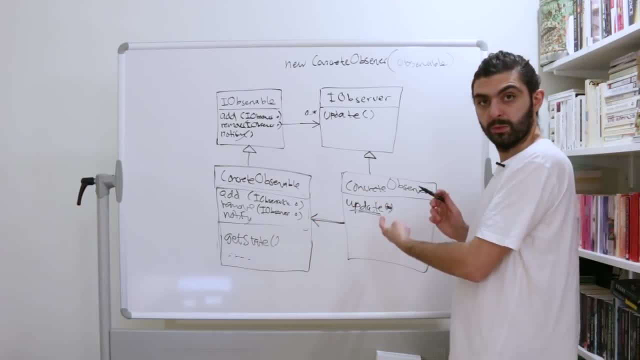 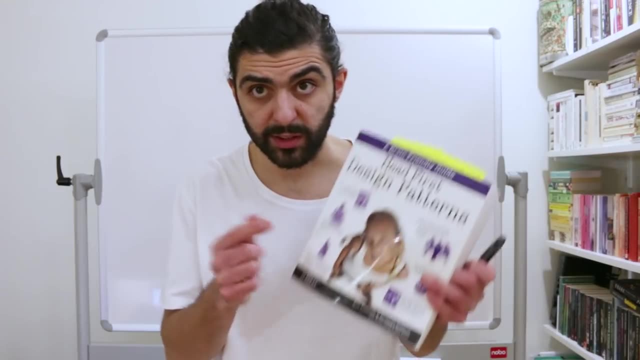 the concrete observer that has been updated. whenever we need to read the updated information, We'll get back to this. So let's flip this over and let's look at a concrete example. So I actually think that the example from the head first book is really good. 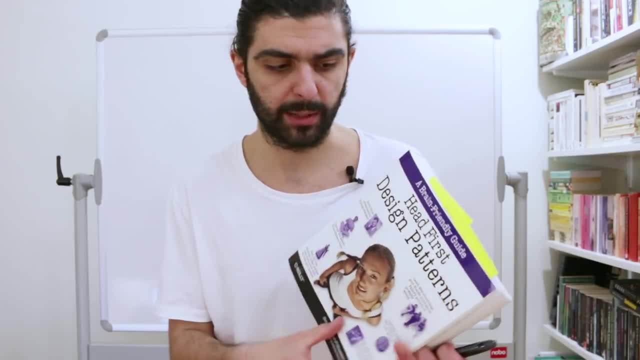 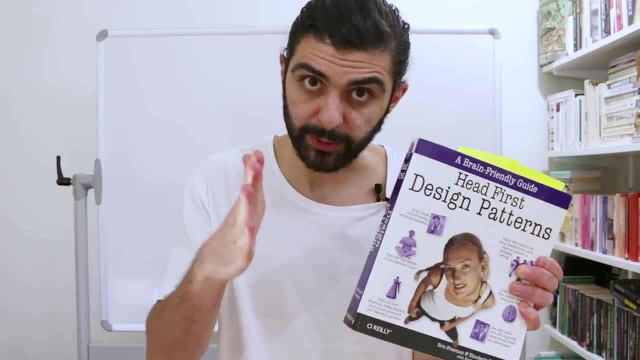 So we'll just strictly look at that example, perhaps with some minor adaptations. Let me just also briefly remind you that I'm always putting links to the books that I'm talking about in the description, So if you get the book, please feel free. 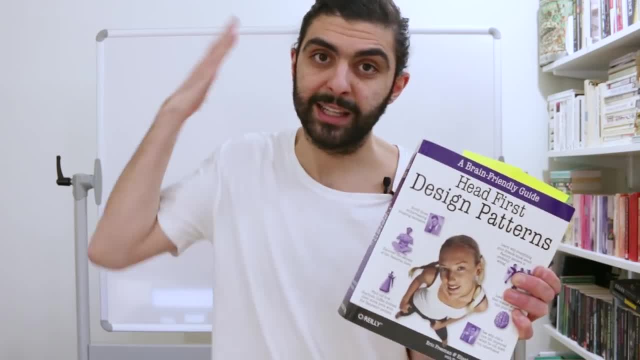 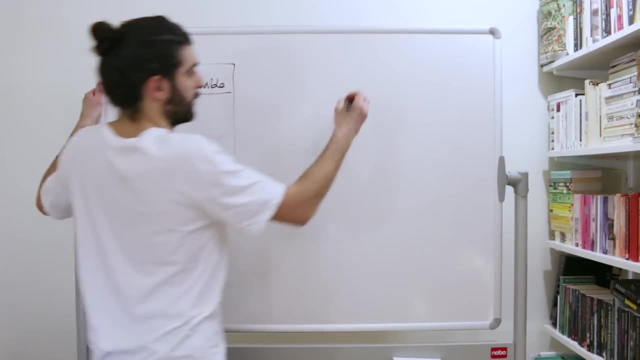 to use the affiliate link that I put in the description, because then I get a kickback and that helps massively Moving on. thank you very much. So let me start by quickly drawing back these two interfaces that we had. So we had IObservable and IObserver. 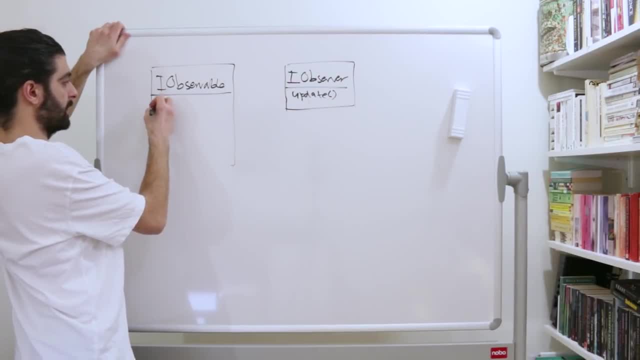 And observer has the method update and observable has the methods add, remove and notify. Add takes an IObserver and remove takes an IObserver. and notify takes no arguments. And that's it for the IObservable. Let's move to the concretions. 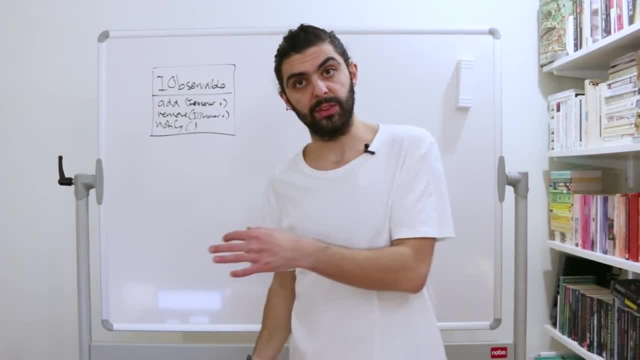 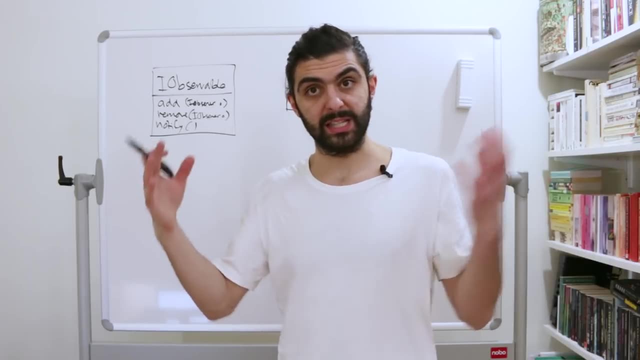 Now, before we move to the concretions, we have to understand the scenario. So the scenario that they're talking about is that they're saying, hypothetically, let's say, that you have some kind of weather station and this weather station receives updates. 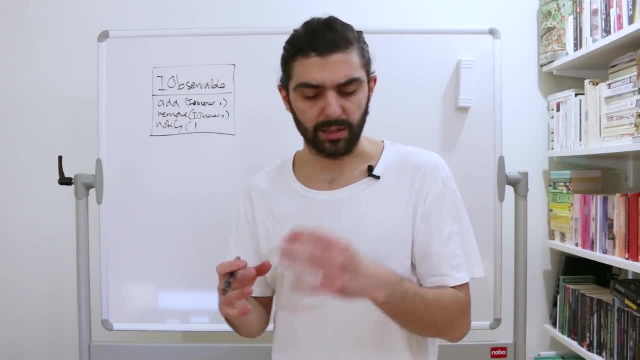 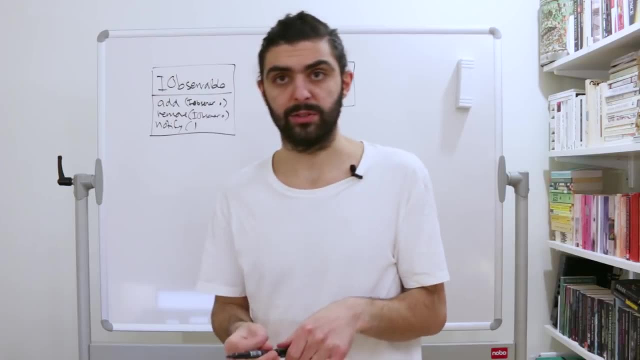 by sensors that they have in the. let's actually say that I mean, maybe it's a weather station that observes the weather. That's actually probably what it is, because they have temperature, humidity and pressure, So something like that. You have a weather station. it has sensors. 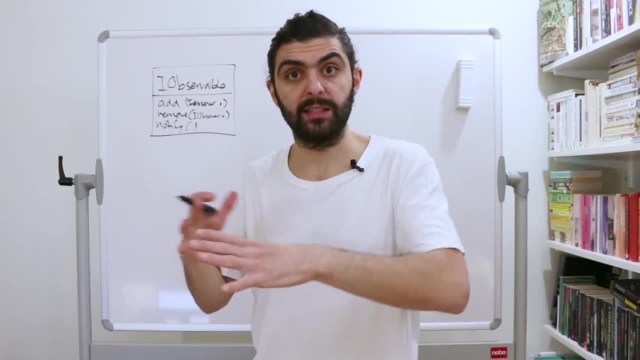 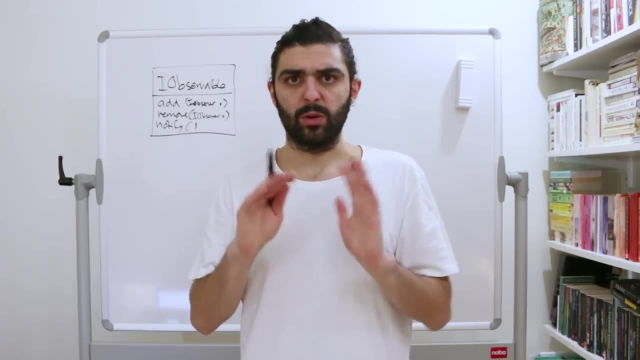 and it observes the environment And through observing the environment, it updates its own state of its measurements, So its temperature and its humidity, and et cetera. But let's again, let's keep it simple. So let's only talk about temperature. 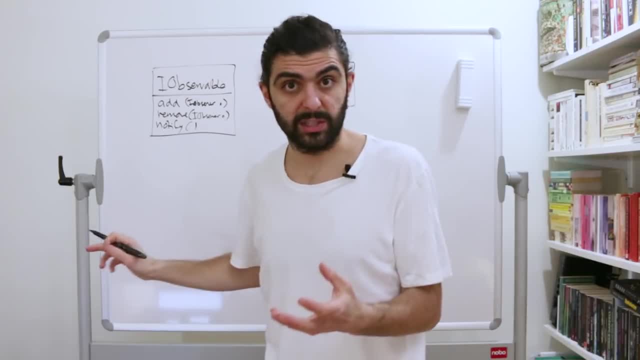 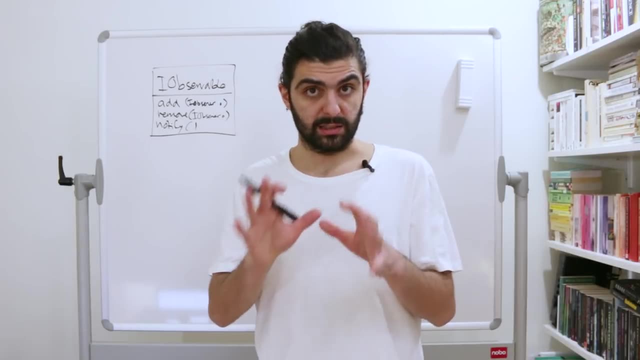 So essentially we need to have a weather station here, but the weather station in some sense is just a thermometer, But in order to stay consistent with the example in the book, let's call it weather station. So you have this weather station. 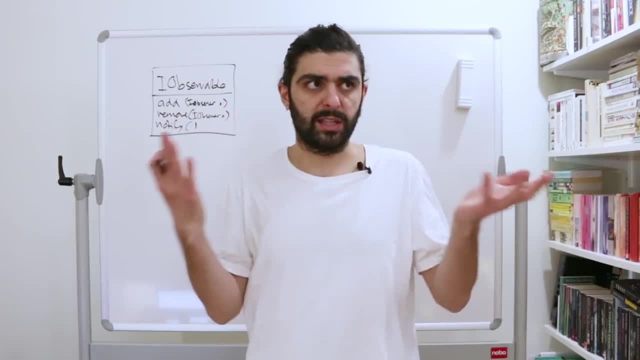 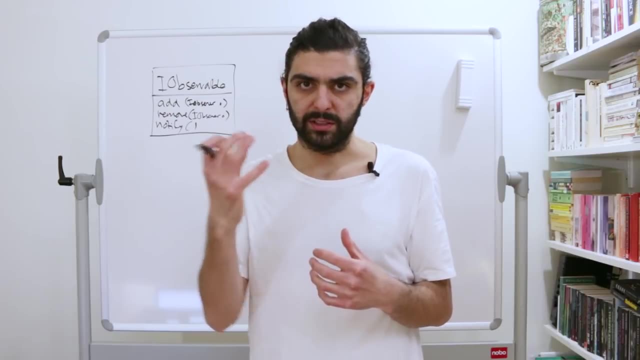 or actually, sorry, they call it weather data, but I'll call it weather station because I think it makes sense to think of it as the physical entity. It's the entity that collects data. So we have the weather station, but what do we want to do with this temperature data? 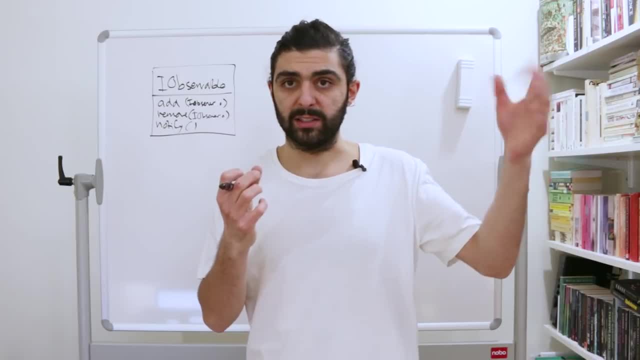 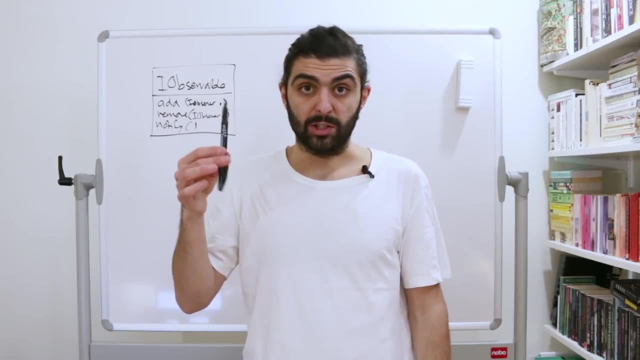 that we have in the weather station. Whenever it changes, we want to notify some other things. And what are these other things? These other things are displays, So that's not absurd, You could imagine. I mean say that you have the measurement station. 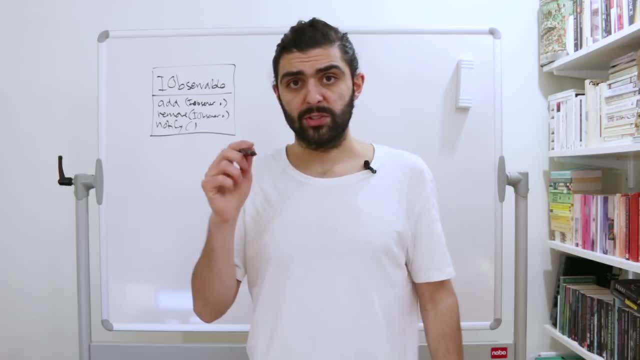 that measures your temperature. Just think about the room that you're currently in. Just imagine that you have some kind of sensor somewhere and that's the weather station. You have some sensor, but that sensor doesn't display anything. right? That just measures the temperature. 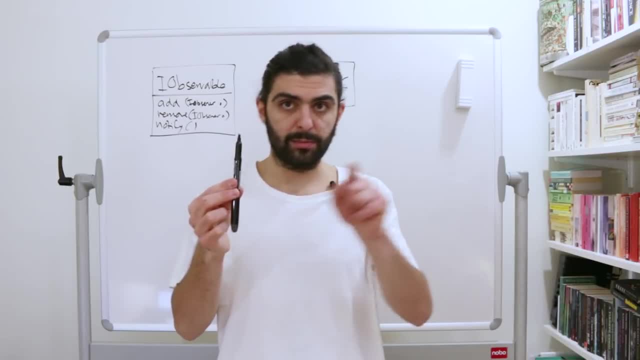 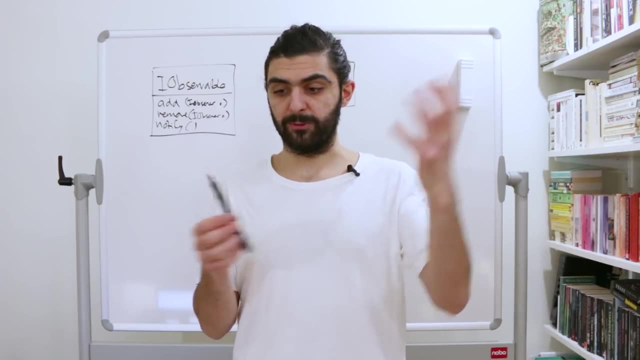 Whenever the temperature changes, it pings. It pings right. It sends a message to whoever you've registered as an observer. That might be your cell phone, for example. your smartphone Could be a physical display that you have next to your desk. 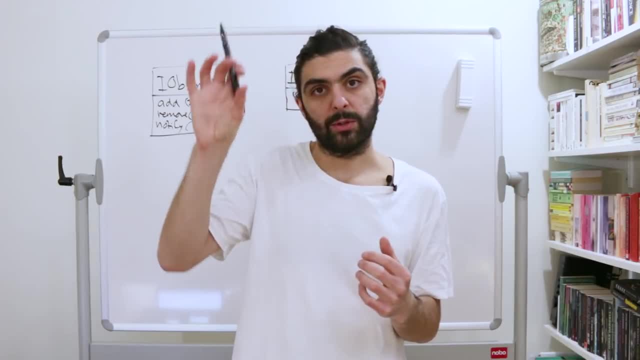 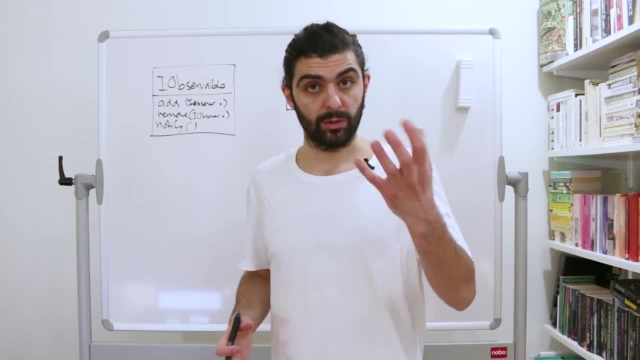 or wherever you're watching this, or a thing that you have in your window, or whatever, whatever. Essentially, the point is that you have a bunch of what the book calls displays. The display could be your cell phone or a physical display. 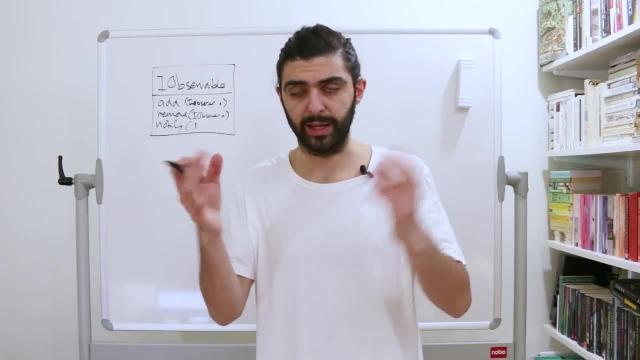 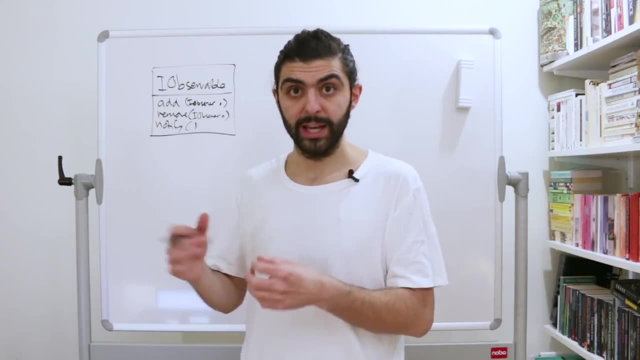 Let's just think about these two, right? Let's think of the smartphone and the physical display. So these two displays are the observers. They want to observe the observable, and the observable is the weather station. So let's draw this up. 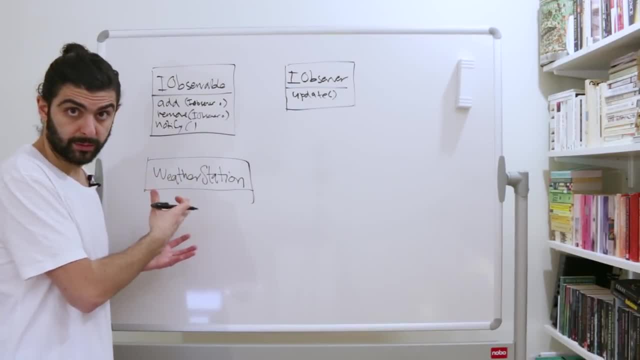 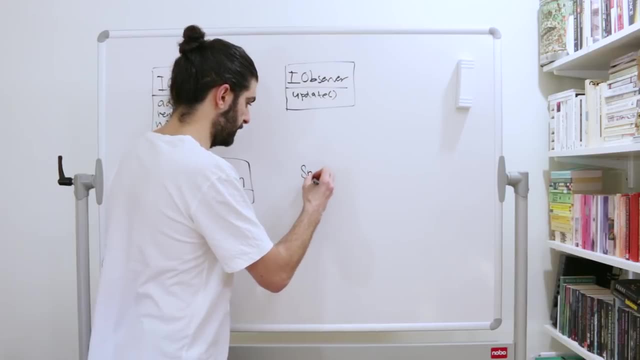 We have the weather station, which essentially is the glorified thermometer, It's the sensor, And then you have a bunch of displays. There could be many, but we'll stick to the two. So we have the smartphone- Actually, let me just say phone to save space. 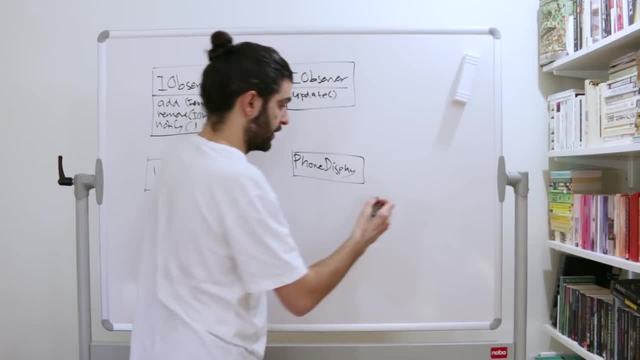 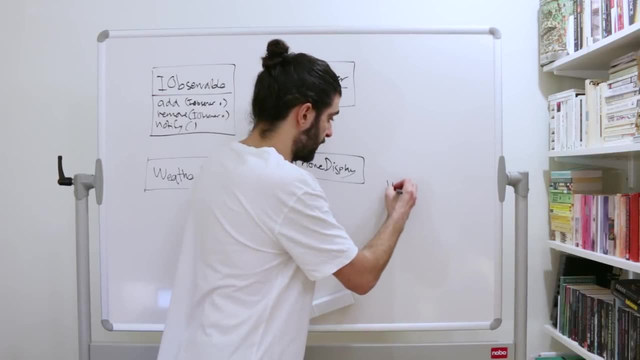 So we have the phone display and we have another one which is the physical display. Actually, a phone is physical as well, so that's kind of funny. Let's just say I mean, this is silly, sorry, but let's just say window display. 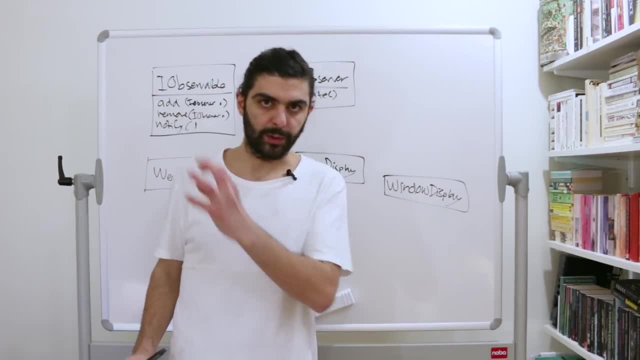 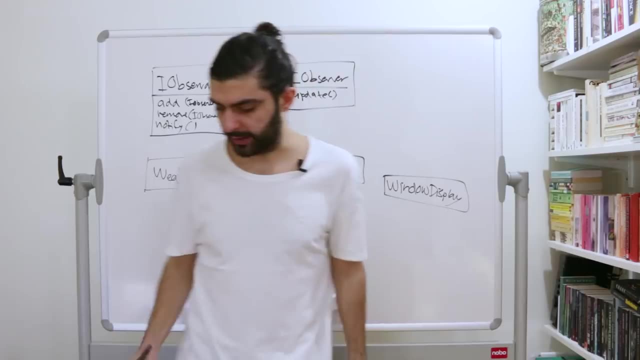 Perhaps we could have called it LCD display or something, essentially that you stick to the window right. So it's not a smart device like this, is This maybe has a lot of other functions? this doesn't I mean. this is just metaphorically, so it doesn't matter. 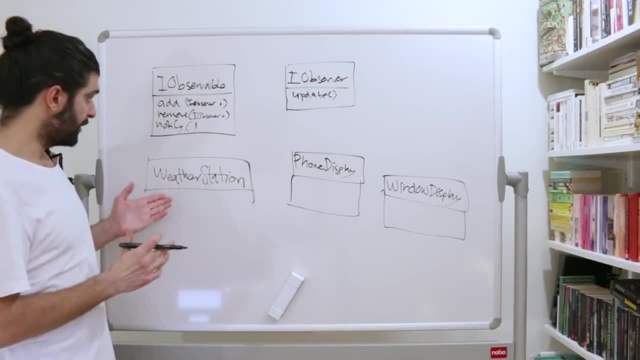 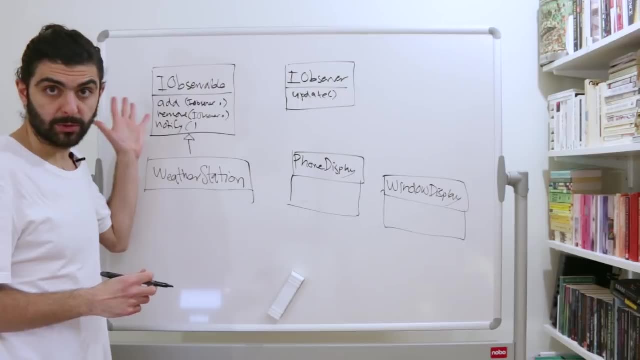 We have these two displays, So let's figure out the relationships now. The weather station, as we were saying before, is a observable or, because it's an interface, implements the iObservable interface. The weather station is an iObservable. The phone display and the window display. 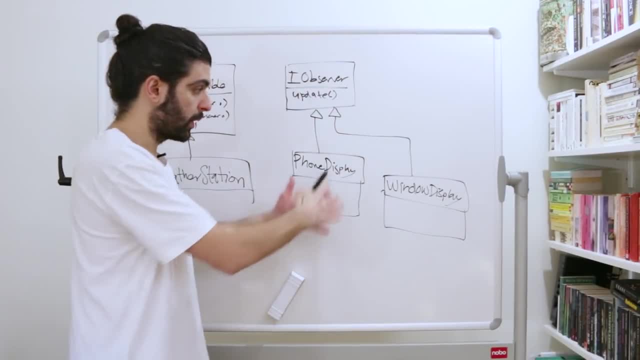 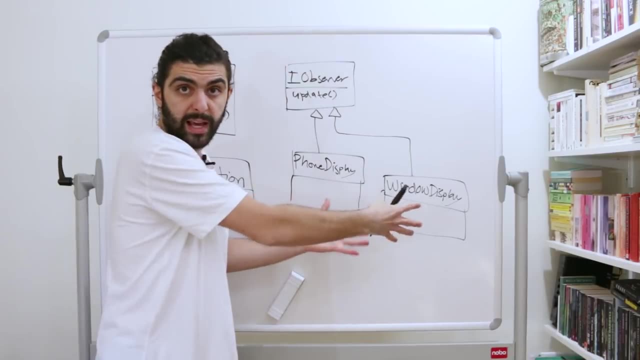 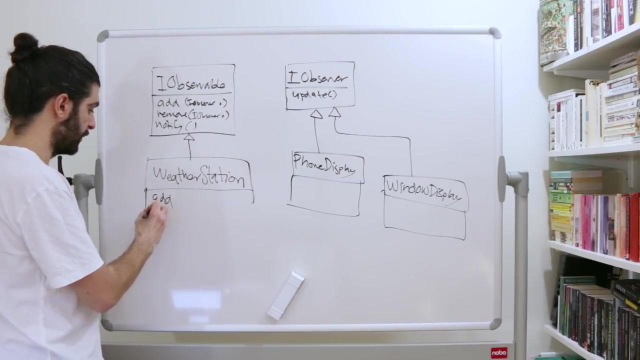 implement the observer interface. They are observers, They register to the observable weather station and when the weather station changes, these displays get notified. So that means that if weather station implements the iObservable, we need to add the add method, the remove method and the notify method. 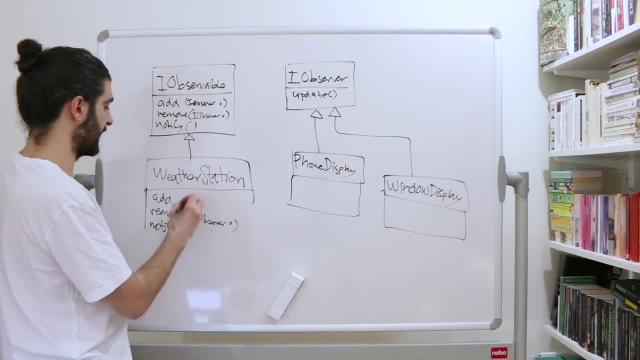 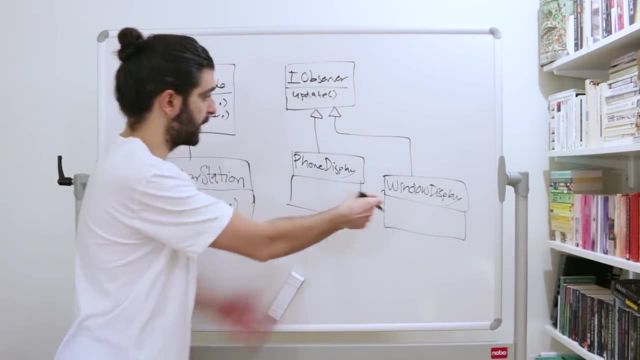 Notify doesn't take arguments. Remove. takes an iObserver and add: takes an iObserver. Pardon my sloppy handwriting, Whatever, and that's the weather station, But the weather station, the phone display and the window display implements the interface iObserver. 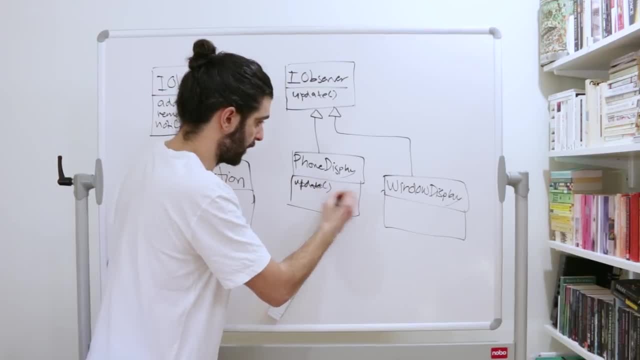 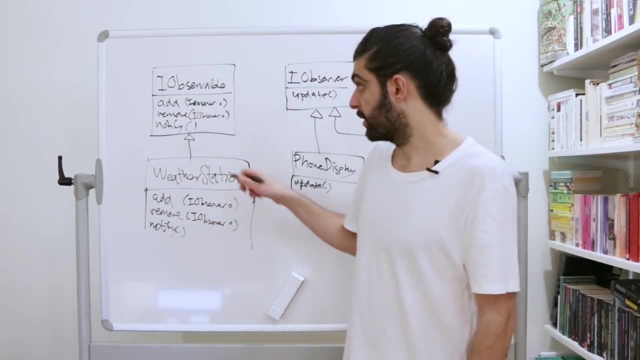 so that means that they need to have the update method. Update takes no arguments, Update takes no arguments And that's it. But recall from the example that we had on the other side of the board That when we talked about the concrete observable, 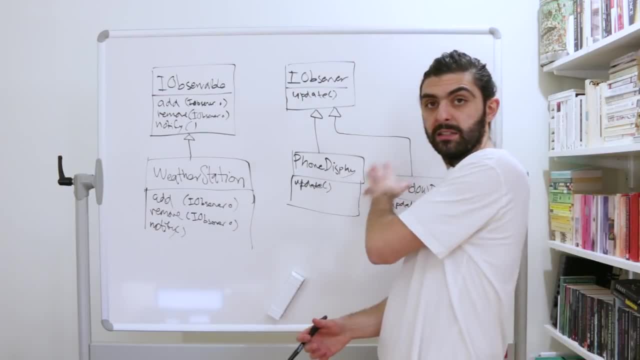 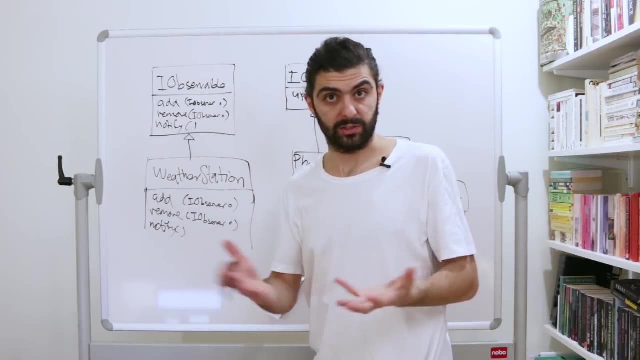 we talked about the method called getState. Somehow these guys need to be able to inspect the state of the weather station, of the observable, to see what its current state is. And here we actually. that's why I was saying, that's why I was saying: 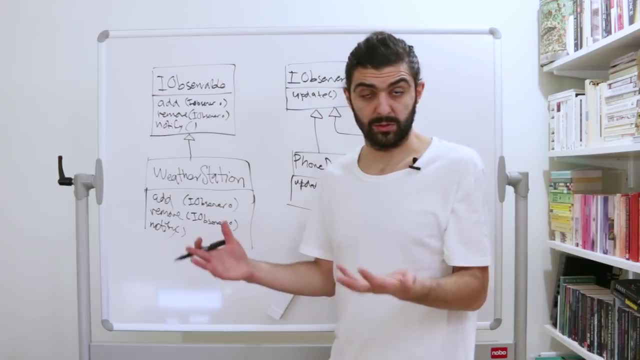 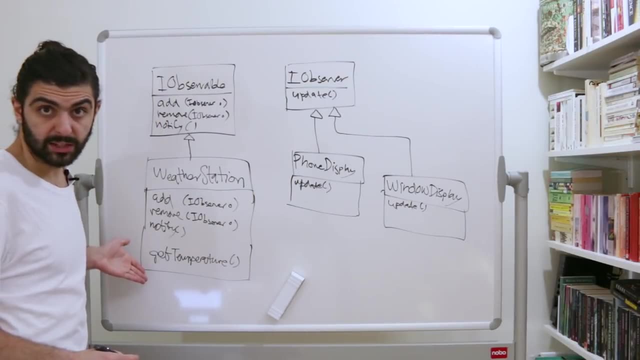 it's a placeholder, because it's a concrete weather station. it makes no sense to say getData. If we're interested in temperature, we could just say getTemperature. So that's a method on the weather station. So in other words, whoever has access to an instance of a weather station? 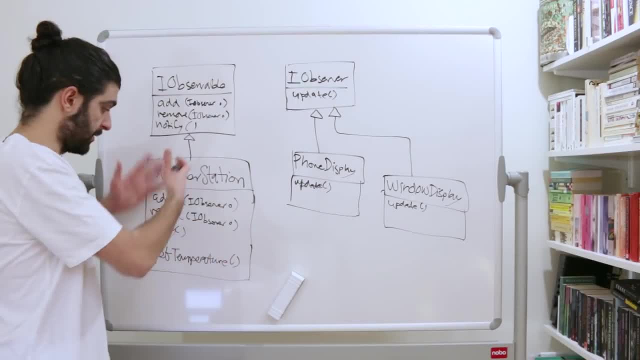 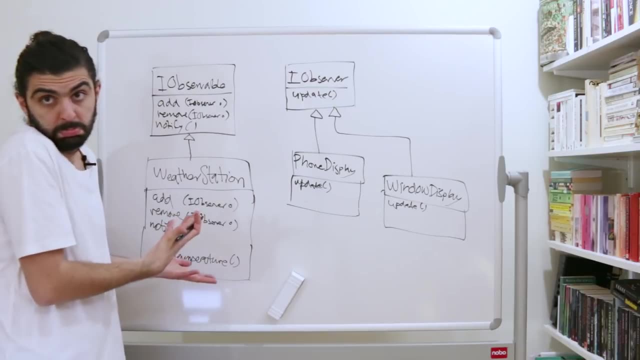 can ask the weather station what its temperature is. It's a thermometer, it's a sensor and you can ask the sensor what's your latest reading for the temperature? right now Makes sense, And again. then they have some more cruft. 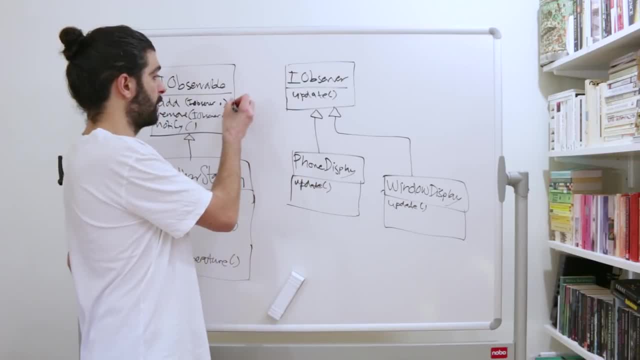 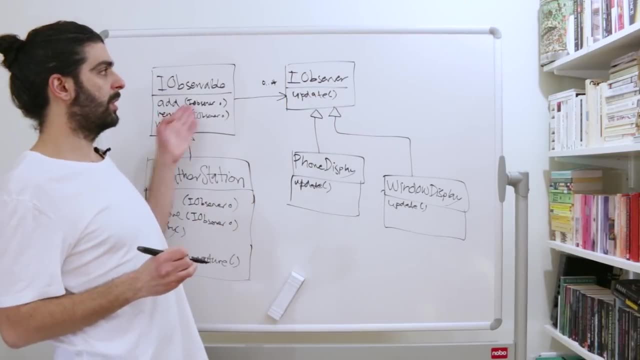 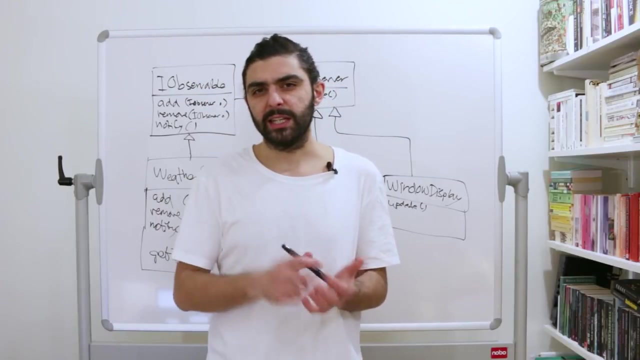 but we'll skip that. And, of course, what we forgot is that the observable needs to have hasObserver, and this is zero to many. An observable has zero to many observers. You can have many observers observing the observable, And while this isn't really necessary, 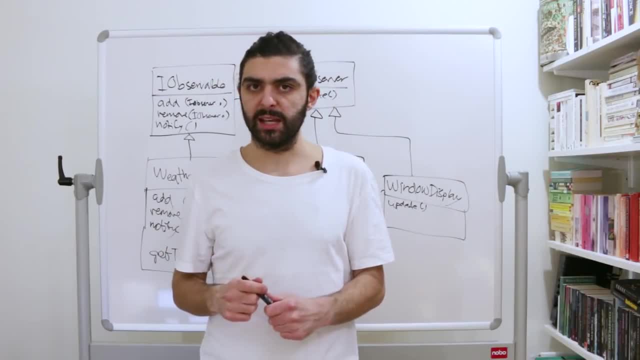 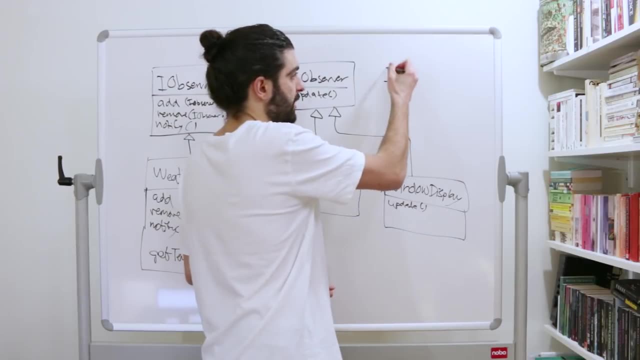 to show the sort of structure of the pattern. what they put in in this example is another interface, and that actually makes a lot of sense if you want to make the program actually do anything useful. So what they have is that they have an interface. 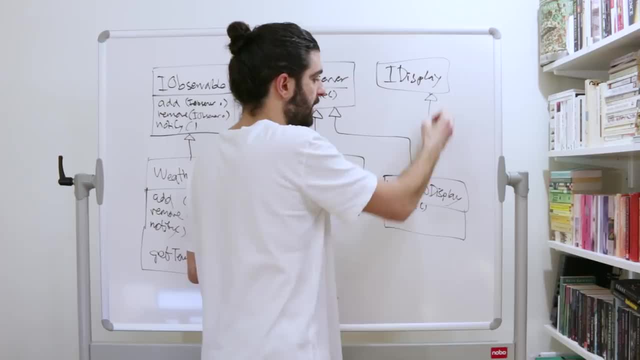 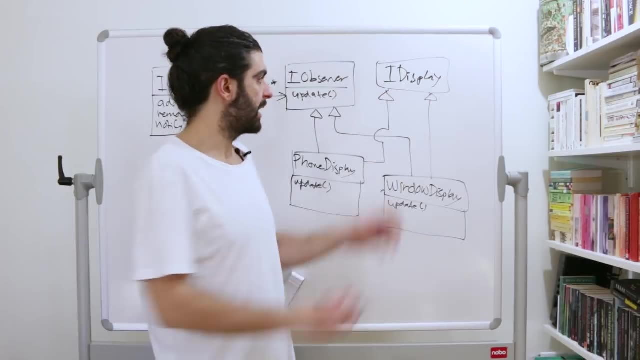 called IDisplay and essentially these two- these two displays- implement the IDisplay interface. Sorry for the jumping arrow here, But again, this doesn't matter in terms of the observer pattern. It's just that this is a way they're doing it. 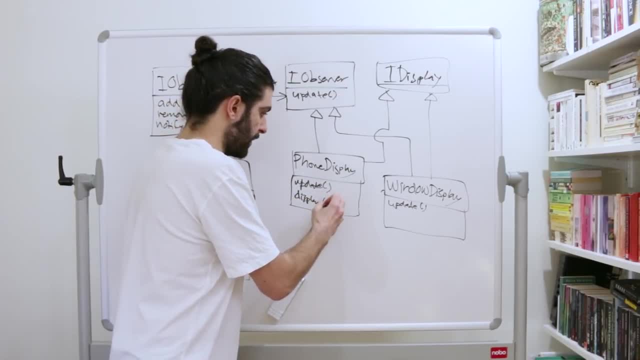 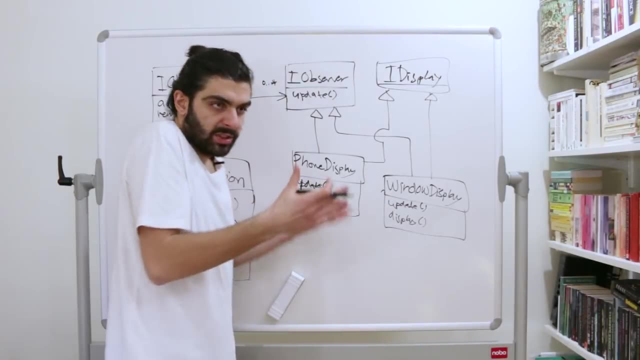 to say that these displays actually should have a display method as well. So when you call update on these, the internals of the displays are changed, but you're not actually displaying anything. So you have to call display on these particular displays in order to actually display anything. 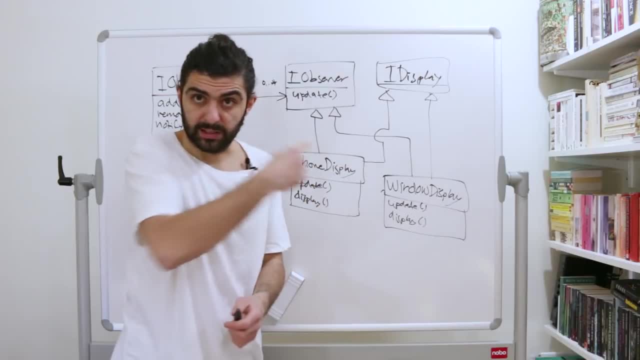 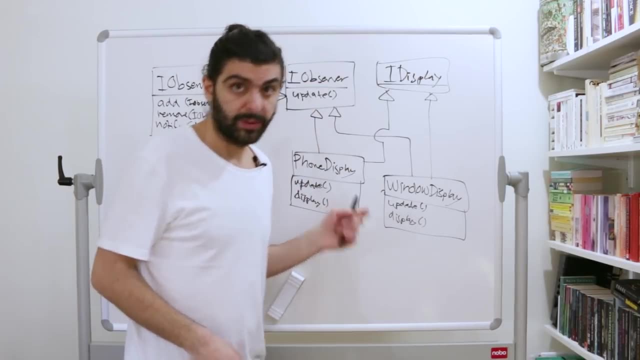 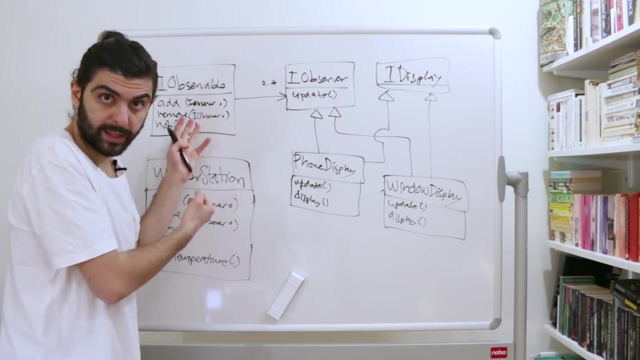 Again, not necessary for the pattern, But what's interesting with this is perhaps the reflection that this was possible because we used interfaces rather than inheritance. Remember we said before that IObservable, we could have constructed that as an abstract class and then inherit from that. 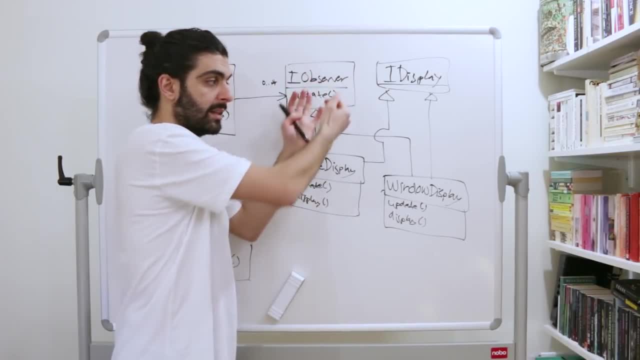 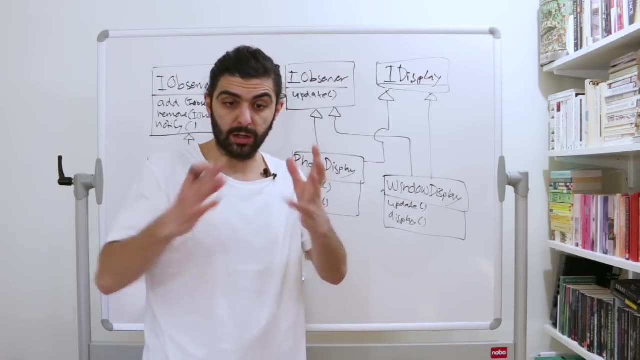 And we could have done the same thing with IObserver. We could make that an abstract class and then inherit from that. But if we inherited from that, you know, remember right, when you don't have multiple inheritance, you only have one space for inheritance. 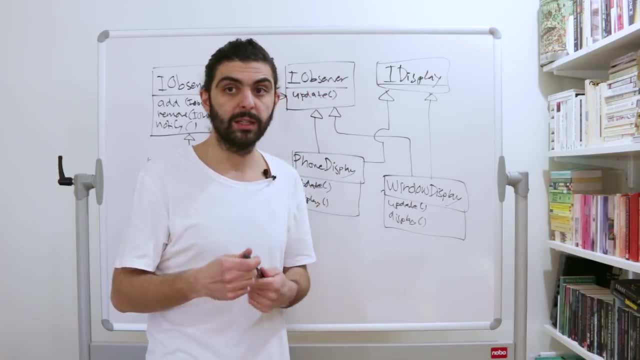 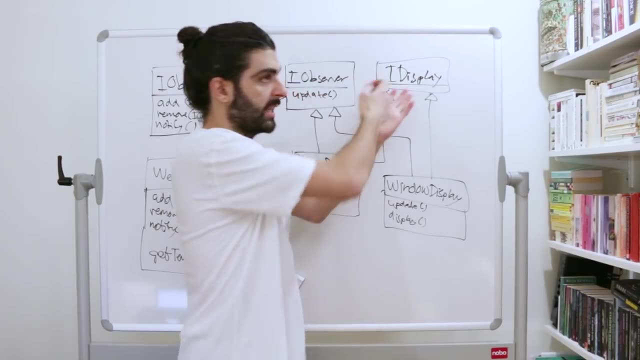 A child can only have one single parent in object-oriented programming. But when you're using interfaces, you can implement multiple interfaces. So the display can implement the IObserver interface, but it can also implement the IDisplay interface and another interface. and another interface if you want to. 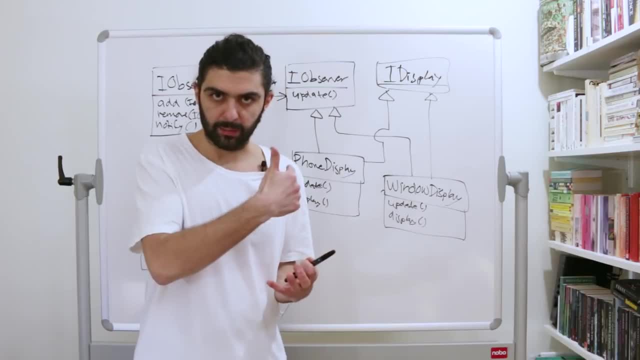 But that's that about that. So if you start to look at this, take a step back and think about this, it's sort of kind of starting to string together right. Let's think about the flow of the program. How would this work? 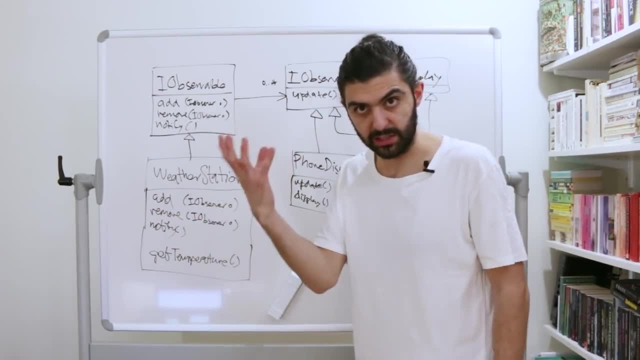 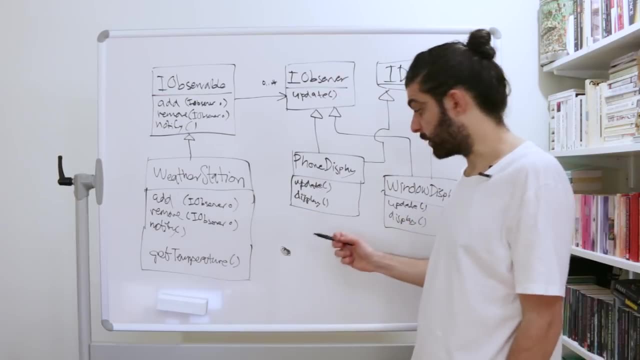 You would do what You would instantiate a weather station. You have an instance of a weather station. okay, It is an observable, so that means it can be observed. So you have the weather station. Then you take the weather station and then you say: okay, 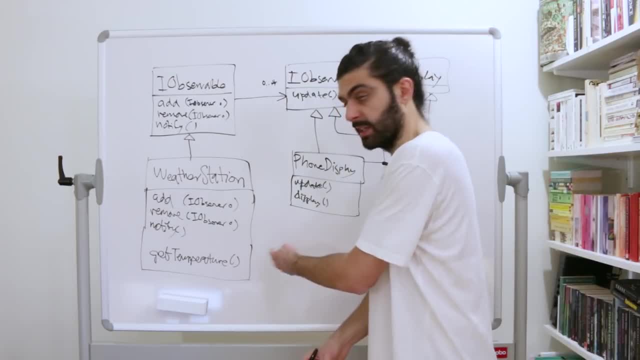 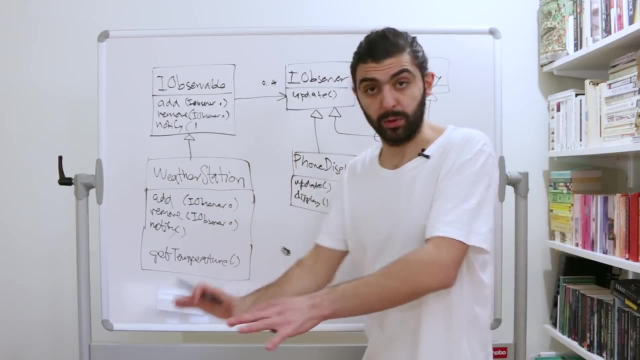 I want to have some displays that are notified whenever the measurements in this weather station change. Of course we haven't talked about how the measurements in this thing changes, right? That's outside the scope of this diagram. The book gives an example. 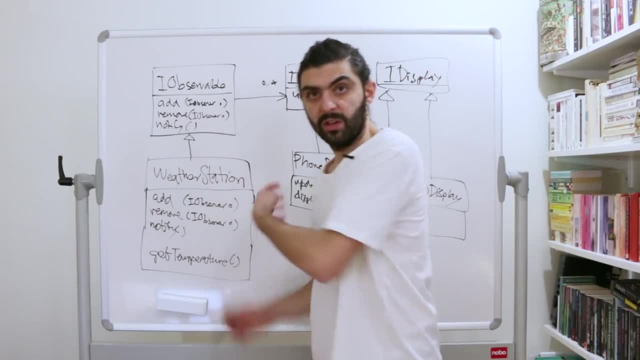 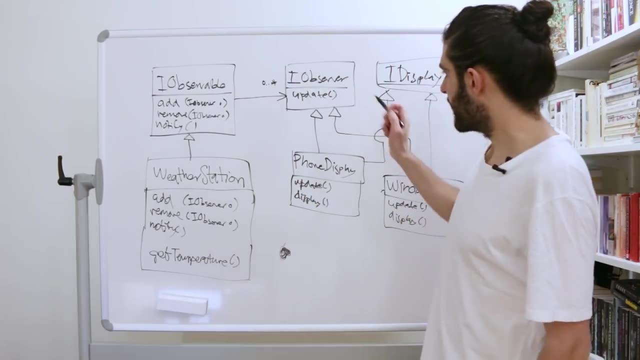 but let's just not make it too complicated, right? You can just imagine that somehow the state of this thing changes. But you have this weather station, right, This single weather station, this single observable, And then you instantiate a bunch of observers. 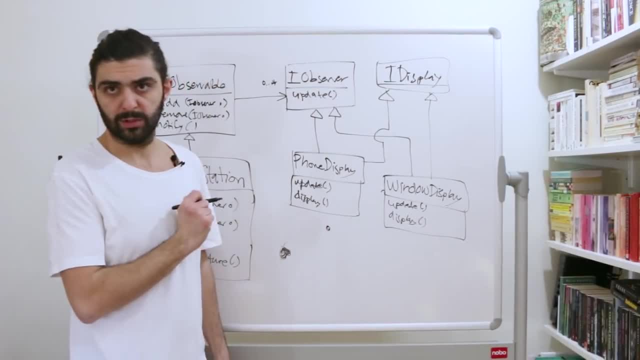 So you instantiate a bunch of observers. You say: okay, let me have the phone display, Here's the phone display. And actually, because this is a class, let me have phone display A and let me have phone display B. right, 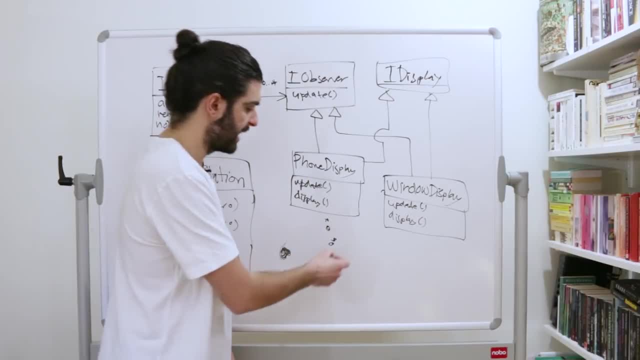 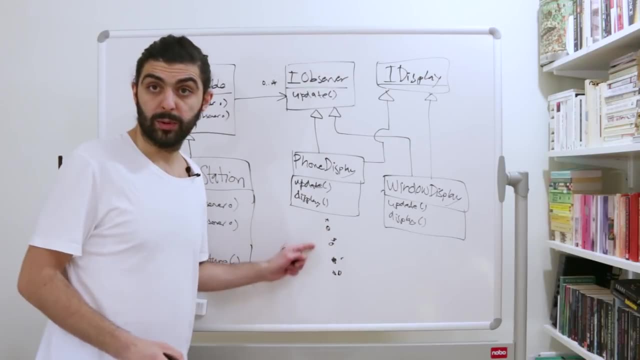 It's my phone and it's your phone. So these are two observers, And then I have a window display for the kitchen window and office window and da-da-da-da-da, right. So observer A, B, C and D, So a bunch of observers, right. 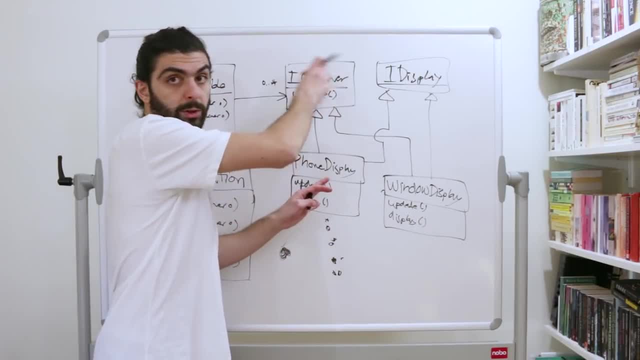 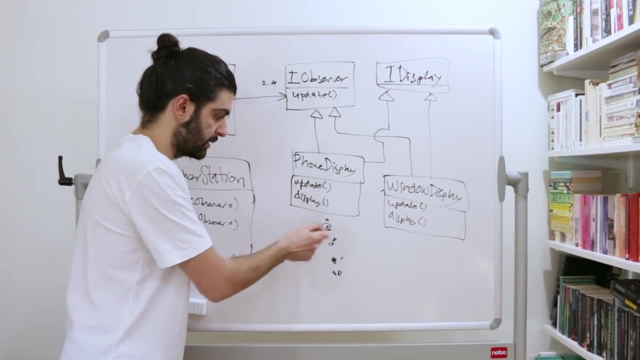 It doesn't matter what type, they are right, Because they are eye observers. And what you do is then that we call add, we call add on the weather station and we pass all of these. So we call add with this one. 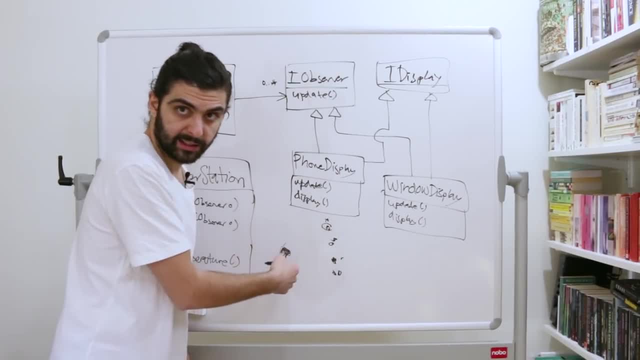 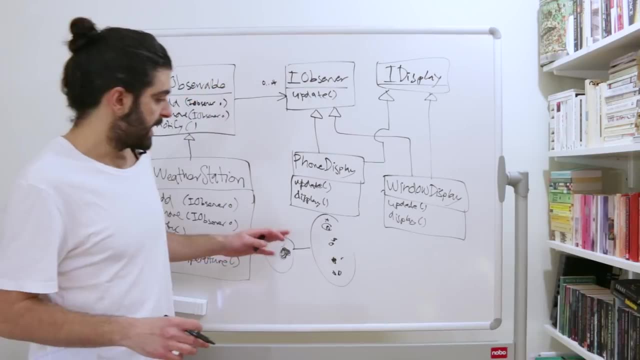 shoop, add it in. We call this one, add it in. And we call with this one and add it in. So then, the weather station now has some kind of collection and the collection contains all of these. Now, what I didn't say is that when we instantiated these, 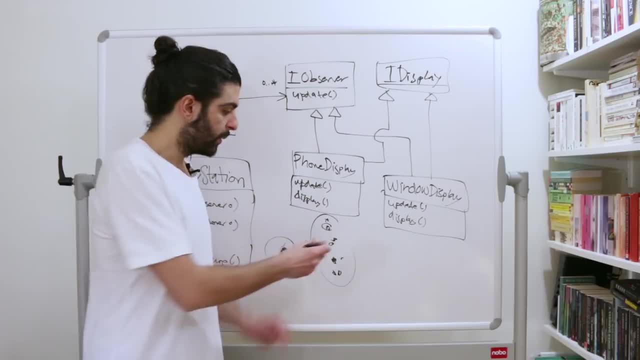 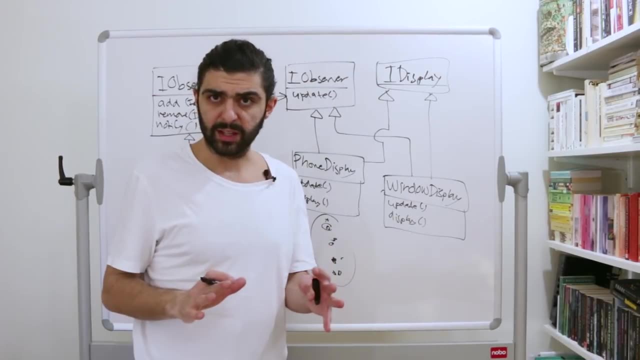 we talked about this briefly before. when we instantiate these, we need to also pass a reference to this guy, So the observers need to know about the observable. So actually I think it makes sense to start to look at actual code. So hopefully we can figure out. 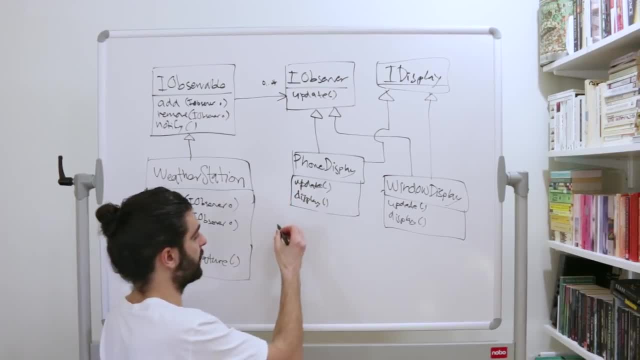 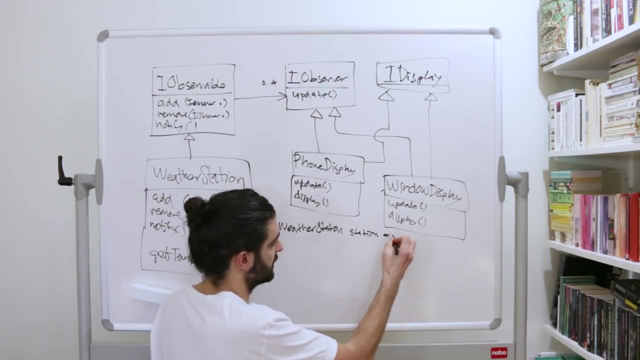 how to fit in this space. I'll try. So we start, let's redo the same thing. We instantiate the weather station. Weather station, let me just call it station. variable name is a new weather, my God room station. 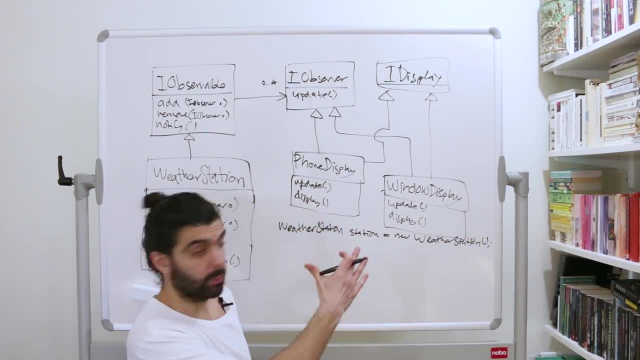 So we have a weather station called station, that's a new weather station. Then what? Then we instantiate a display. So let's instantiate a phone display. I'll only do one display, but I think you can generalize and figure out how it works for the other displays. 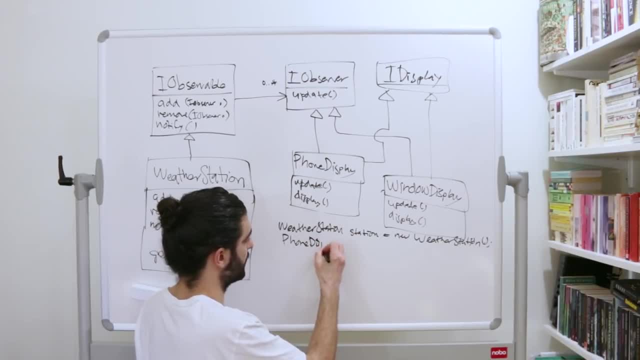 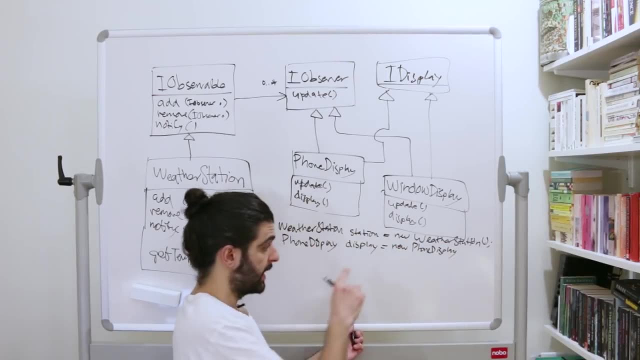 So let's say we have a phone display, So we instantiate a phone display. Phone display, let's call it just display, and it's equal to a new phone display. And here's the kicker: it's a phone display, but in the constructor we pass what? 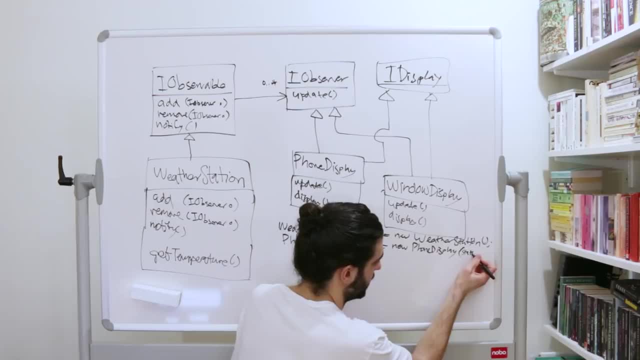 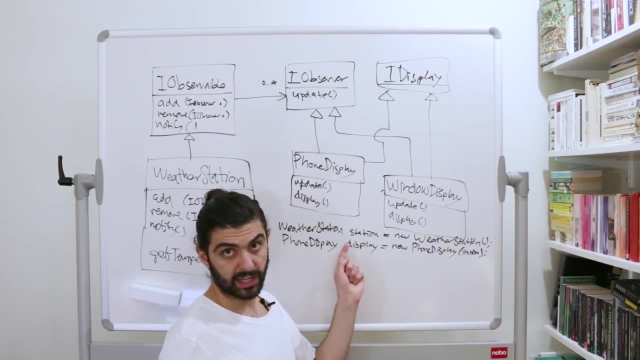 We pass the station, So super tiny station, So we instantiate a phone display and in the constructor we pass an instance of a weather station. And we're doing that, remember, we're doing that because the display somehow must be able to. 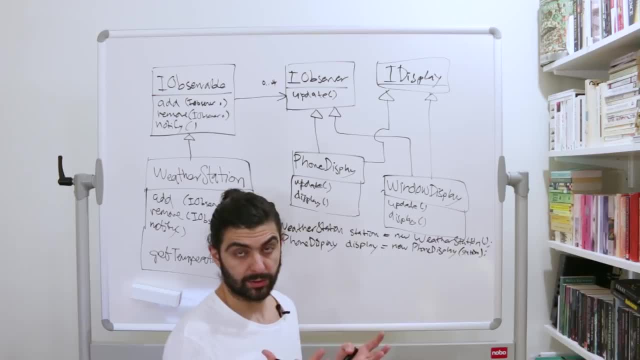 look at the weather station and figure out what the current state of the weather station is, Not because it's pulling, not because it's asking whether the state has changed- That's what we're solving with observer pattern- But because, when it knows that the state has changed, 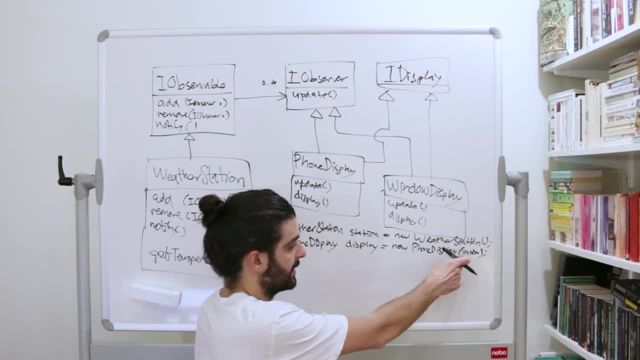 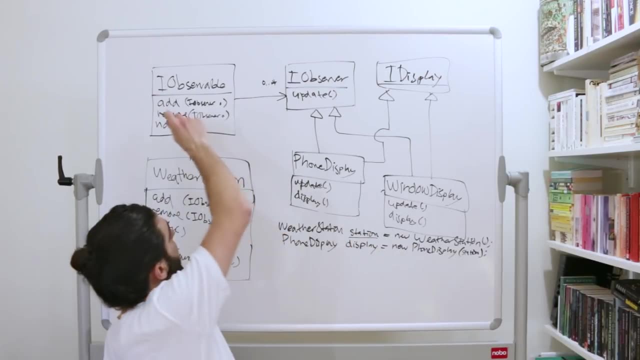 it needs to somehow access the new data, And this is why we're passing it in. Then we do what? Then? we need to make use of observer pattern, We need to take the station variable and we need to use the add method. 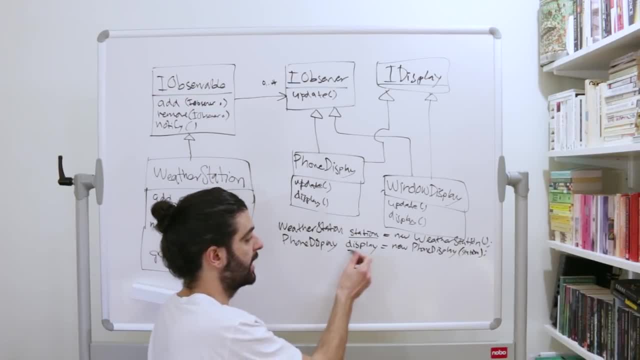 because it's an observable right. It has the add methods. We need to add this display right. So that's what we'll do. We'll say stationadd and we pass in the display. Super simple That means, if we have the correct implementation. 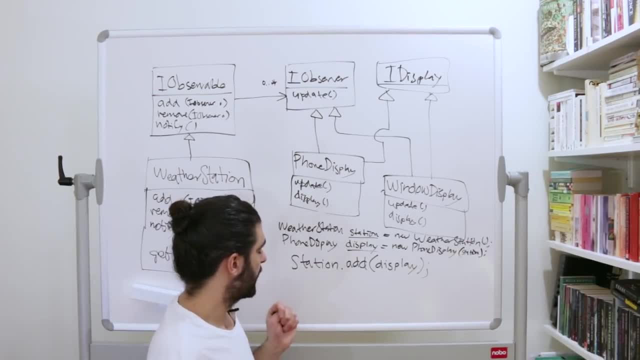 of notify, of course, but that means that whenever notify is called, this display will be notified via the update method of the fact that the station has changed. And then we could go on. We could say: stationadd another display, stationadd another display. 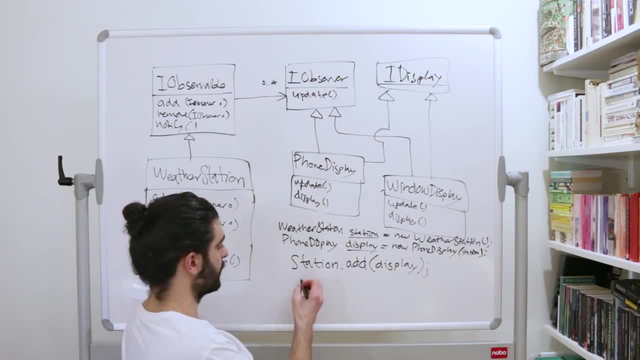 stationadd, another display, et cetera, et cetera, et cetera. And then again we would say we could say stationnotify, and then all of the observers would be notified. Of course you could argue that notify should happen. 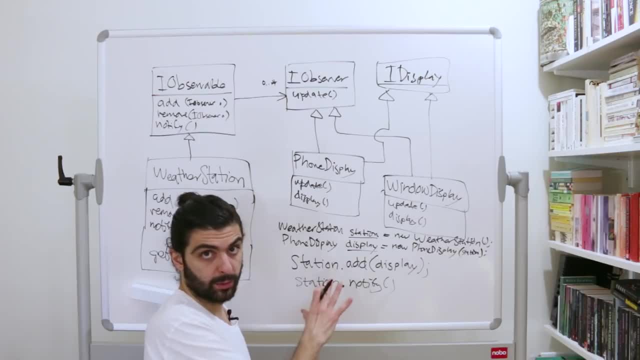 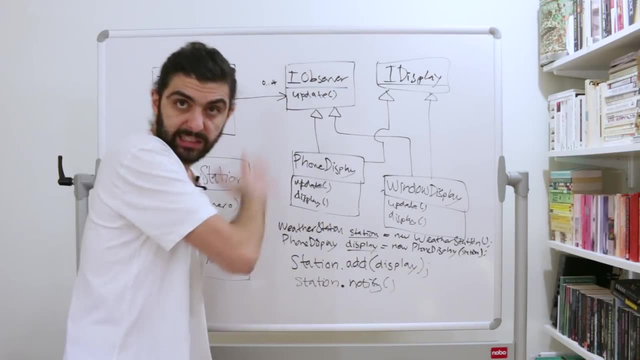 within the station rather than from the outside, but let's not worry about that right now. So that's how we would use that. Let's super quickly look at a short code example that does exactly what we've done here. We'll remove the display interface and the display methods. 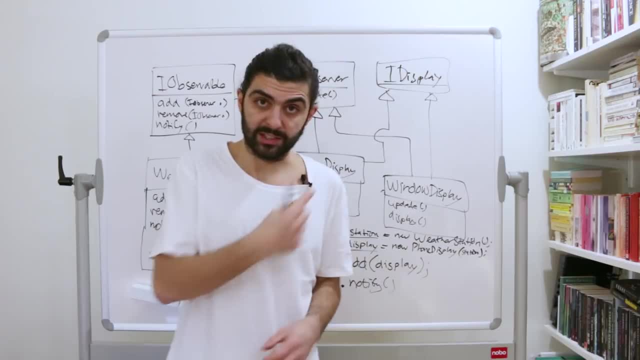 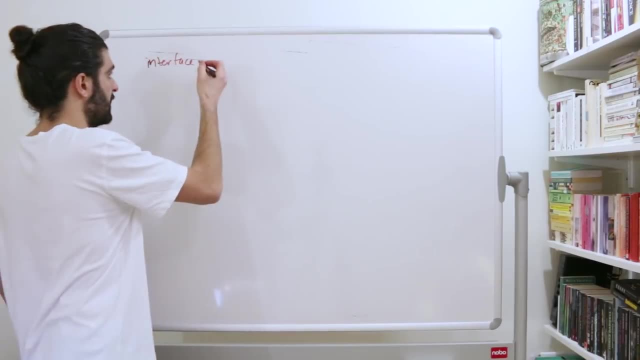 just to sort of keep things small so that we can actually fit on this whiteboard. But let's jump into the code. So let's start off with the interfaces. So we've got an interface, So I'm using C-sharp-like syntax. 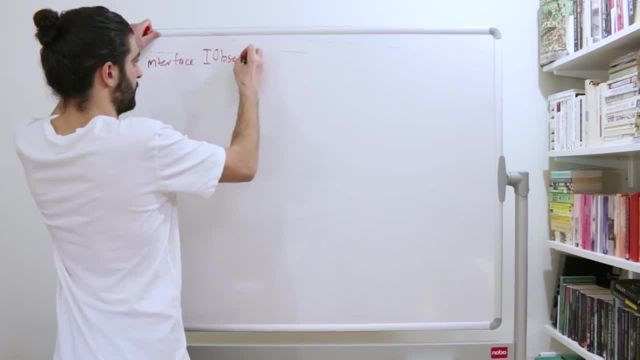 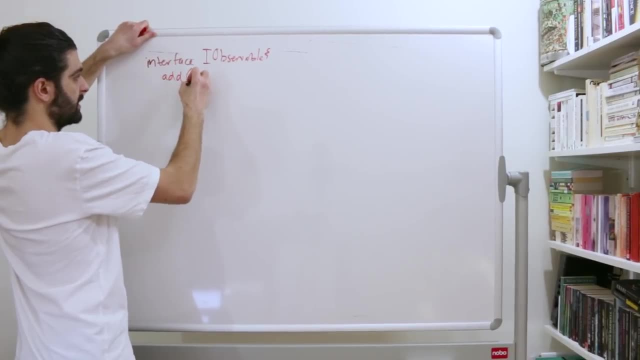 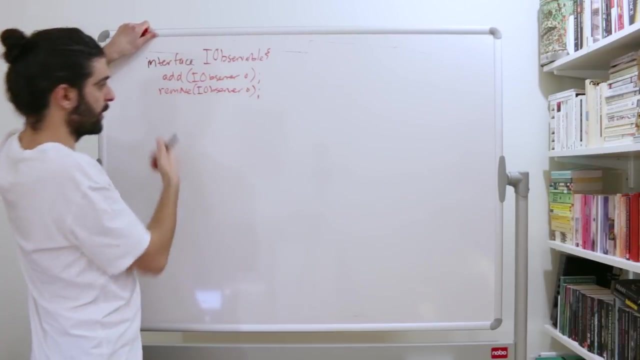 So we've got an interface called iObservable or subject in the book, And it essentially just states that you need to have the add method, which takes an iObserver, and you need to have the remove method that takes an iObserver, And depending on your scenario, of course, 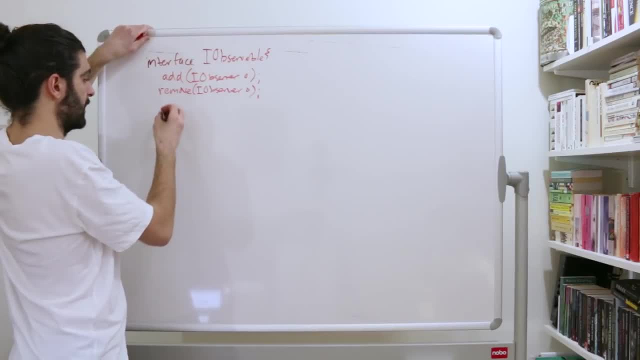 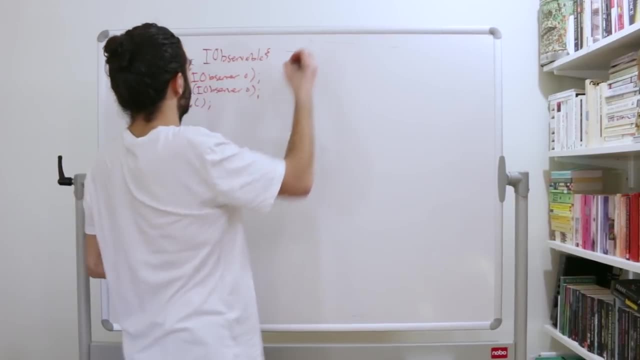 you might not even need the remove method. We're just trying to be exhaustive here- And then you need the notify method And that takes no arguments. That's the interface- iObservable- And then you need to have another interface, Interface for the observer. 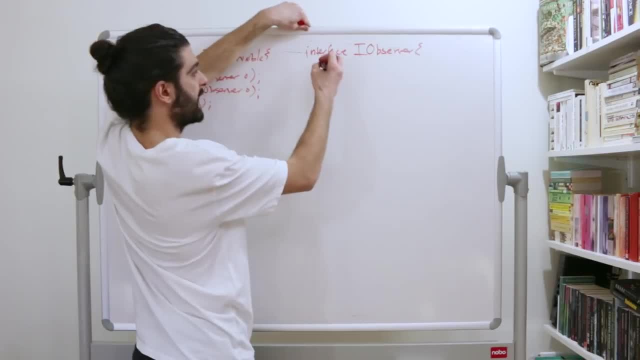 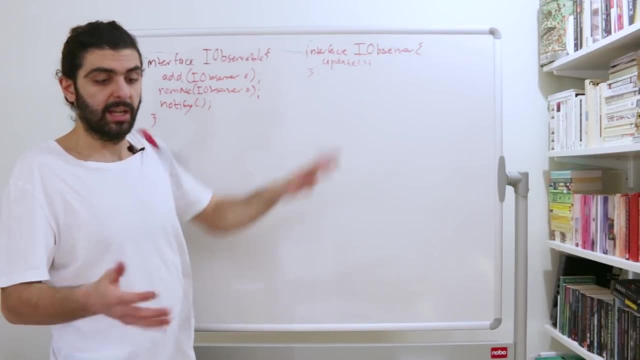 So we used to call that the iObserver, And that thing essentially just has an update method. So we have the iObservable interface and we have the iObserver interface. Then we had what? Then we had the weather station and we had the two displays. 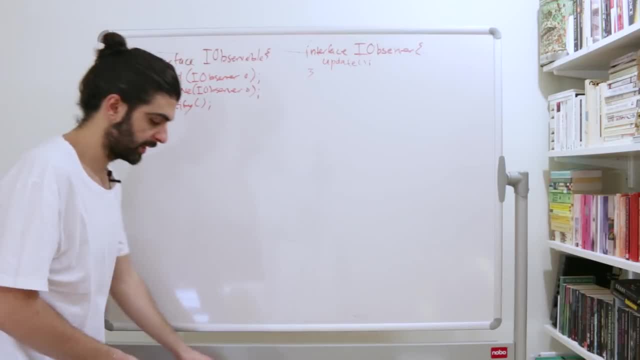 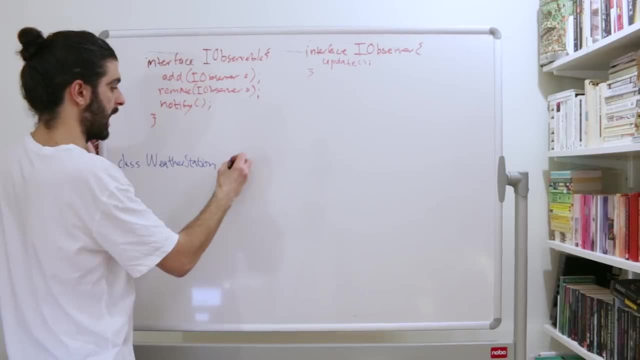 So let's first build the weather station. The weather station implements the iObservable interface, So let me switch colors. So we have a class called the weather station And it implements iObservable. It implements the interface iObservable, And we'll add those methods. 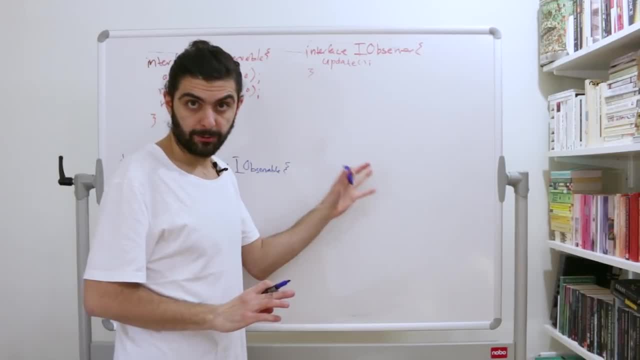 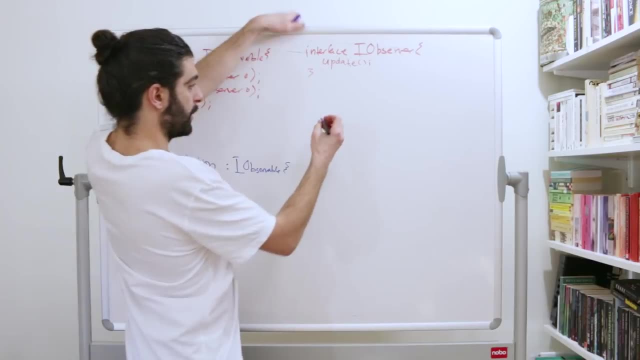 but let's first do the next class. So let's only do the phone display, And then I think you can figure out that the window display or whatever other display you want to produce, is essentially the same thing. So then we would have another class. 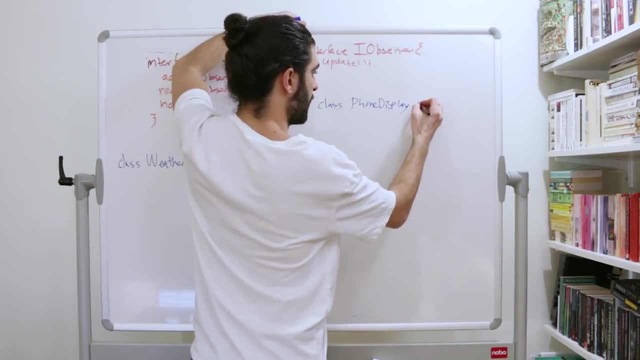 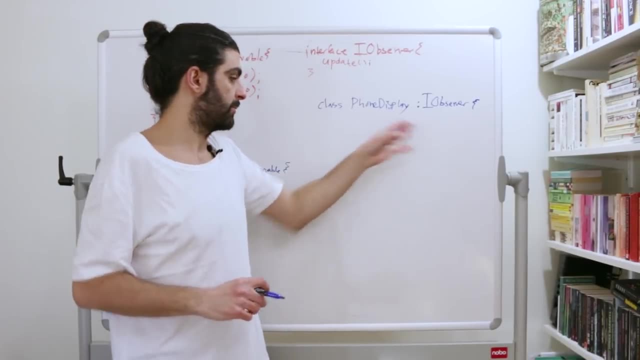 a class called a phone display, which implements iObserver. And again, here you can add multiple interfaces because, as we were saying before, in their example they also implement iDisplay. So let's start with the implementation of the weather station. 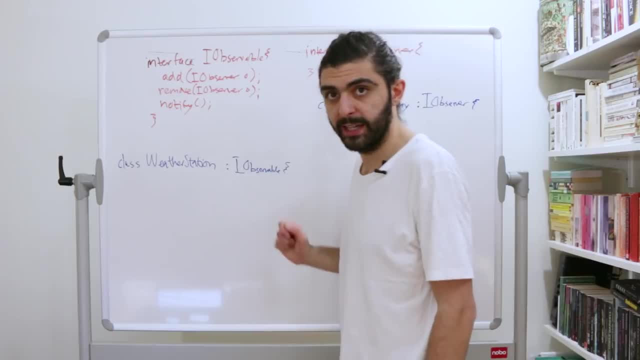 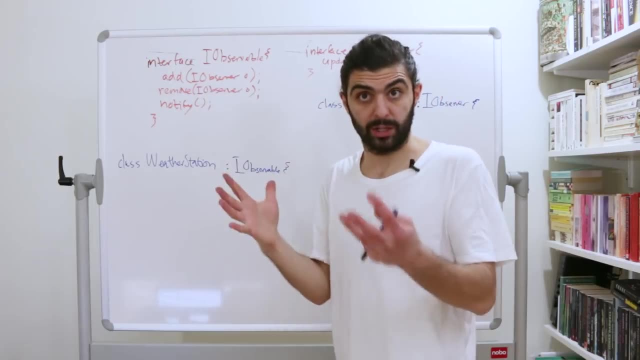 The weather station needs to do: add, remove, notify And, as we saw before, we also have the get temperature method. that's specific to the weather station and has nothing to do with observables in general, So I'm probably not gonna be able to fit this. 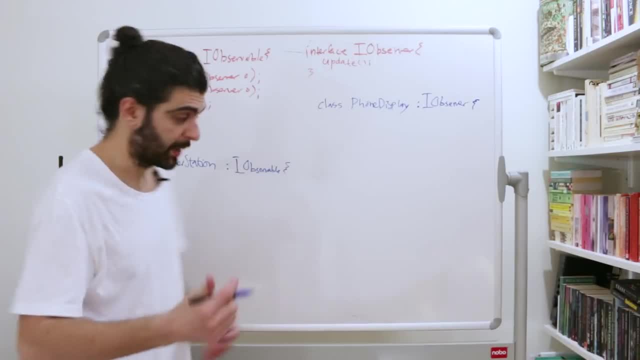 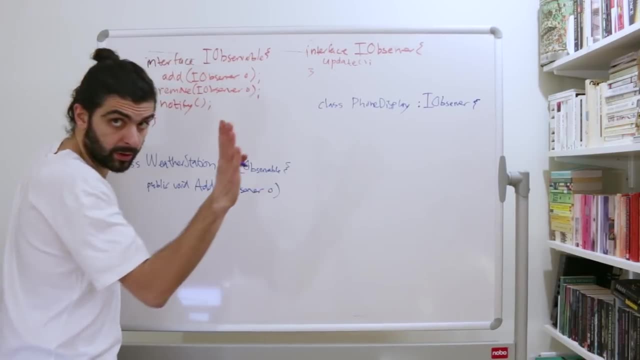 on the whiteboard. So I'll have to use some heavy pseudo code. So hang with me. It's really simple actually. So the add method- let's say public void add- takes an iObserver. let's call it O, sorry. 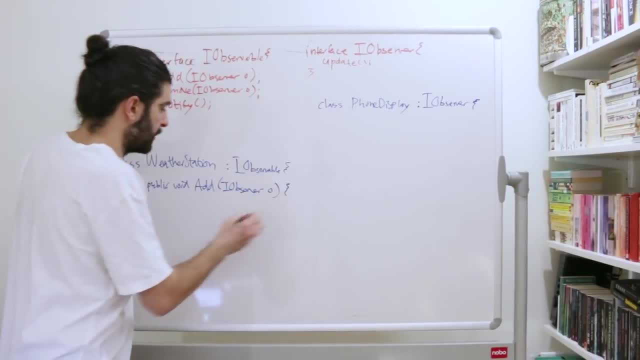 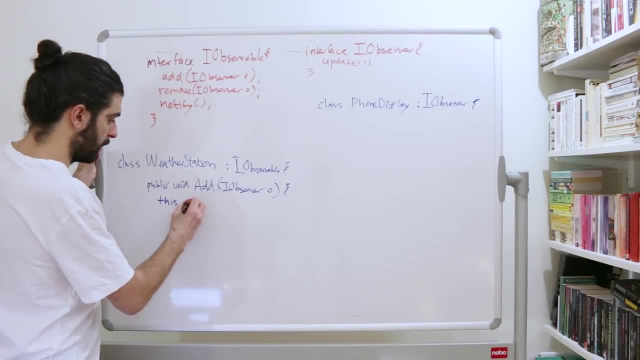 bad variable names. Never do bad variable names. This is just for the example, And the implementation of that method is that we add it to some list that we have in this class. So let's say that we have a list. We say thisobservers right. 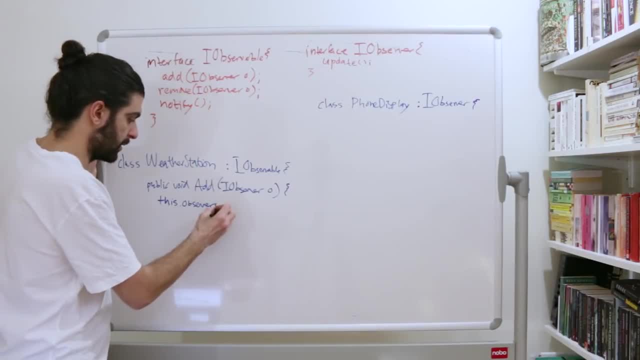 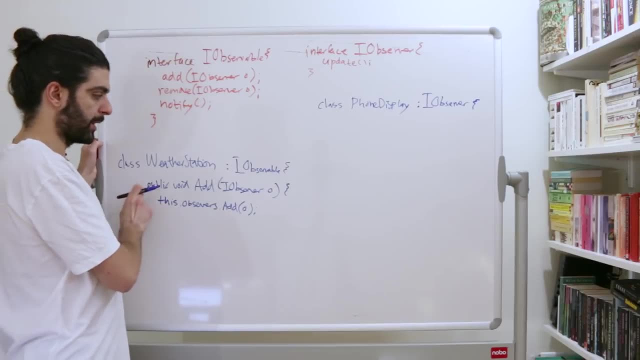 Let's imagine in this class I have a list of observers, Thisobserversadd- and I add this O that it was passed in right. So the weather station has a method called add and the method add gets an argument When you call the method add. 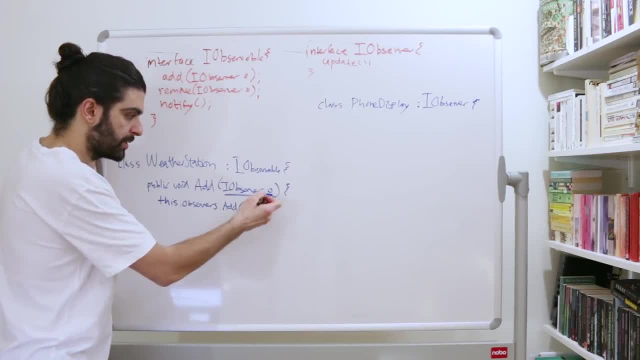 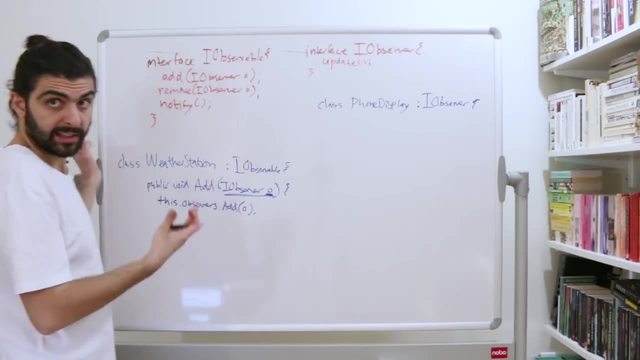 you call it with an argument and that argument is an observer and that observer instance, that observer object. you then add to a list that you have inside of this class of observers And that's how we keep track of the observers And that's how the observable keeps track of the observers. 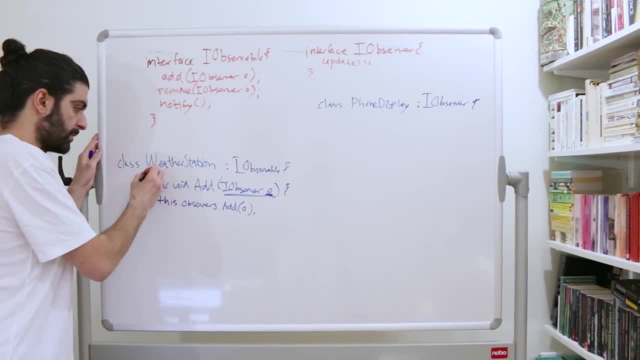 that are observing this particular observable. So of course that means that we also need to have the list here. So again, for the sake of space, I'll skip that, but here you would have to define that we have a list of observers. 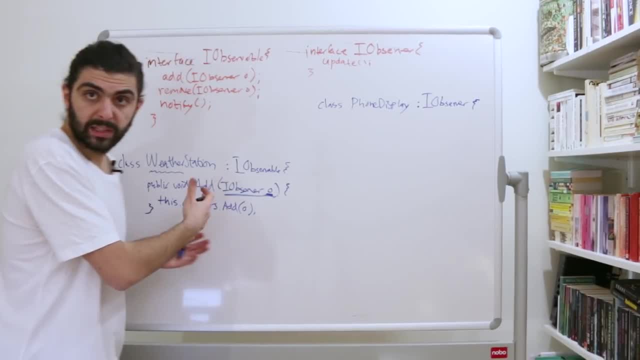 I think you can figure that out And that's the implementation of add And then remove is essentially the inverse of this. So I won't do remove right, But remove essentially just say okay, thisobserversremove this particular observer that I was passed in. 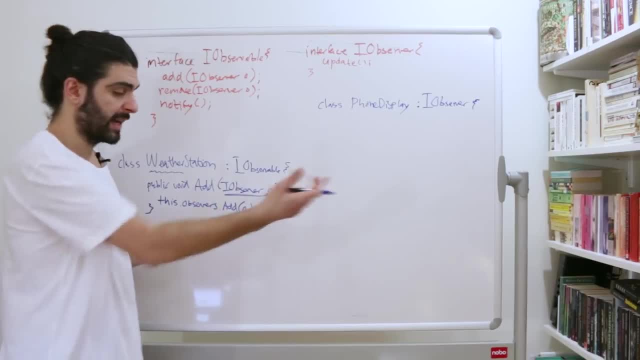 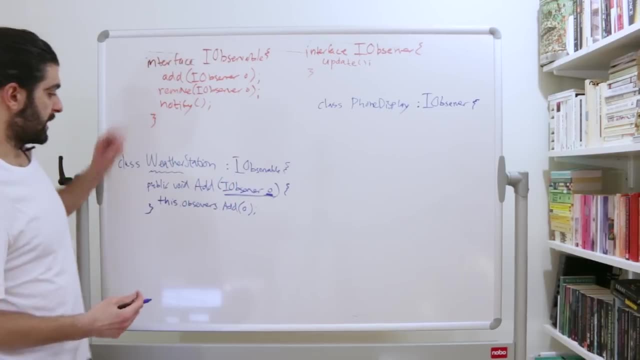 So it's collection. The weather station is collection of observers. You can pass in observers that you add to the list and then you can call remove to remove observers from the list, or rather, more generally, the collection. But, more interestingly, we have the notify method. 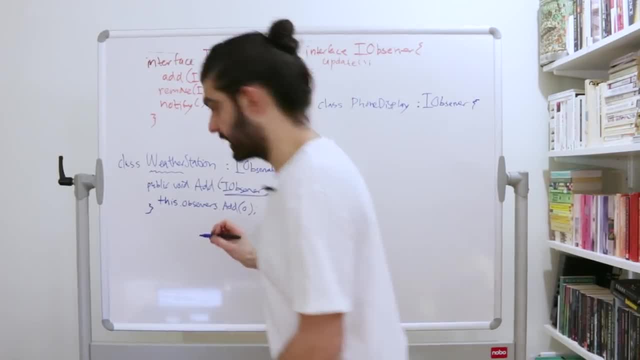 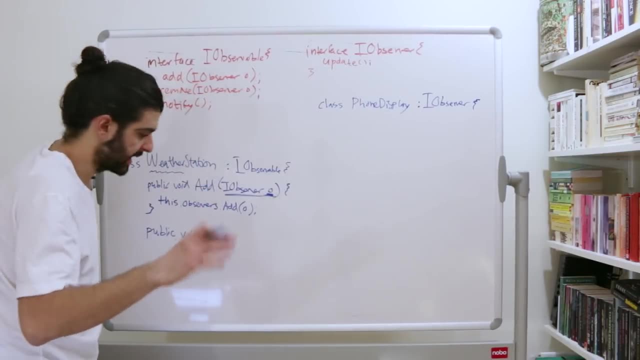 And the notify method is really simple. What we do is essentially, let's just say public void, notify. So sorry, here I used lowercase and here I used uppercase, but you'll figure it out, Apologies. Notify takes no arguments. 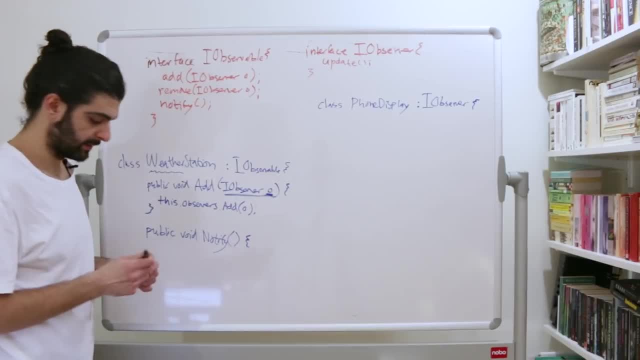 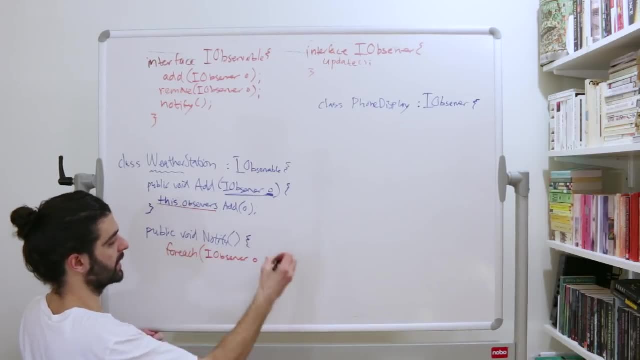 And what's the implementation of notify? The implementation of notify is that we say for each iObserver, let's call it o in my list of observers, in thisobservers, for each of these observers do what o the observer update? 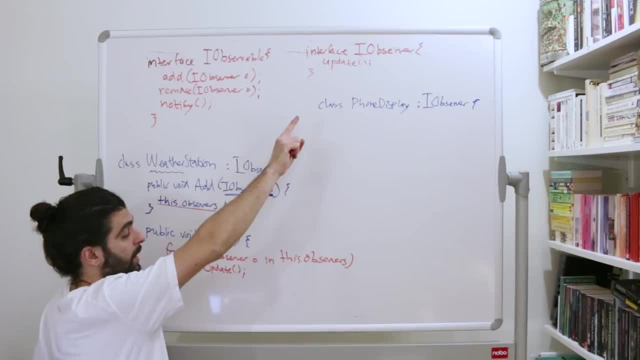 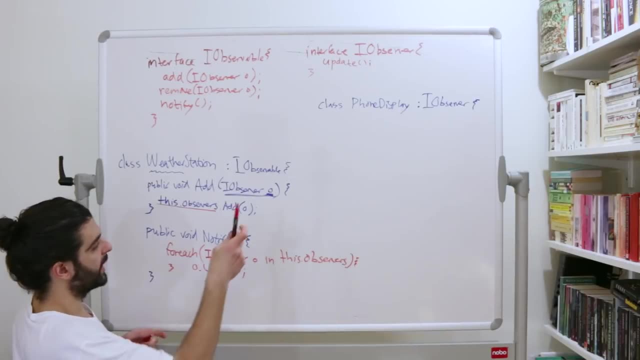 Because each observer has a method called update And that's how we notify When you call notify. let me close this curly brace. When you call notify on the weather station, you iterate over all of the observers in the collection: thisobservers. 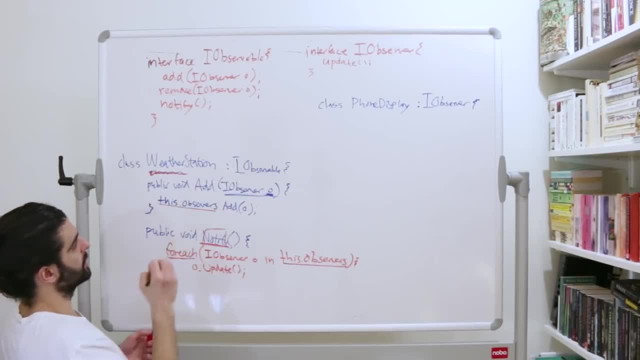 in the collection observers that we defined here in the weather station. So the weather station has a collection of observers. You iterate over the collection of observers and then you call update on each of those observers, And this is the heart of the observer pattern. 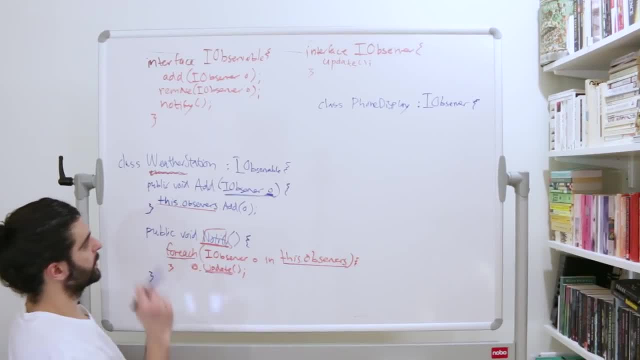 If you get that, you get the observer pattern, And of course, we talked before about how the weather station needs to have some method that it makes it possible to access the data that's in there. So we also need to have, let's say, that the temperature is returned as an integer. 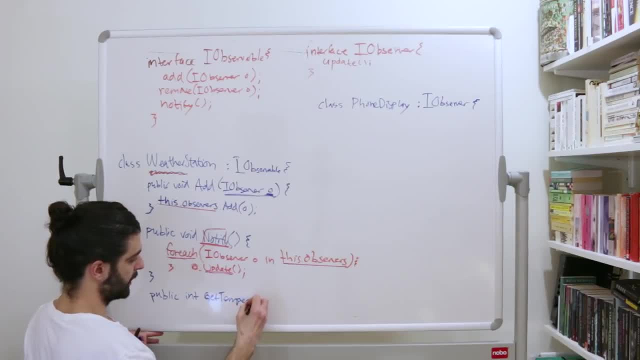 So we have a method, public int getTemperature- and we haven't built that We would need to define an instance variable here that holds the temperature or something like that. So let's assume that we have that, or let's pretend that we have that. 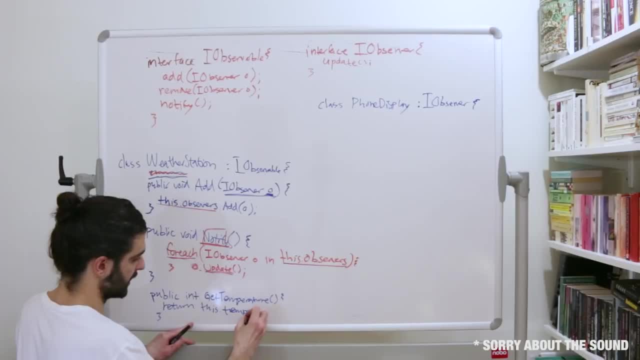 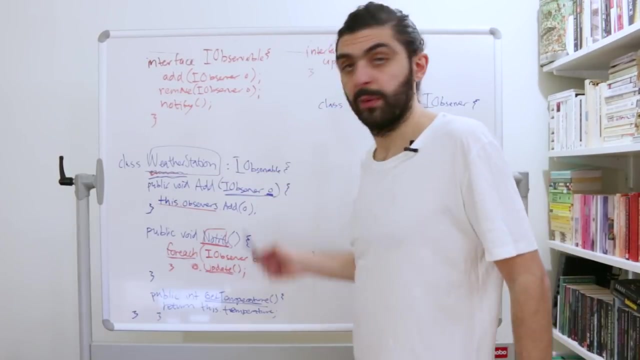 Then I would say something like return Thistemperature, right? So when you call getTemperature, you get an int back which corresponds to the temperature of the weather station at that particular time. Let's close this curly braces. So that's essentially the implementation. 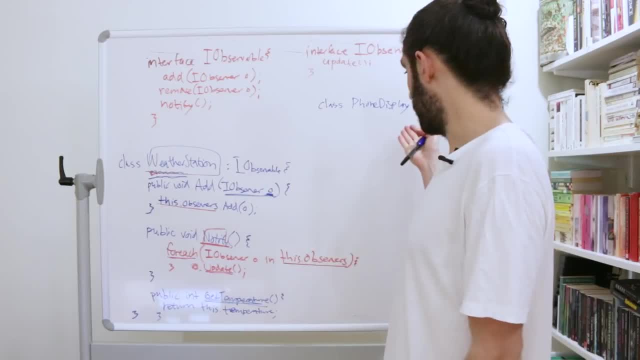 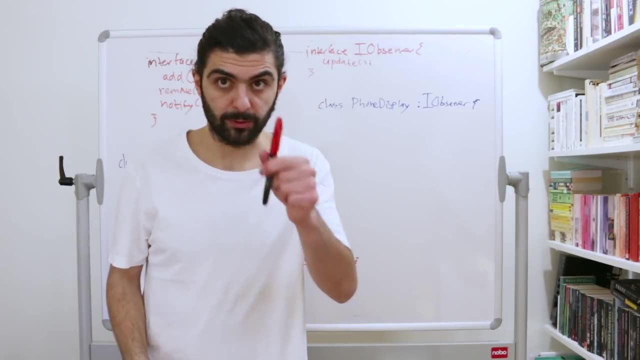 of the weather station. And then what's the implementation of the displays? Well, the displays essentially need to have the update method, but the crux is: remember that we've talked before about that constructor, So now we need to actually build that constructor. 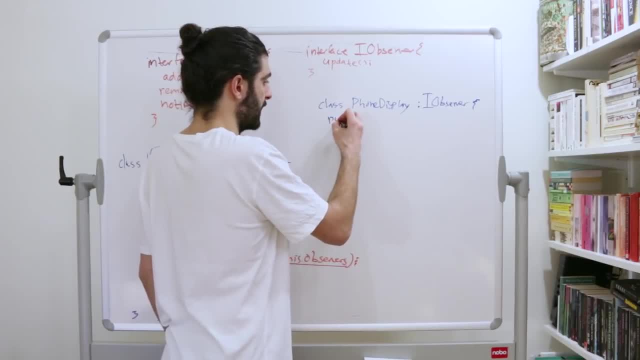 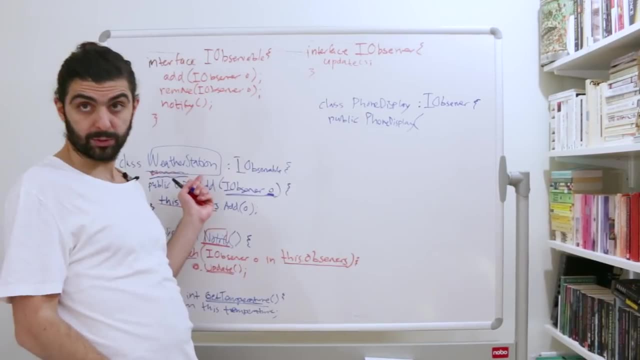 So let's build a constructor of the phone display, So let's say public phone display. and here's the key. it takes an argument, And that argument is of what type? It is of type weather station. So it takes a concrete weather station. 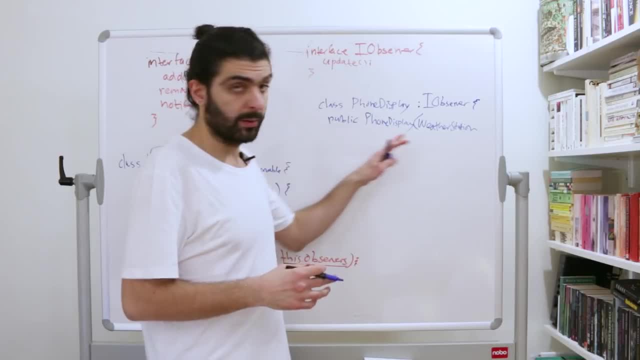 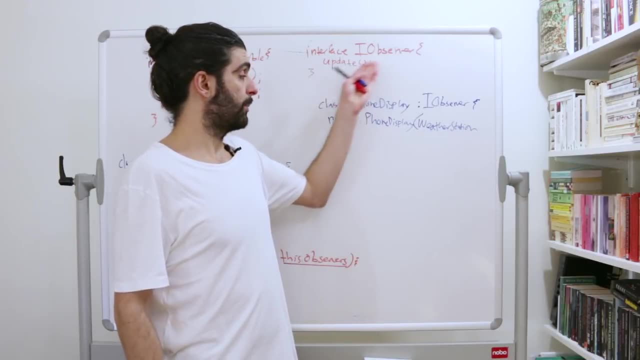 And again I mean: don't freak out about coupling to concretions. There's probably a better way to do this. Yes, let's dig into that some other time, But coupling to the concretion weather station here is less bad than if we would have coupled. 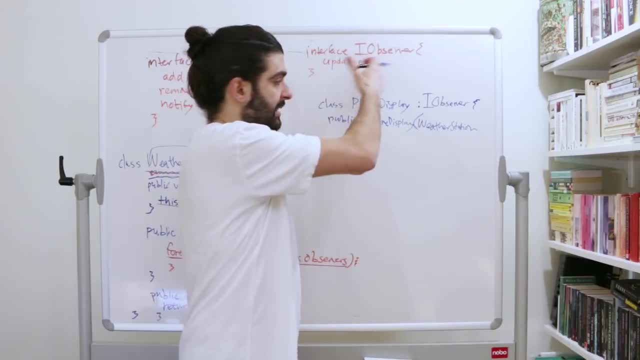 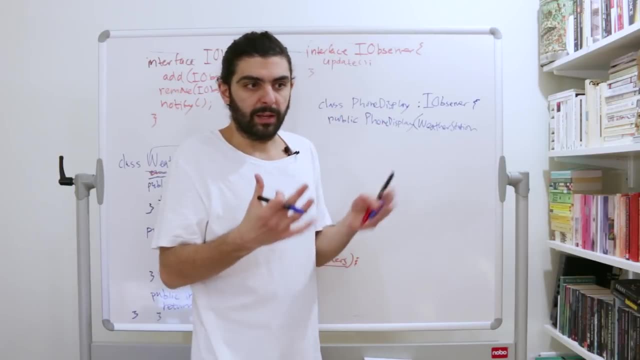 to the concretion weather station here, Because at least then you have an abstract ancestor up here that isn't coupled to the concept of weather station, But when we have a concrete phone display, that's suddenly a phone display for weather stations. So it's not really. 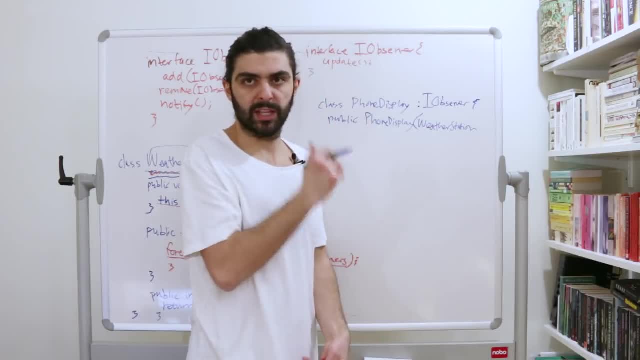 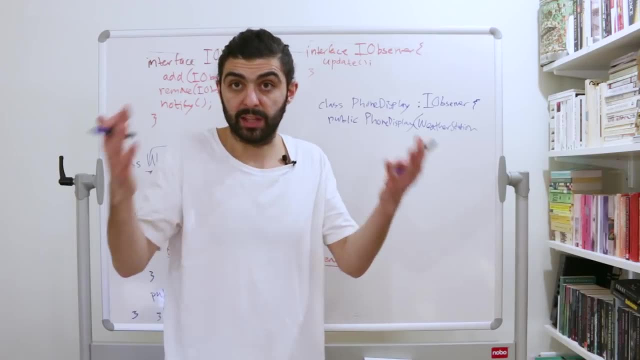 to me it doesn't really feel that bad that we're coupling to a concrete weather station, right, Because you can think of it in terms of the semantics. right, You can think about how a phone display isn't a display that displays anything, right? 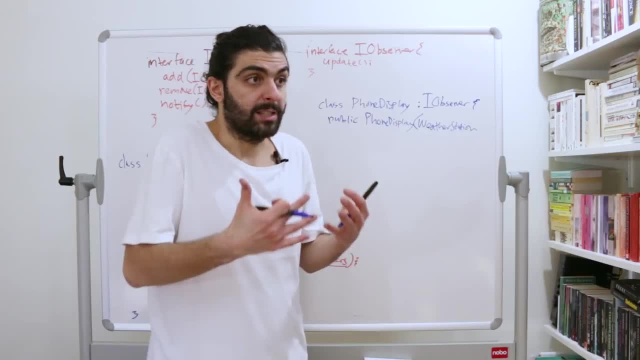 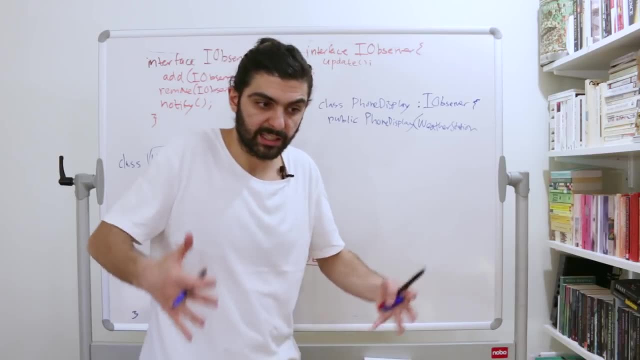 In this particular scenario, we're modeling a display that displays weather station data and thus it can couple to the concretion weather station. If we want to model a display that can display anything, we need to increase abstraction and get rid of the weather station. 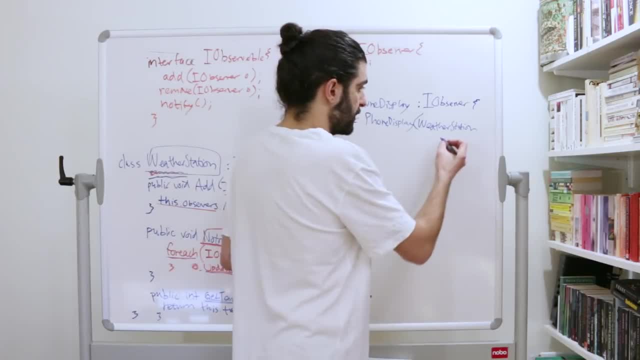 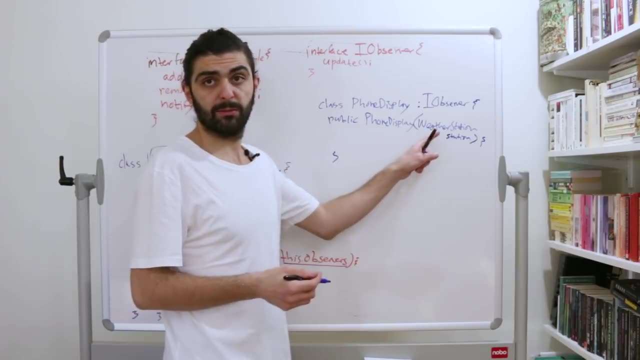 But that's not relevant for this example. so let's move on. So we pass in the weather station, let me call the variable name station and I'll open the constructor. And what's the implementation of the constructor? Essentially, we'll just save this parameter. 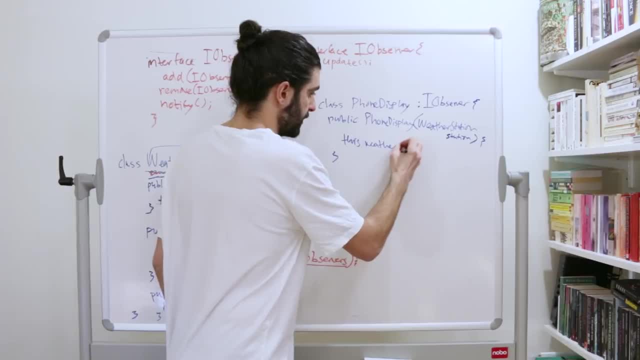 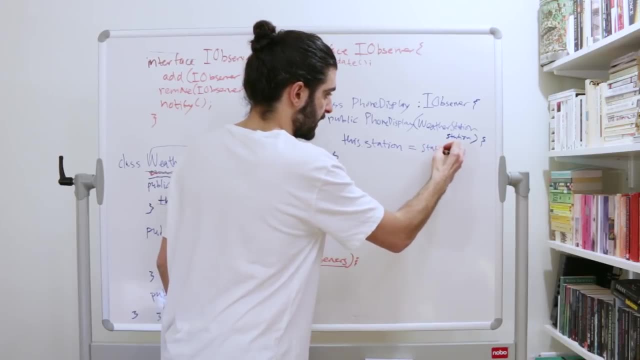 that we were passed in. So we say thisweatherStation actually let me to save space. let's say thisstation is equal to the station that we passed in, And it's important to realize that what we're doing is that we're setting the variable. 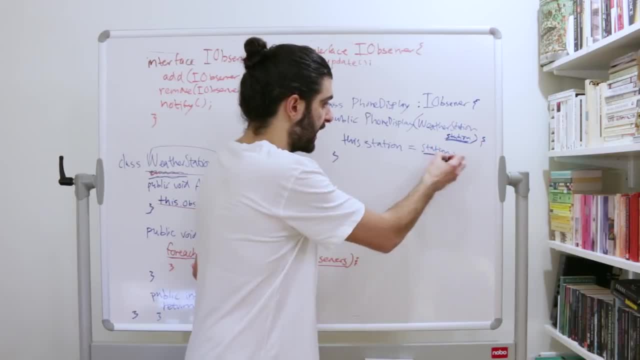 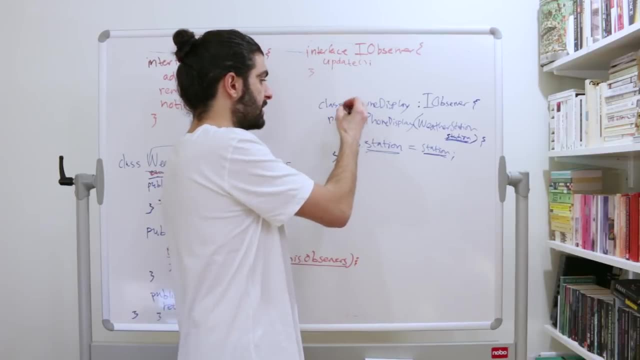 the value that we passed in through the constructor, that's this value. we're taking that value and setting it to a variable that we have in the scope of this class, in the scope of this instance. So we have an instance variable here, called of type weather station. 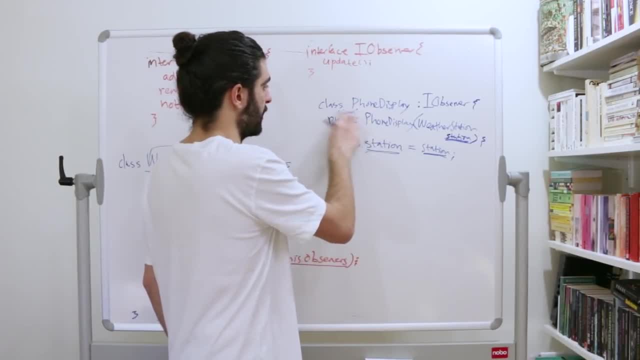 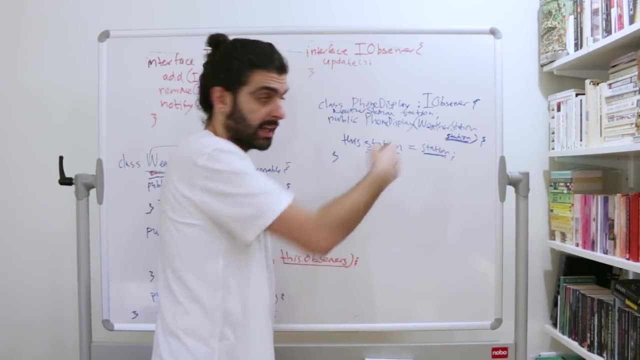 Man, this is totally messy. I apologize for that. We have an instance variable here called weather station, So it's that variable that we're setting when we're passing this in here. If that doesn't make any sense to you, please be sure to check out my previous video. 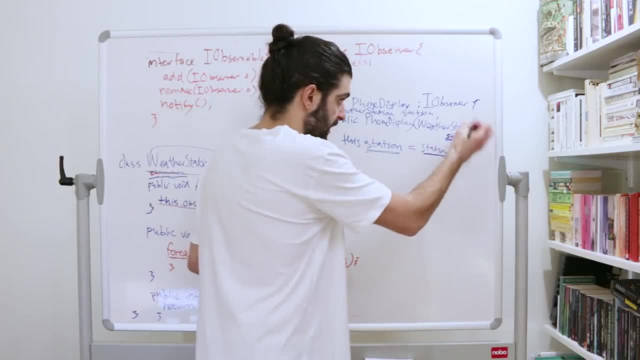 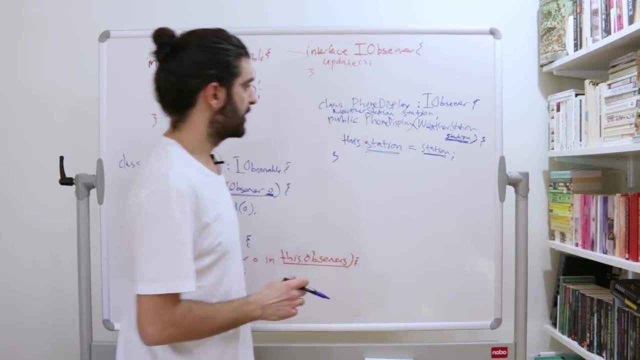 on strategy pattern where I make that more clear. But we're essentially passing something in dependency injection through the constructor and then setting that on the instance level. So, now that we have that station, what's next? Well, what's next is to implement the update method. 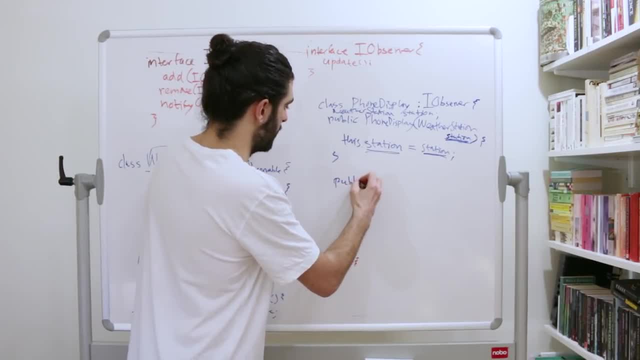 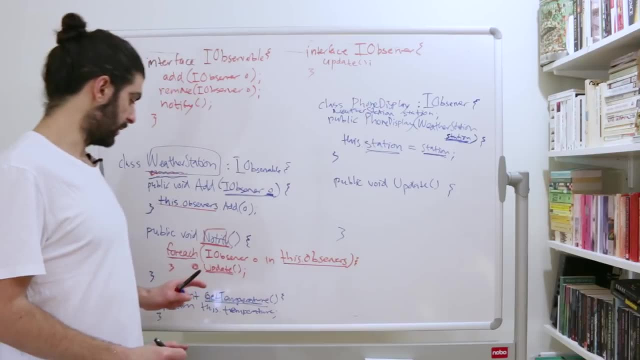 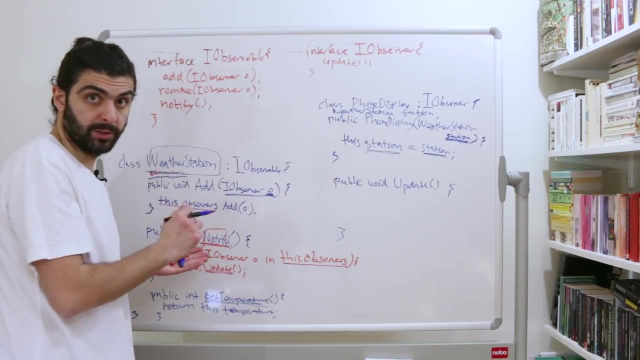 So let's implement the update method. So the update method says: okay, we have a public void, update takes no arguments. And what's the implementation? Think about when update is called. Update is called here. Update is called whenever the weather station wants to notify all of the observers. 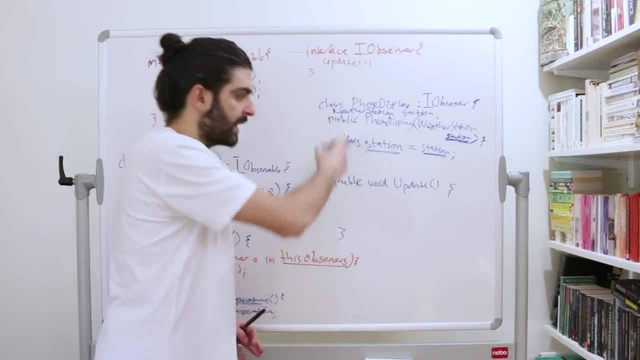 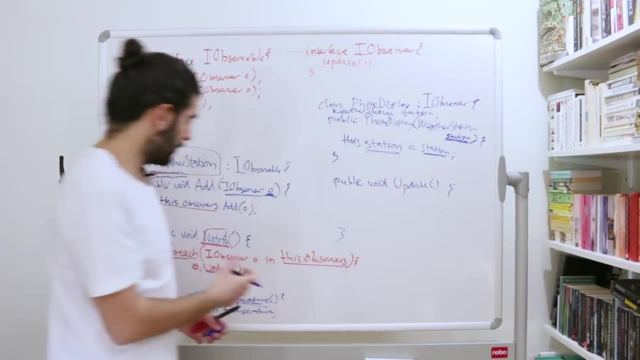 When somebody calls notify on the weather station, all of the displays, their update methods, are called. The update method of all of the displays is called. So this update method is called whenever there is an update. It's essentially called whenever something has happened. 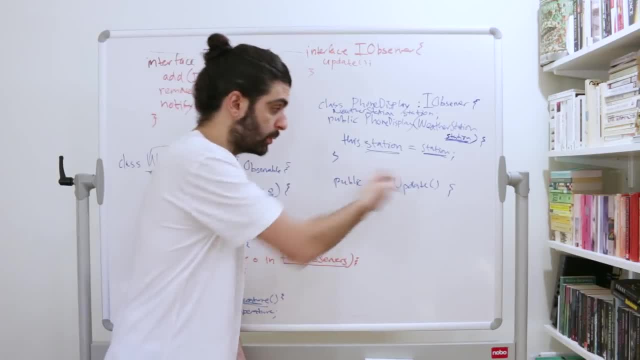 in the weather station that somebody has deemed important, important enough to update. And here's the thing that we talked about before: If we didn't pass in the station to the constructor, if we didn't do that, what would we do here? 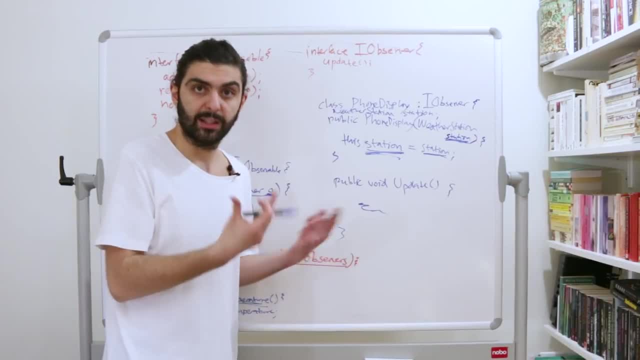 We would know. aha, okay, the weather station has some new data. I know that, But what am I going to do with that data? Because I can't access that data. So, because we passed in the station through the constructor. 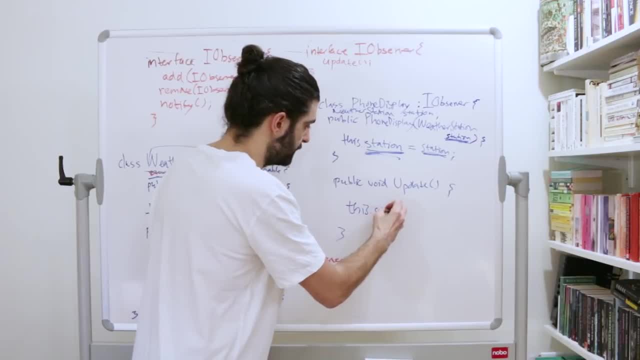 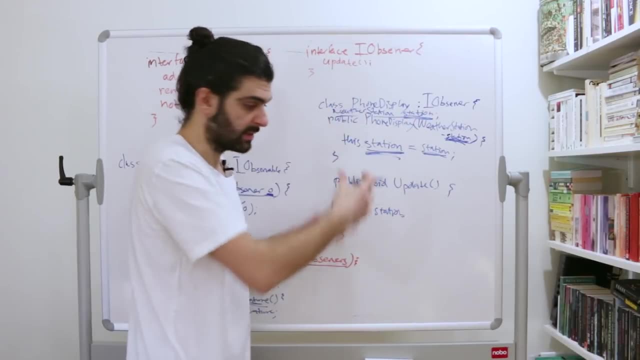 we can now actually access that and say, okay, this dot station, not this station that we passed in through the constructor, but the one that we saved on the instance level, the one that we saved into the instance, So we have access to that station. 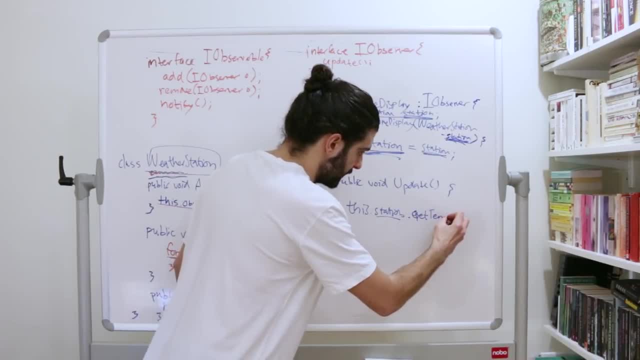 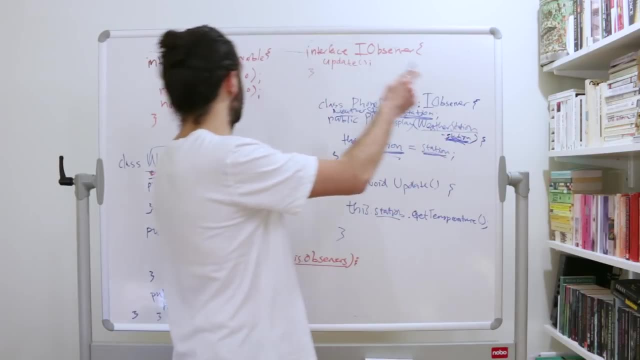 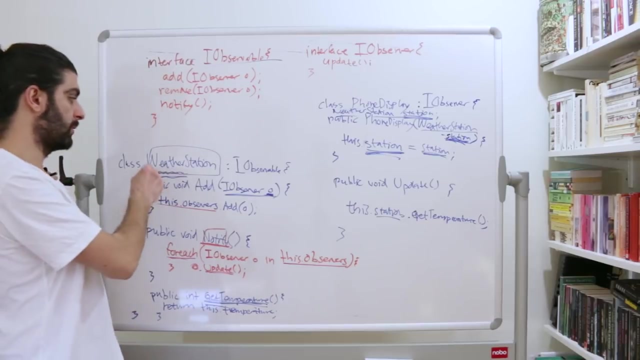 And then we can say this: dot station, dot, get temperature, Boom, Because we defined get temperature Here. So because we're accessing it as a weather station and not as an- I- observable, we can have access to the method get temperature because get temperature is defined on the weather station. 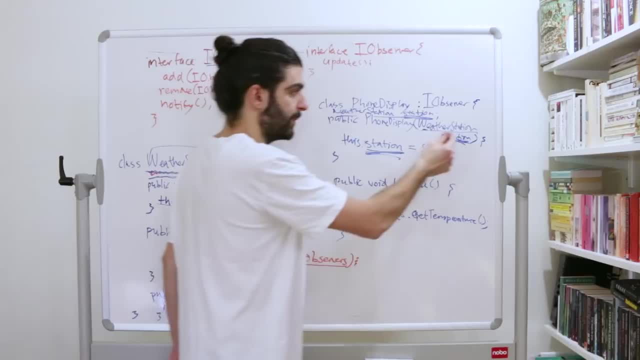 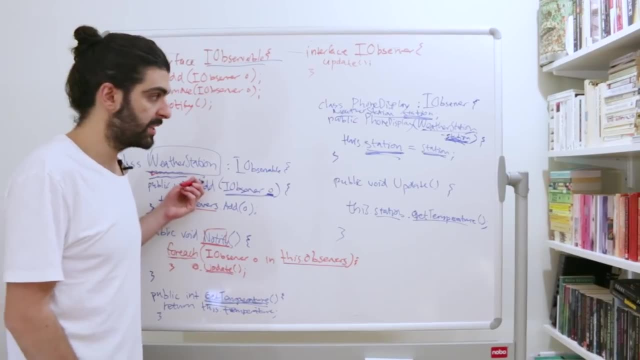 and not on all observables right. So here we're actually coupling to the concretion so that we can get access to the get temperature method. So you instantiate the weather station, you instantiate the display, And when you instantiate the display you pass it the instance of the weather station. 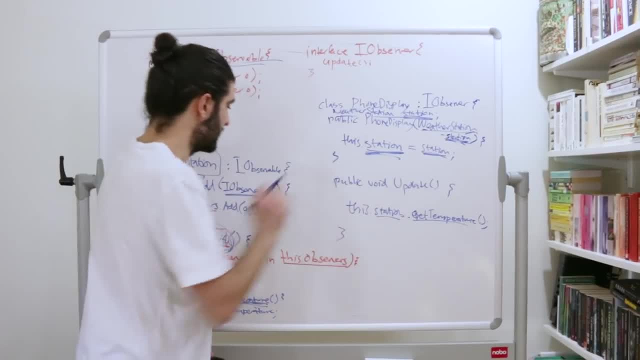 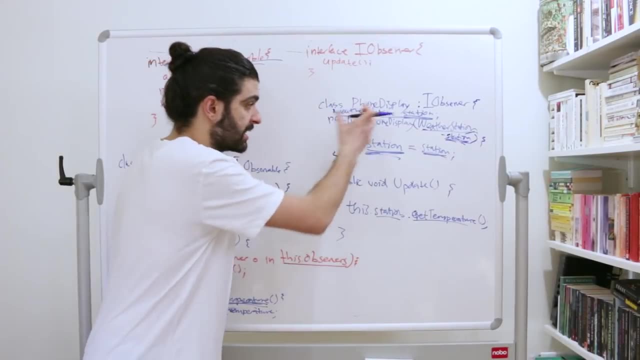 In here And then we take this display instance and we pass it in a call to add. So we call add on the weather station and pass it the instance of the display. When we do that, when we call add on the weather station and pass it an observer, 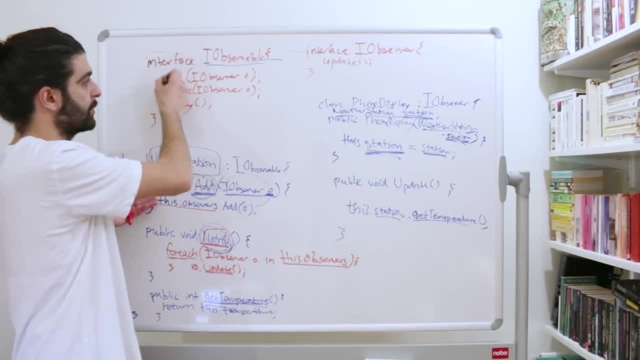 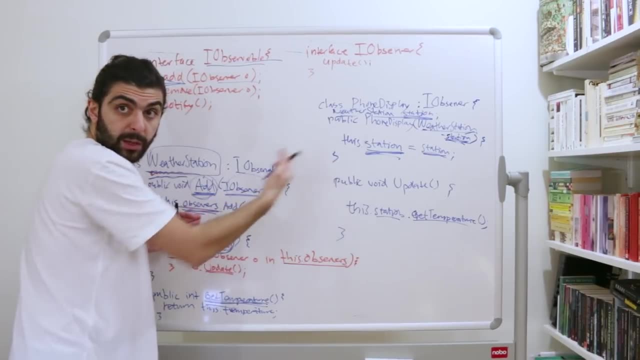 what the weather station does is that it implements the add method that the I observable asks it to implement, And the implementation is essentially that it has a list of observers and it takes the observer that it was passed in and it adds this observer to its list of observers. 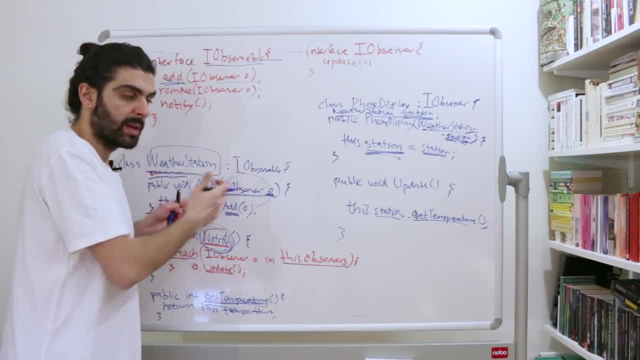 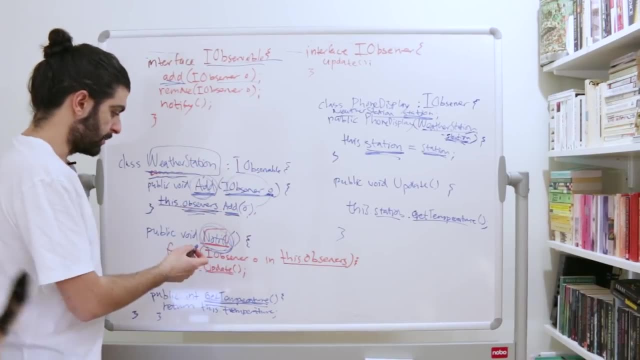 And semantically, why it does. that is that because it wants to be able to notify that observer whenever something changes. And then at some point later something changes. right, We haven't covered how or why something would change, but essentially we have the notify method. 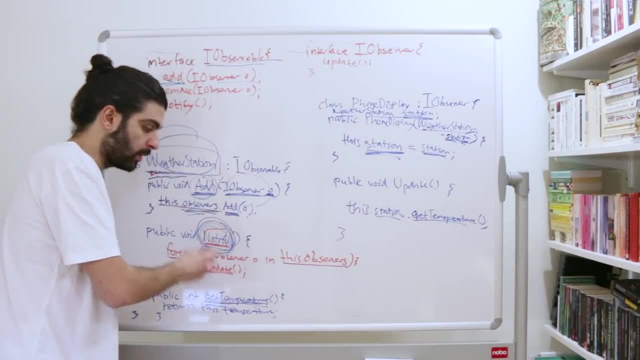 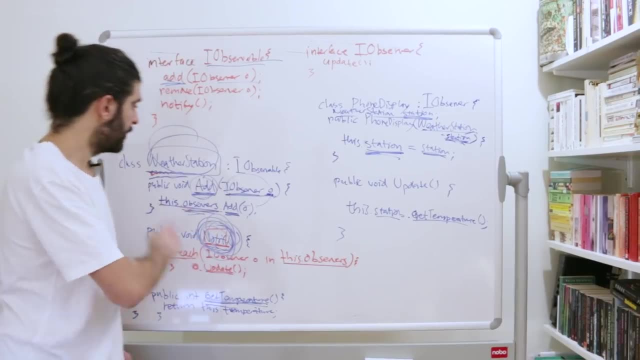 So, regardless of whether the weather station itself calls the notify method or whether somebody else calls the notify method, when the notify method is called, what the weather station does is that it foreaches, it loops through it, it iterates through its collection of observers. 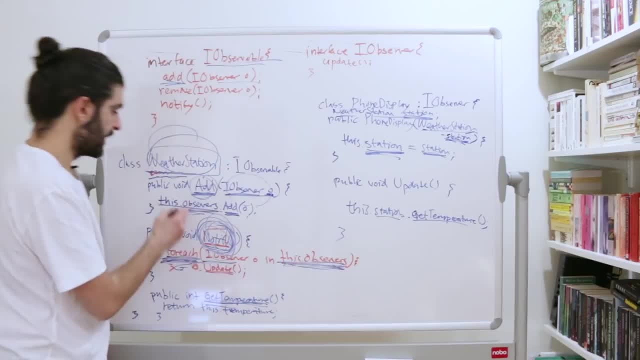 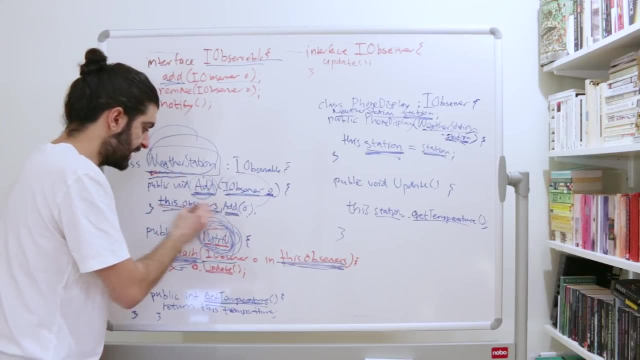 the observers that it has in thisobservers. and this collection is the one contains the observer that we passed in before, because we call the add method and we added in that observer. So we have this list of observers and we iterate through that list of observers. 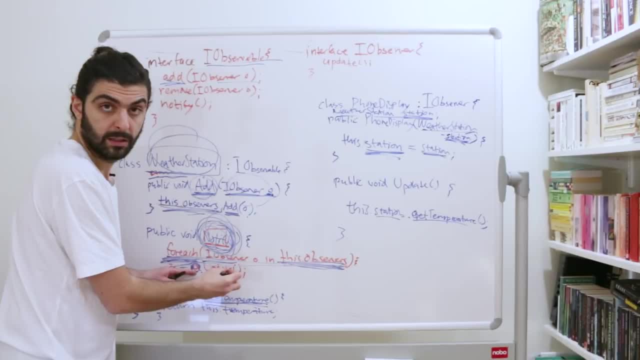 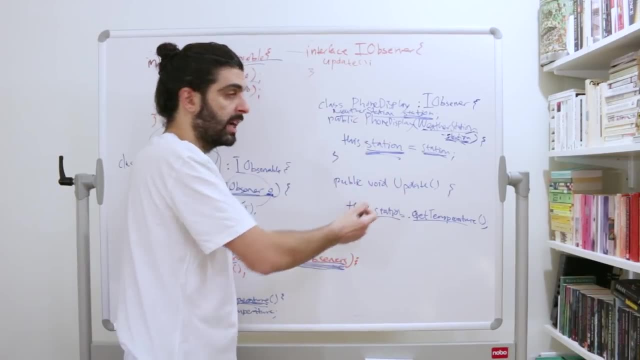 and for each of the observers we say update And when we call update on that observer, we're in here, we're in the phone display because that's an observer and we've added the observer to the weather station, to the observable. 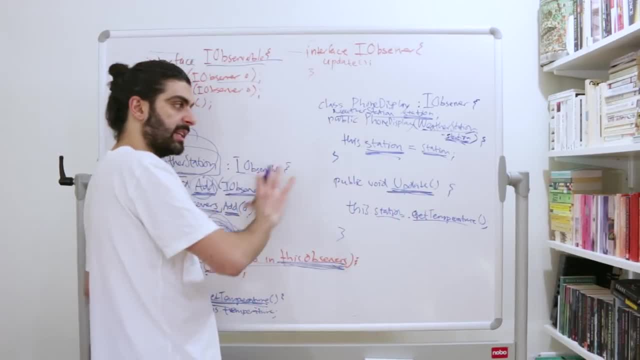 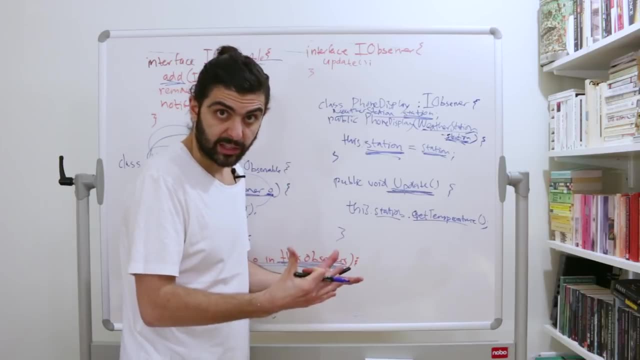 And when we then get a call to update- right, When they send the message, when the weather station sends the message- update here- then the phone display knows that, aha, something has changed and I can now update my display, or whatever this thing wants to do, right. 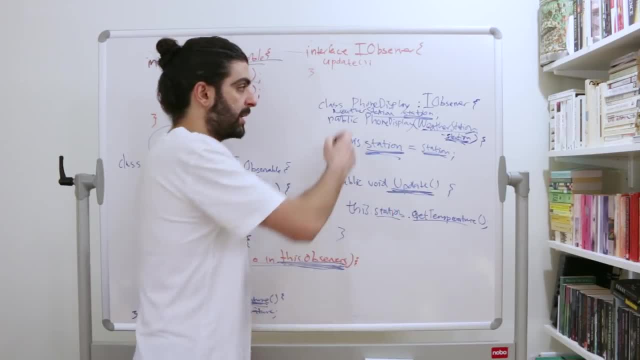 If it's a different scenario, if it's a subscriptions right, Maybe this is an article reader and we know when we call update, we know that there might have been a new article in the database of articles, so I need to update my list of articles that I have here. 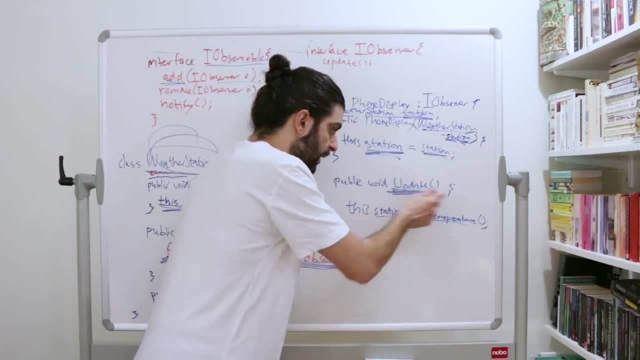 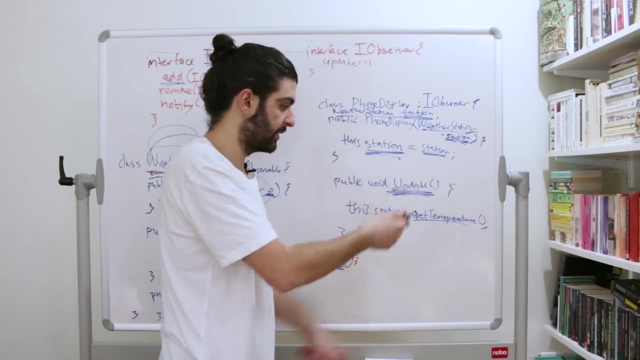 in the display or whatever this is, or the webpage or whatever. When I get that call to update, I know that something has happened and I need to react to this right, Because that's why I subscribed: because I wanted to be able to react to this. 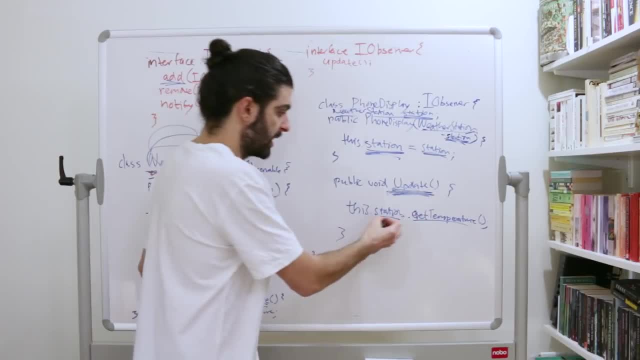 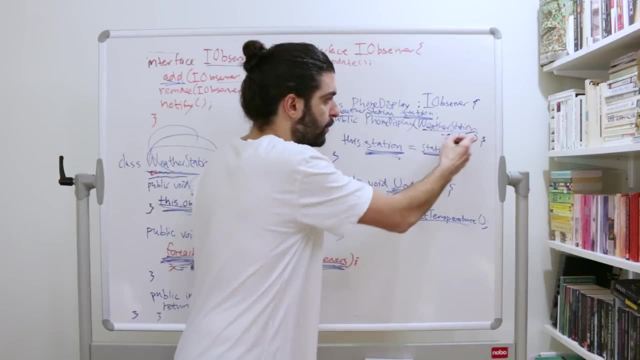 And how I get information from the weather station is through the reference that I have in this dot station, because when I created the display I passed in a weather station, a concrete weather station. I passed it in through the constructor and saved that as an instance variable. 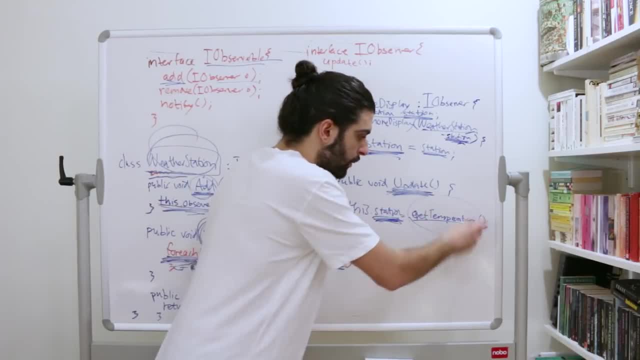 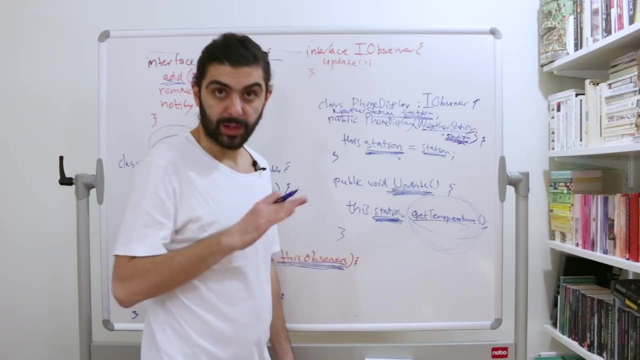 And now I can access that instance variable and call whatever methods I need, such as get temperature, in order to do whatever is relevant to do in this scenario Period. So I'm guessing either that was super overly clear or totally confusing. Please let me know which one. 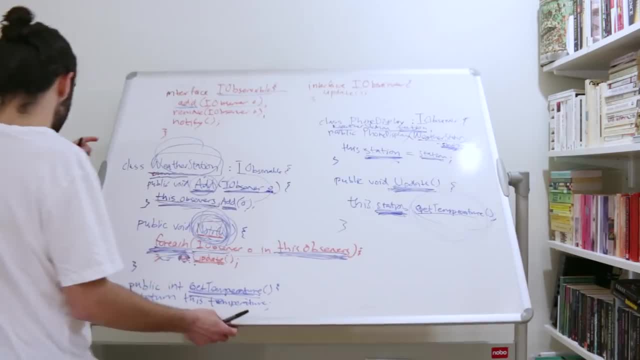 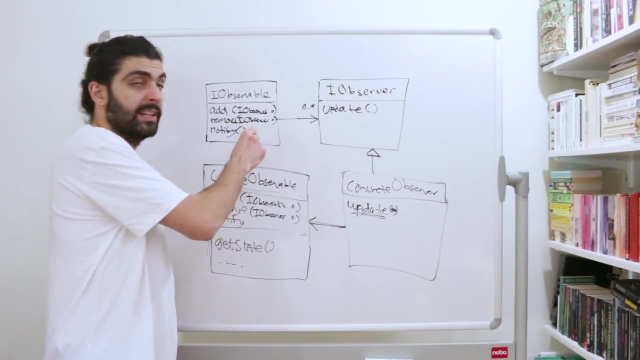 Before we wrap this up, let's get back to the UML diagram. So hopefully now this diagram makes a thousand percent sense. Let's look at it. We have an interface- IObservable- that has zero to many observers- IObservers, which is also an interface. 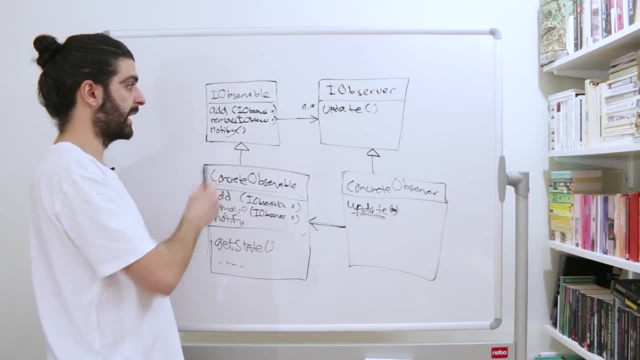 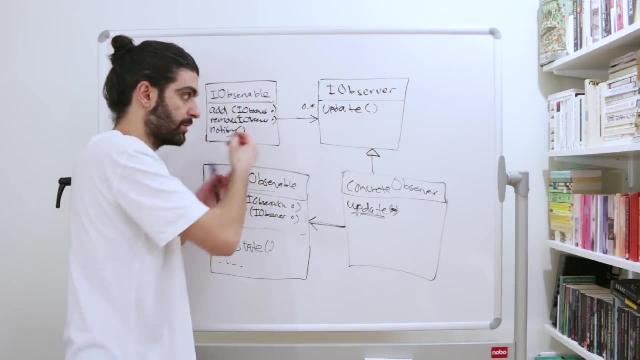 The interface IObservable has the methods add, remove and notify. Add: takes an IObserver so that it can save a reference to that observer, so that it can notify these observers whenever it undergoes some kind of change that the observer should be interested in. 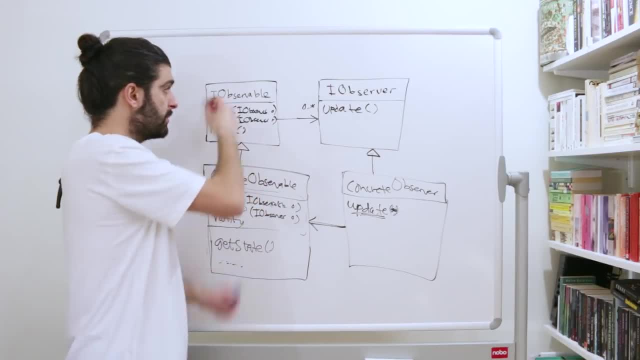 Remove does the inverse of that. It takes an observer and removes it from the list of observers that the observable has Notify, Essentially says, OK, I've got this list of observers. Let me now call update on all of these observers. Something has happened. 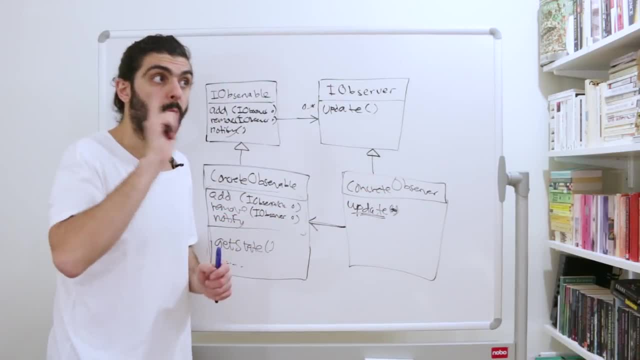 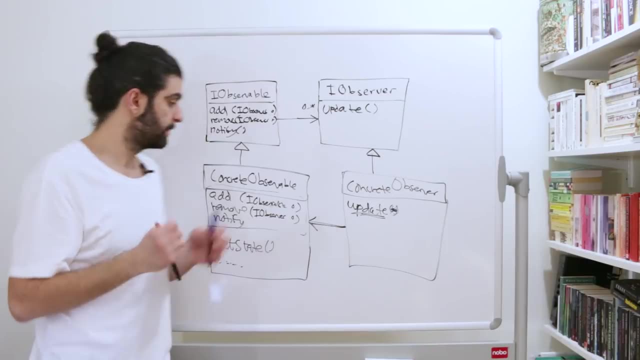 Let me notify all of the observers of the thing that has happened, Or of that something has happened, and that they should look into me to get the data that they're interested in because something has changed. And that's on the abstract level. On the concrete level, what do we have? 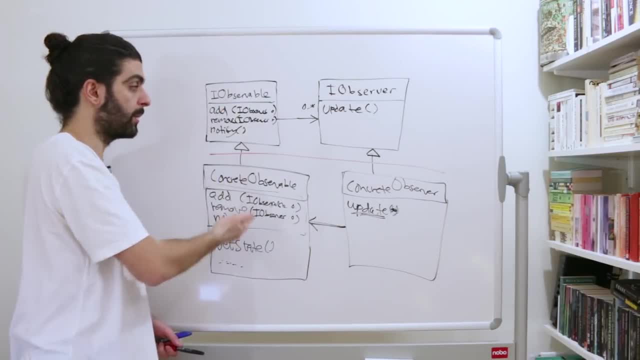 We have a concrete observable, And the concrete observable essentially just implements the methods that we talked about. right, This is actually just the contract. It says that to be an eye observable means that you need to specify these methods. You need to be callable in these terms. 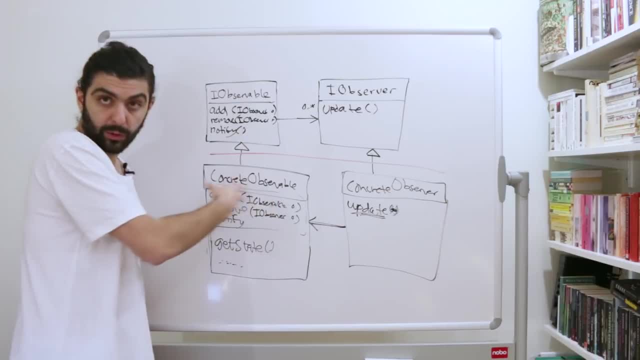 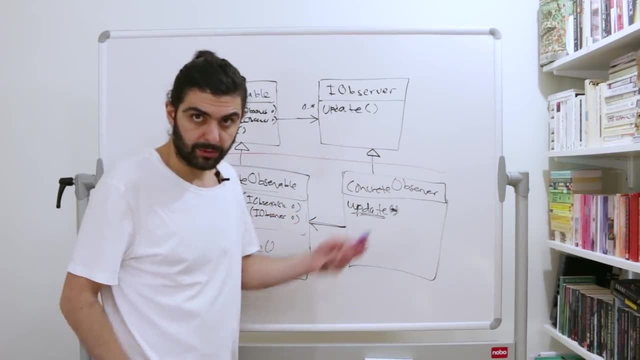 And the implementations that we talked about actually live here in the concrete observable. So this is where we actually implement addRu and notify, And same thing for concrete observer. If you have a concrete observer, then the update method depends on what your observer actually does. 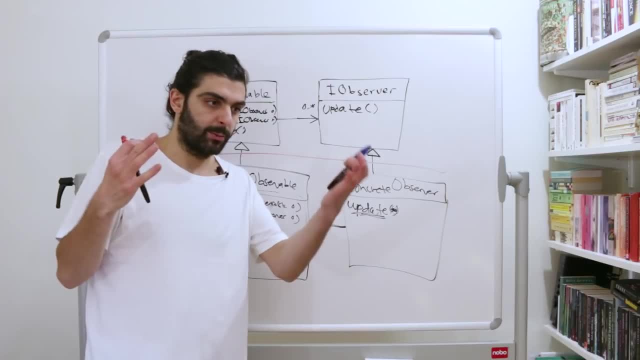 In terms of the displays, you have the LCD display or the window display and we have the phone display, And they might do completely different things, Or maybe you could think of it this way: Maybe you have a web display and a file display. 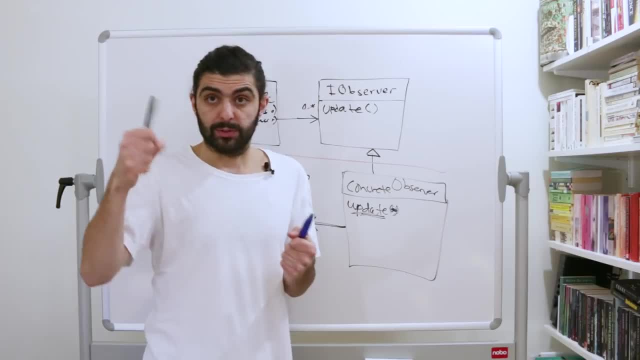 So one produces a file like a PDF file and one produces a web page, And the logic in these two methods will be completely different. A lot of overlap, but also completely different. So that's why the update method, the implementation of the update method, lives in the concrete observer. 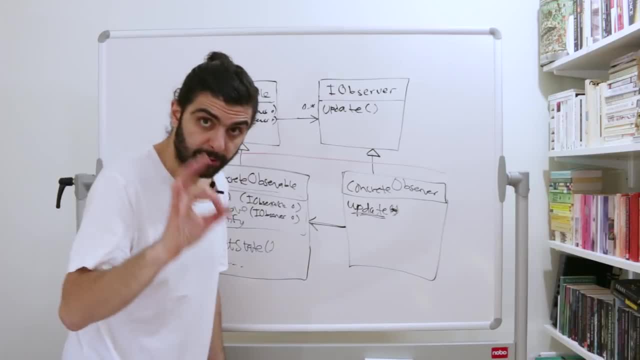 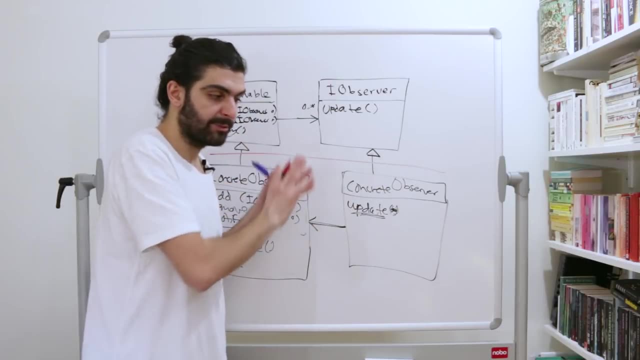 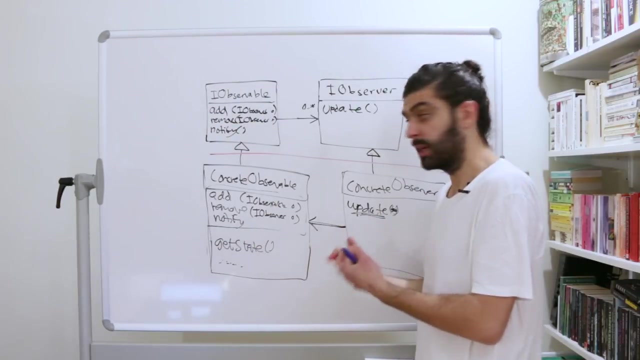 And then we have the method getState, because the particular flavor of observer pattern that we looked at here is one where you push the fact that you have a change, but the observers have to pull data. I should do this: pull in this direction. 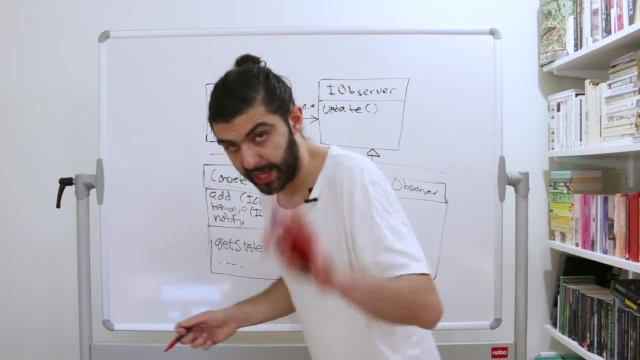 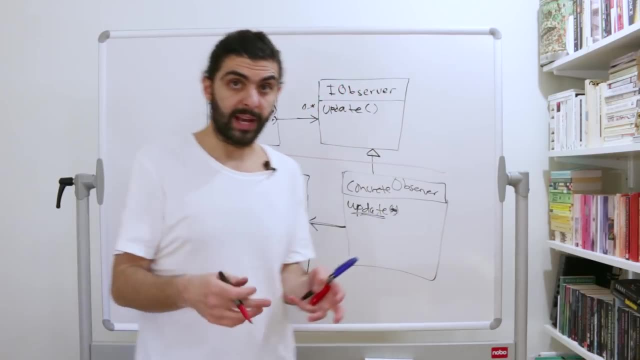 pull data from the concrete observable. There are variations of observer pattern. Let me know if you want us to discuss this and we'll dig into that in a different video. But there are variations of observer pattern where, instead of forcing the clients to have to pull data, 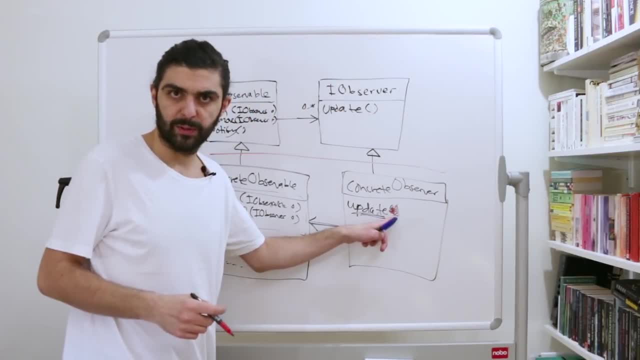 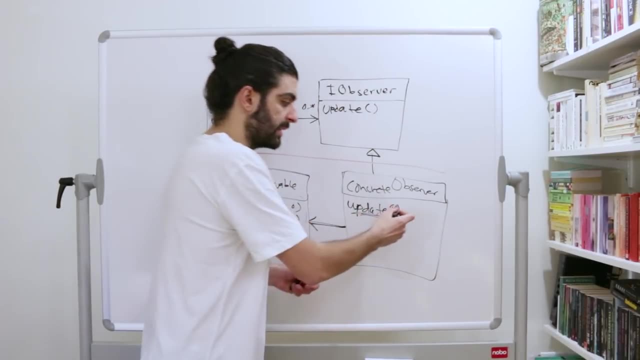 you push data through the update method- And we touched upon this before. Instead of just having an update method, you just have to pull data through the update method and then use the update method. that doesn't take any arguments. You send the message: update with some data. 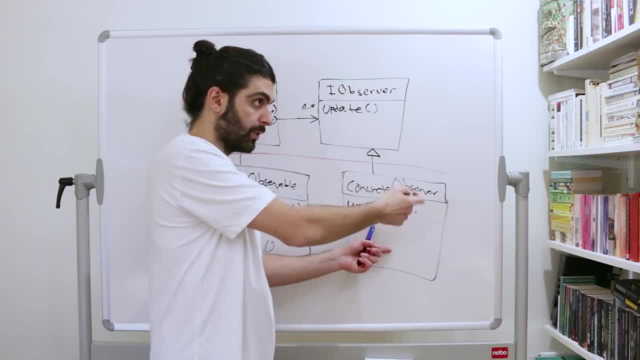 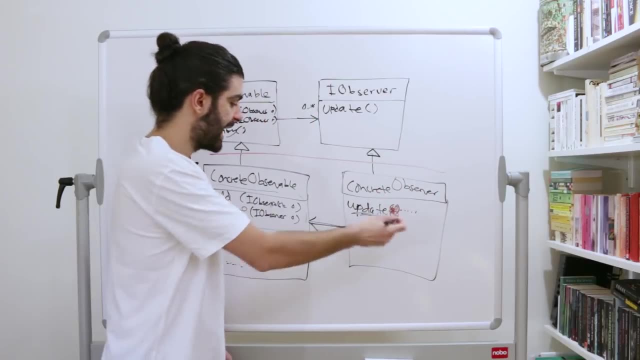 that the observer should be interested in. That means that the observer remember how we passed the observable through the constructor to the concrete observer. that means you don't have to do that. That means that the observer doesn't need to have a reference to the concrete observable which. 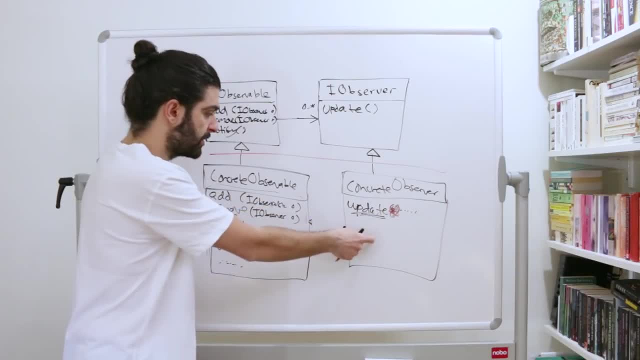 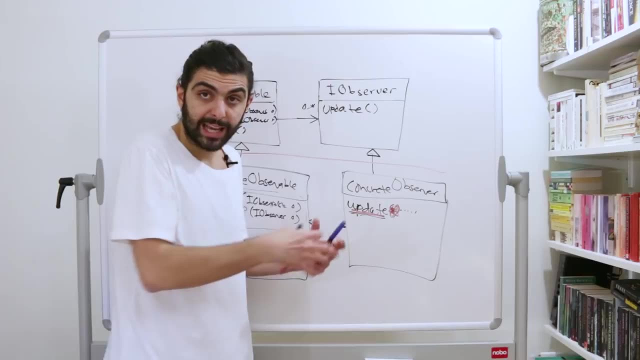 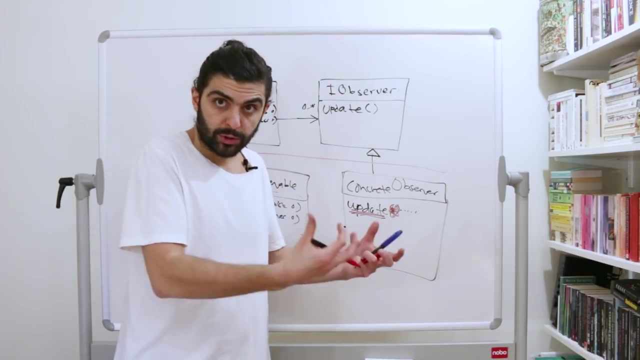 essentially, in terms of this UML diagram, the concrete observer does not need to have a concrete observable, because whenever you call update, the concrete observer gets not only notified but also gets the data that it should, that it should be concerned about. so then you're, it's kind of a push, push, you're, you're pushing. 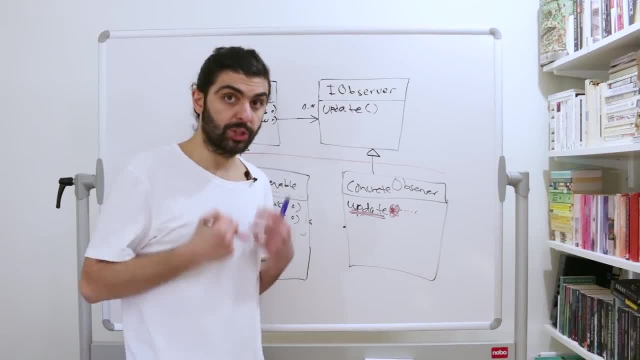 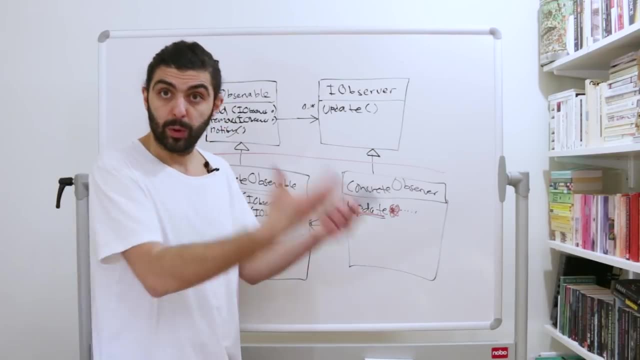 the fact that there has been a change, but you're also pushing the data that the observer should be interested in. what we've looked at here, when we still have this arrow, is more like a push pull. so you push the fact that there has been a change, but then the observer has to pull data from the 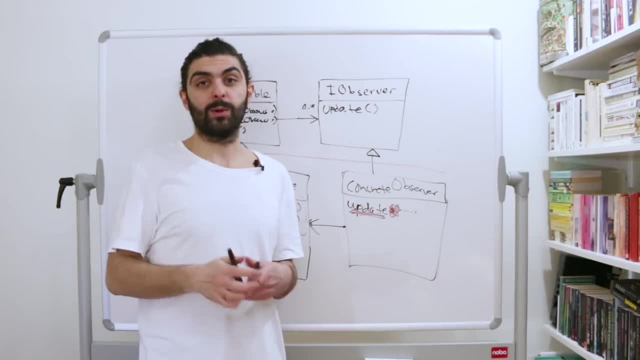 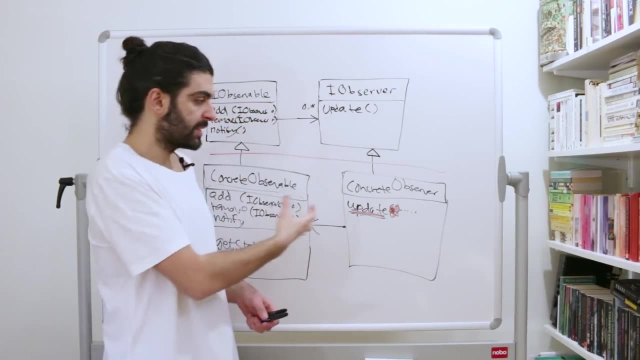 observable. but if we rewind all the way back to the beginning, where we started with the discussion about push versus poll, notice how i'm saying poll and not pull. so what we're saying here is that data has to be pulled, but it's still better than than having to pull for changes. the implementation: 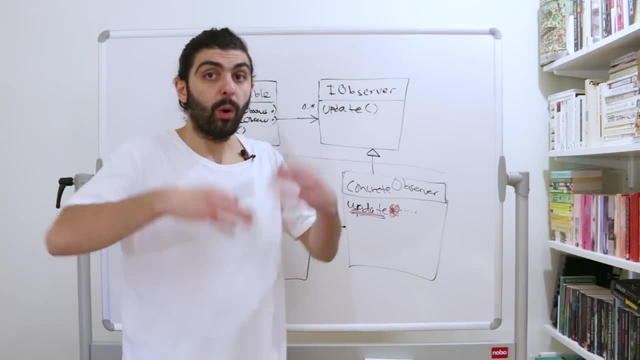 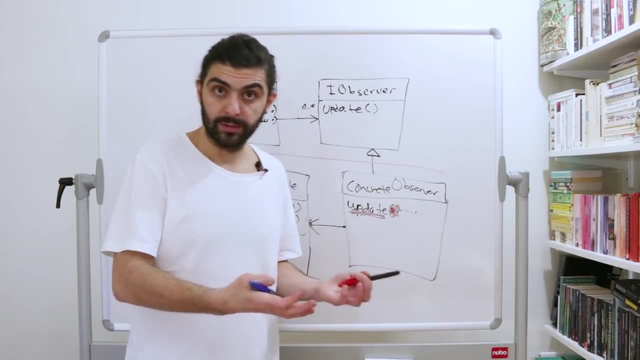 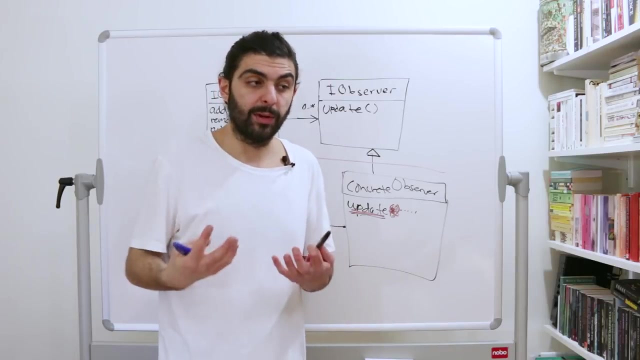 that we have here is kind of push pull, but when we talk about a poll implementation, we talk about polling for changes. we're talking about a, a pool pool or a pool push polling essentially means that the first step, the the idea of knowing whether there has been changes, that that step is carried out via pool right, is carried out. 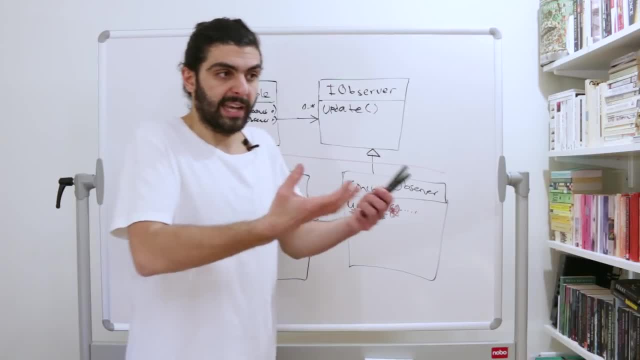 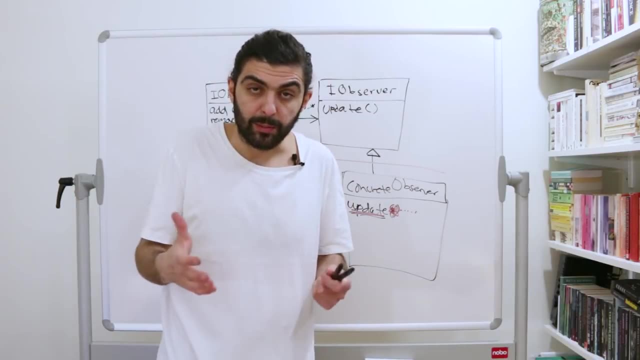 by the observer asking the observable whether it has changed. but if you're always asking whether it has changed, you can't know certainly when it has. but in in that kind of implementation you have to continuously keep asking in order to be notified at the correct time, because you never know. 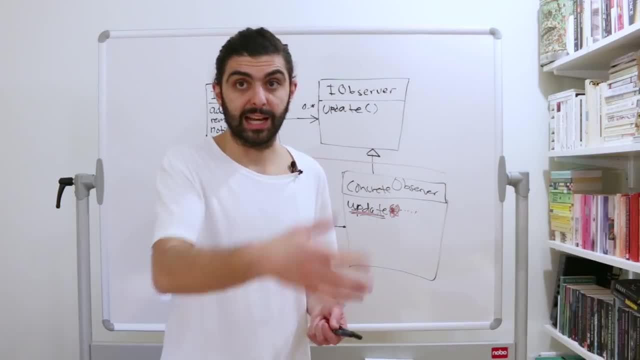 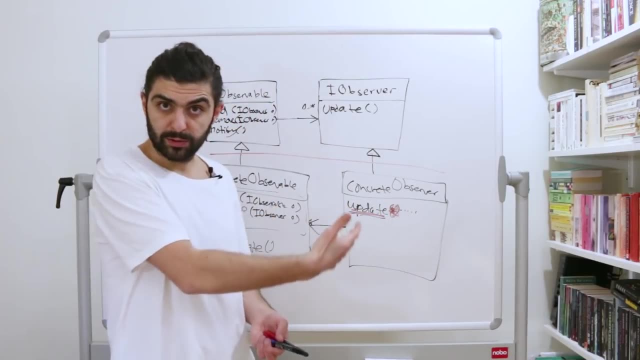 whether it has changed or not. so you just have to keep on asking, and asking and asking, and sometimes it has changed and sometimes it hasn't. but when you do a push push solution or a push pull solution that we looked at here, then you don't have to keep on pulling because you register your interest. 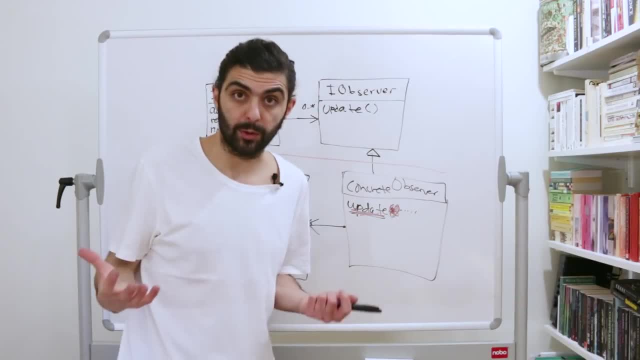 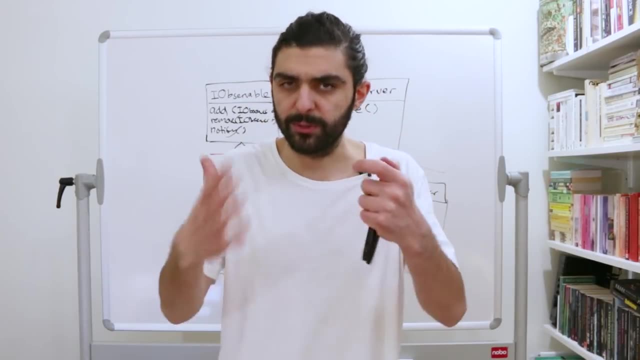 the observers register the fact that they want to be notified and then they're notified. so now i'm really smashing this in too much and i'm sort of iterating. so let me know if that was helpful or if you're looking for different kinds of information. if if you want to know more about the 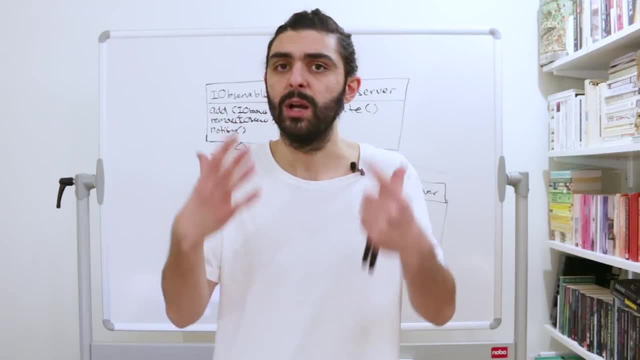 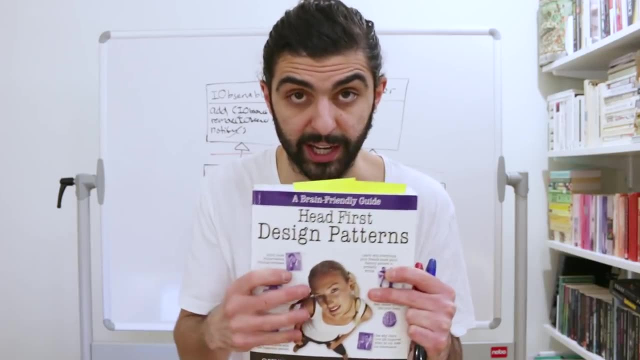 theory, or if you want me to sort of twist these things in different ways, i'd love to listen to you. your opinion matters greatly to me, so so shoot that in the comments. the link to this book is in the description. be sure to check it out. we've got tons of patterns to go, so remember to subscribe. 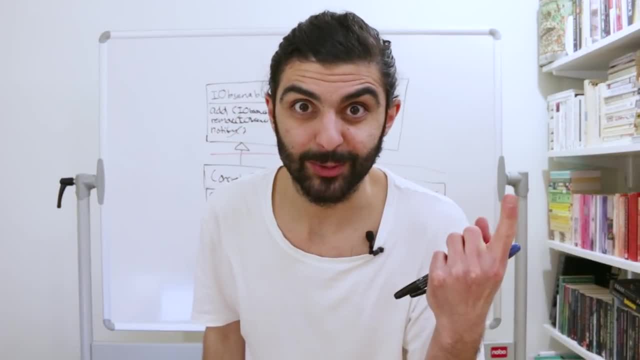 if you're not already subscribed. thanks for watching and i'll see you in the next one.